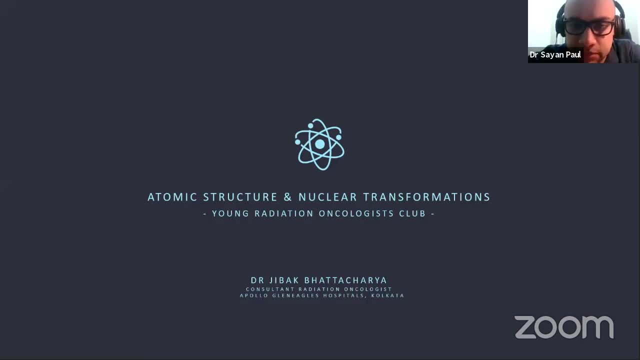 Faizan M Khan's medical physics book, from first chapter to last chapter. So those who want to ask any question can write it or type it in Q&A section. Don't type it in chat section. Type it in Q&A section And we have already reached our limit. Almost 500 people have joined, So I think we can. 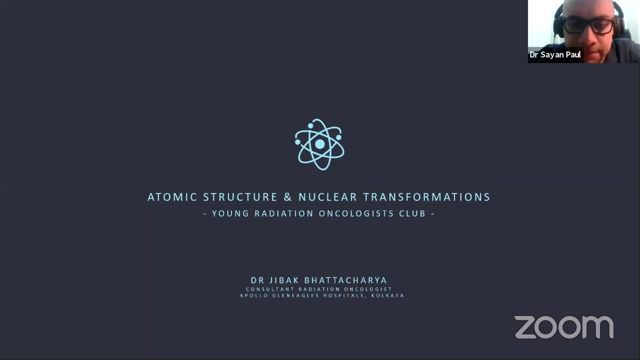 start the course And I welcome our first speaker We'll be talking today on atomic structure and nuclear transformation: Dr Jeevak Bhattacharya. Dr Jeevak Bhattacharya is a young, dynamic radiation oncologist. He is a consultant. 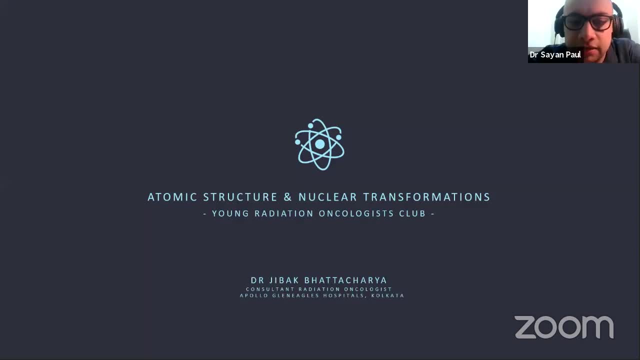 In Apollo Clinical Hospital, Kolkata, And he will be taking the first class And I hope everybody will enjoy the class and everybody will be benefited. So let us welcome Dr Jeevak Bhattacharya, And now I hand over this mic to Dr Jeevak Bhattacharya. Dr Jeevak Bhattacharya, please. 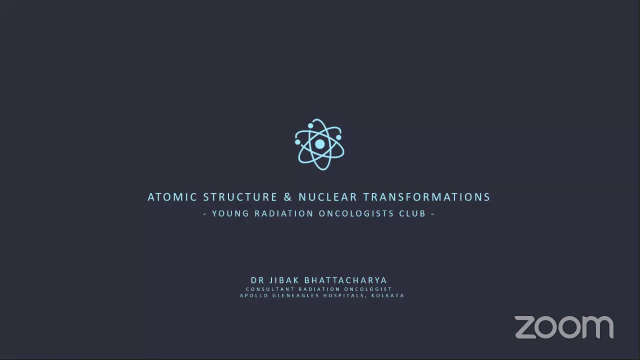 Thank you. Thank you, sir. So good evening everybody. First I would like to thank the panel for giving me the opportunity to present today, And particularly this topic of atomic structure and nuclear transformation is very close to my heart, And so I have tried to make it as. 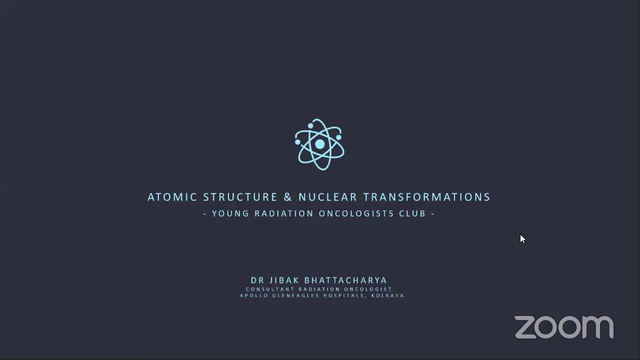 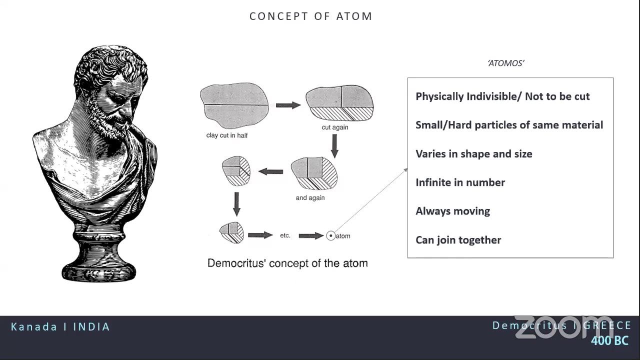 interesting as possible. So let's start the atomic structure. So if you trace through the history, you will find that the concept of atom was generated in almost 400 before the year, 400 before Christ. At the same time, in the Greece by Democritus, and in India has found the concept of atom as the 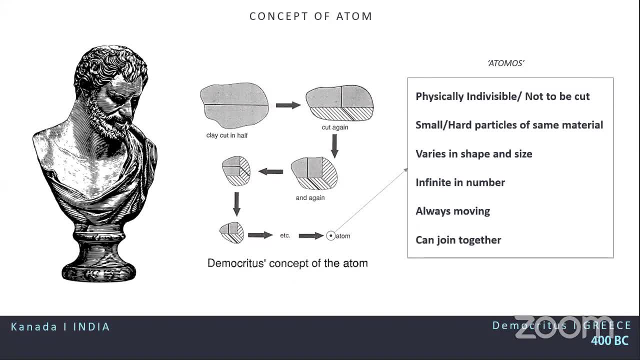 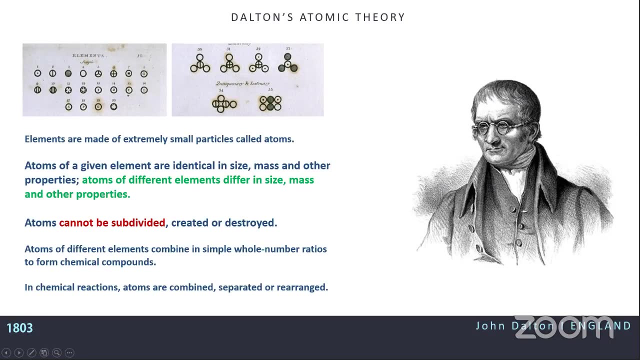 indestructible element of the nature, that if you start cutting something one by one and again and again and you'll find something when you cannot cut it further. So they named it atom. So for next 2000 years nobody actually was interested to know about atom, And then at around 1800,. 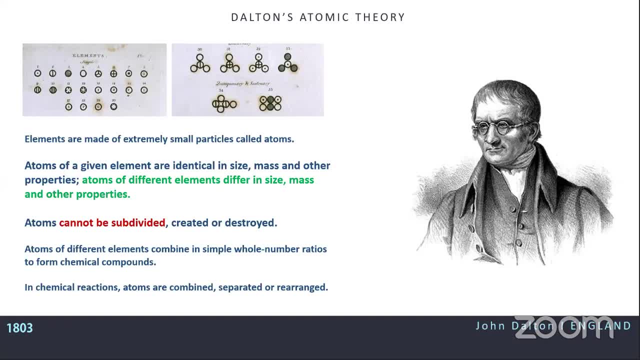 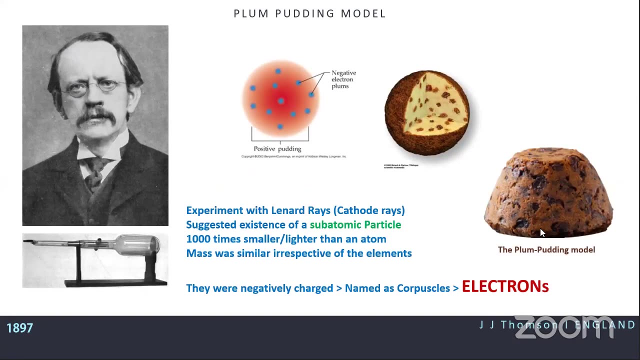 John Dalton first published the atomic theory, who said that the who just identified that the atoms are solid particles of elements which are different elements, and for different elements, the differing size, mass and other properties. He did not go to any further detail. The most interesting part started as early as 1897, when the British scientist JJ Thomson 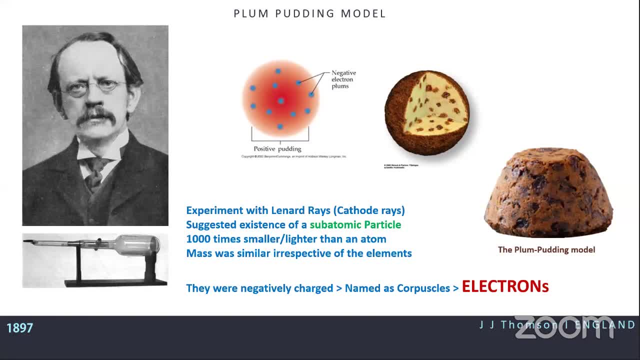 was experimenting with this cathode ray At that time. the cathode ray was named as Leonard ray's, So what he found was that there are some subatomic particle coming out of the elements which are very lighter or smaller than the atom actually, and which is almost 1000 times smaller. 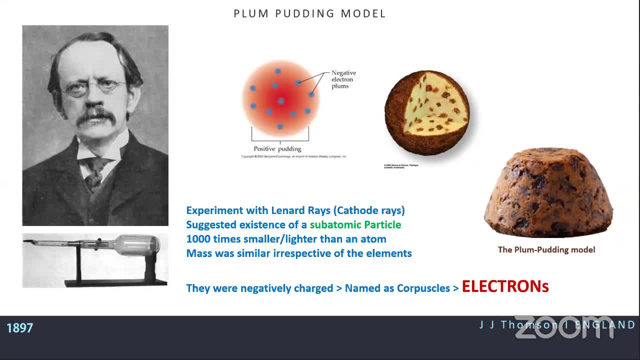 or lighter than the atom and having a negative charge, And this was common for all elements. I mean irrespective of all elements, So this is not be something common for all elements. So he named this negatively charged particles, corpuscles, And these were later named as electrons. So we found 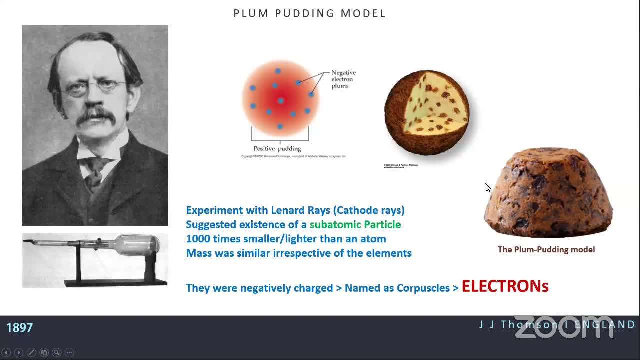 that for the negative electrons they were called electron. Now JJ Thomson also gave a model of atom which is known as Plum Pudding model, which is a British deserter, where you can see the resins are scattered in a in the pudding, And he said that the entire 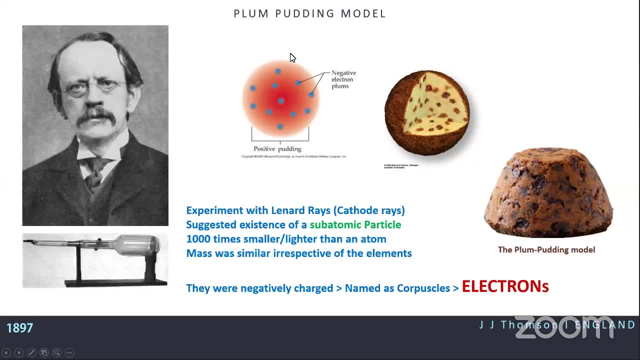 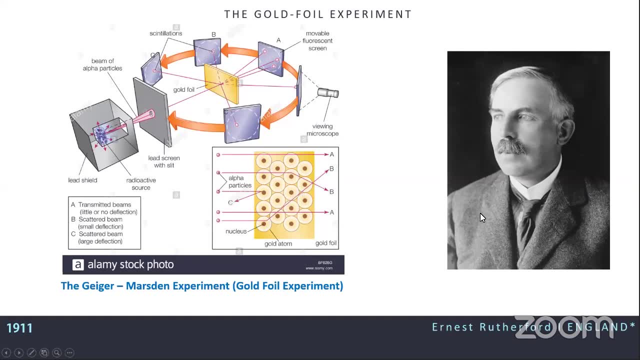 atom is basically a soup of positive material in which we have negative electrons. palms scattered discreetly the famous experiment by Ernest Rutherford, who was born in New Zealand and later established in England. He found that in the gold foil experiment he bombarded the gold foil with alpha particles. 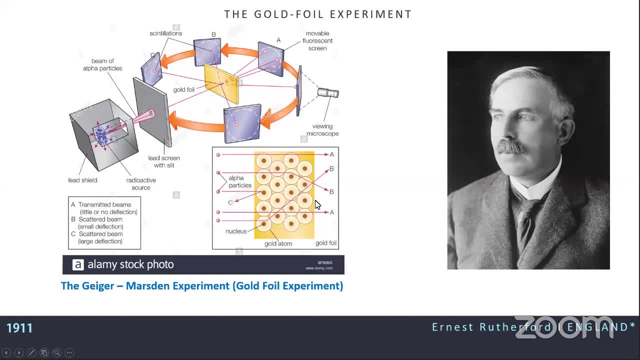 which are basically positively charged heavy particles. So these heavy particles, he found that most of the particles are going through and through the gold foil, But some of them are deflected and some of them are just coming 180 degree back. So from this experiment he concluded that the atom, which is basically a hollow structure, 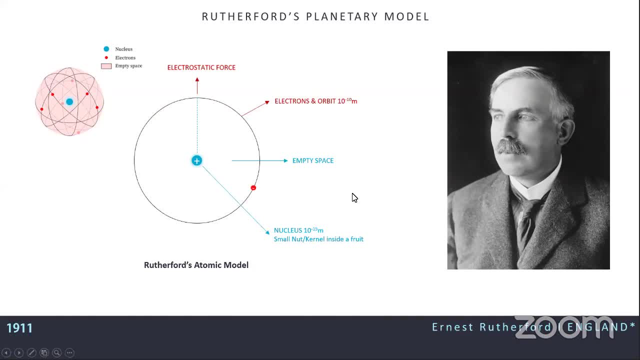 which is mainly the hollow structure, that is, the most of the part of the atom is empty And the center of the atom there is something, some positive charge, which holds these negative electrons by electrostatic force. And he said that these atoms rotate. 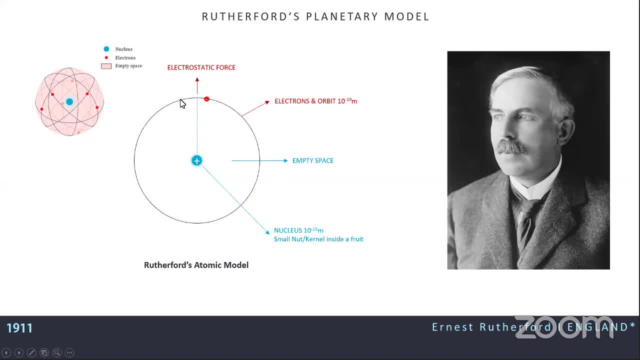 These electrons rotate around the nucleus in a planetary fashion, as the planet moves around the sun. So if you see the diameters, the nucleus has a diameter of 10 to the power minus 15 meter, while the atom has a diameter of 10 to the power minus 10.. 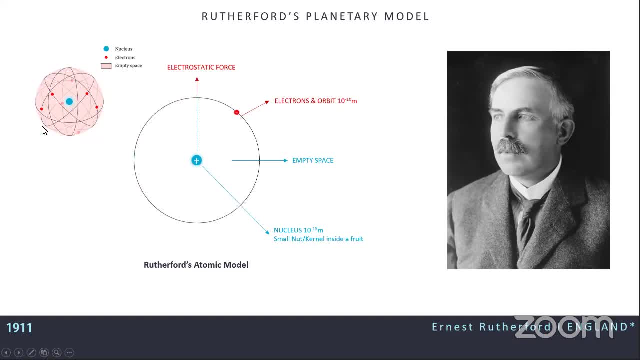 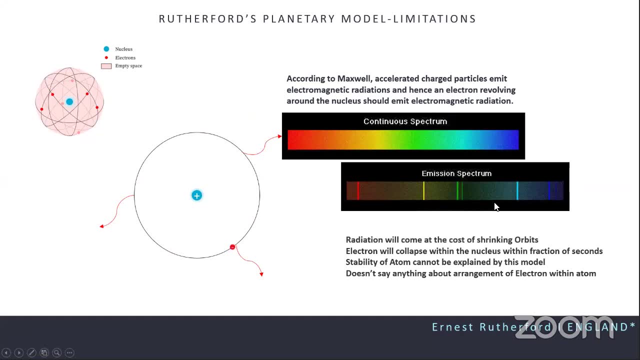 So the rest of the space is empty. That's why the alpha particles were crossing through. Now, the Rutherford model had some limitations. That is According to the theory of classic physics by Maxwell. he said that if a charged particle is accelerated, it will emit energy in form of electromagnetic radiation or electromagnetic. 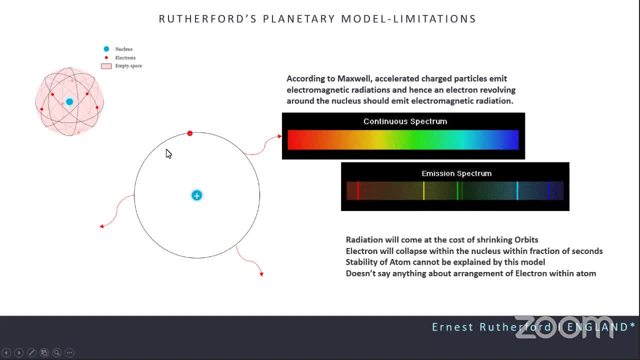 wave. So if the Rutherford model says, as the Rutherford model says, that the electron is moving continuously, so it will continuously emit some energy, So it should be that the energy should look like a continuous spectrum. But in reality from the atom the electron is moving continuously. 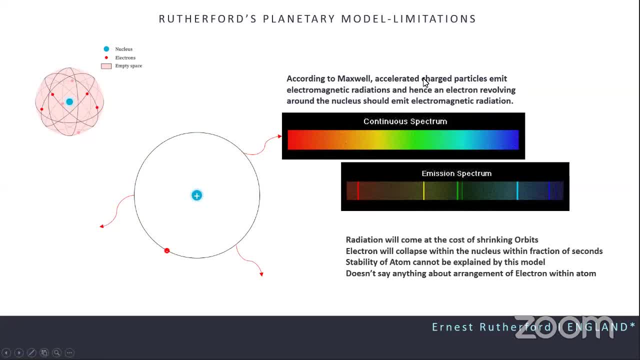 So it will continuously emit some energy. Sometimes we get discrete-energy spectrum, So by that the Rutherford model cannot explain this spectrum. On the other hand, if, as per the Maxwell's theory, if the electron moves in angular momentum, it will lose its energy because it will continuously radiate. 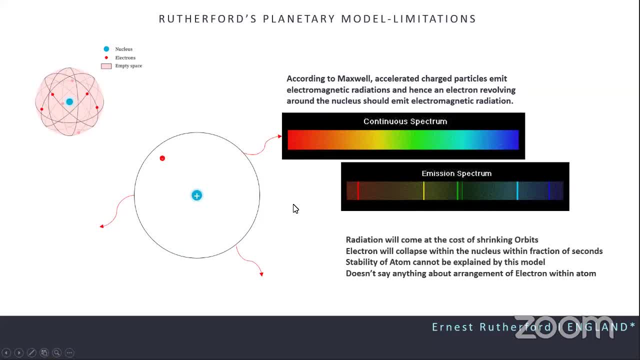 So its orbit will be shrinking continuously and ultimately it will fall into the nucleus And thus, with positive and negative colliding with each other, the stability of the atom will be lost, lost. So the Rutherford model cannot describe the stability of atom During this time. also, 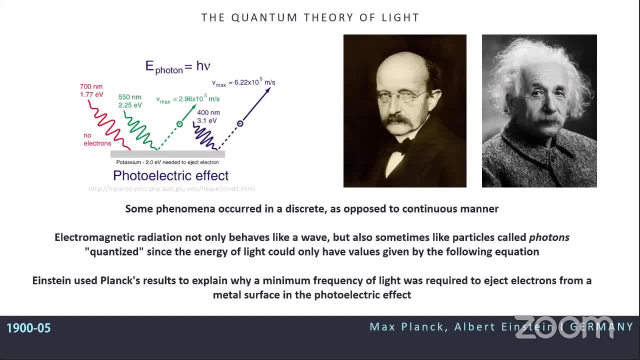 the famous scientist Max Planck and Albert Einstein. both of them developed a new concept of the light or energy, which is known as the quantum theory. That means they found that the light is no longer is a continuous source of energy, but they are actually packets of. 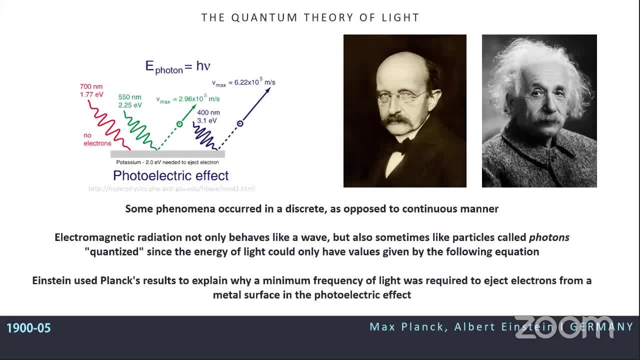 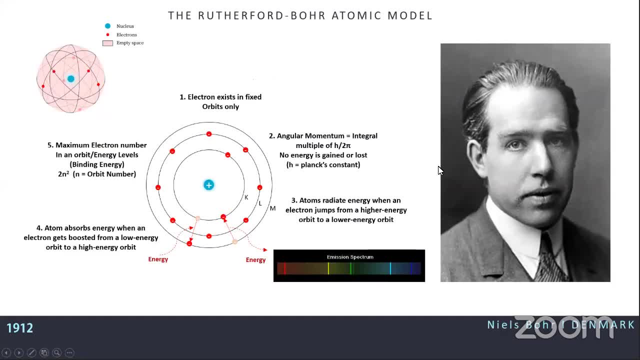 energy, or they named them as quanta or photons. So by this concept and with the drawback of the Rutherford models, Niels Bohr, who was also working with Rutherford, he developed a new concept of the atom. That is, the nucleus remains same in the center of the atom. but what he 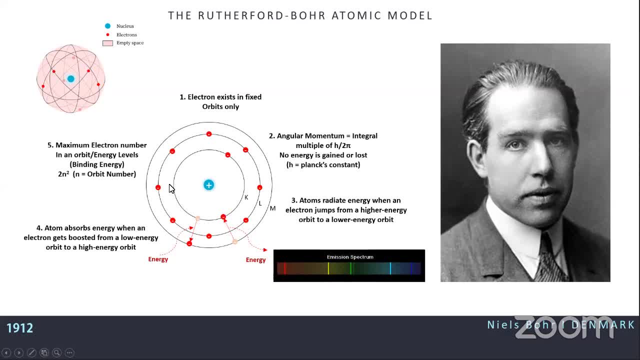 said is that the electrons rotates surrounding the nucleus, but in a fixed orbit It is only, and the angular momentum of this, or the electrons in this fixed orbit are constant, and that is explained by the Planck's constant. So, in this particular orbits, according to: 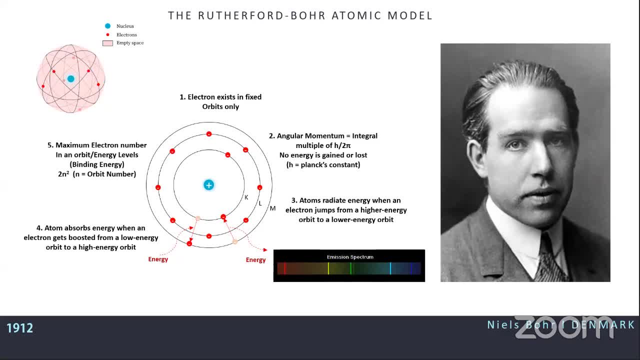 Bohr model that the electrons will not emit any energy or not absorb any energy. So the stability of nucleus can be explained by this model. and he also said that when the electron absorbs some energy from the inner shell, It will Jump into an outer shell and if it loses energy and it goes into the inner shell, it. 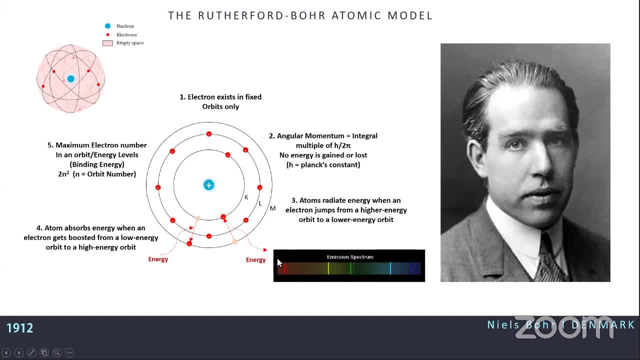 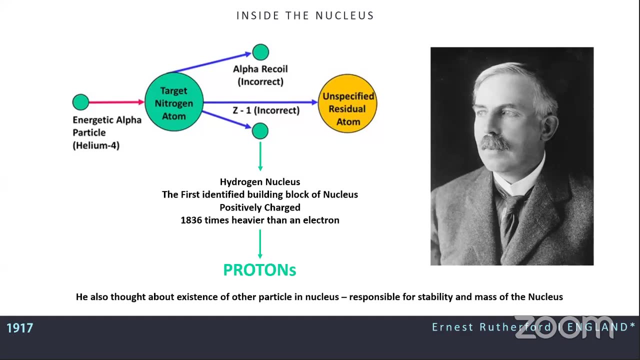 will give some energy, and thus we can have the discrete energy spectrum according to the jump from one shell to another. So this was given by Niels Bohr. Now what is happening within the nucleus now? Rutherford subsequently, in a few years later, found that when the air is bombarded with 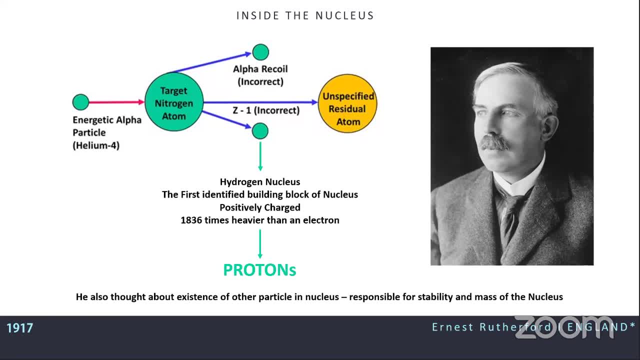 alpha particles. They found that the hydrogen nucleus are. You can find the hydrogen nuclear. nuclear are scintillating in the scintillators. So he found that the hydrogen nucleus must be a one of the building block of the nucleus which is responsible for the positively charged. 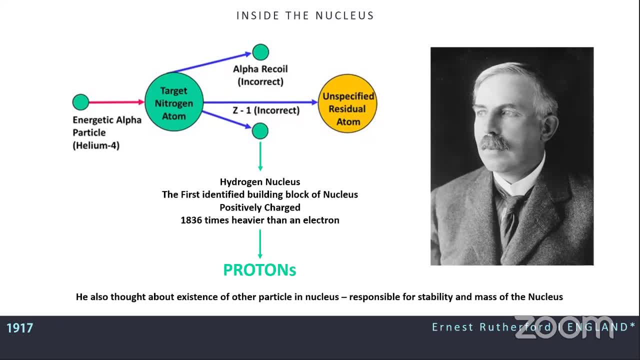 particle, and he also found that these particles are actually 1836 times heavier than the electron which was developed previously. He named them as Proton, as the first particle of the nucleus. You also thought there must be something else to in the nucleus to which is responsible. 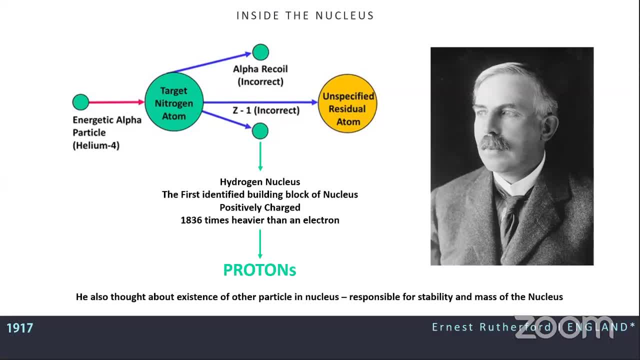 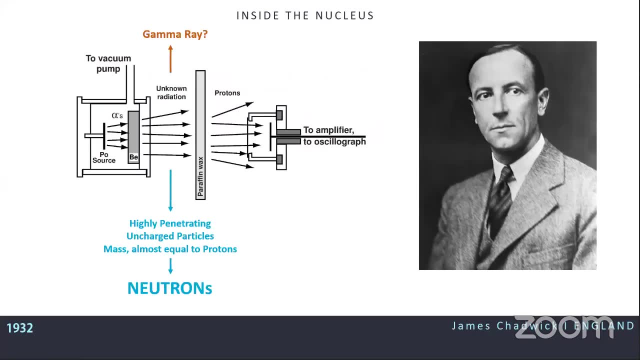 for the stability of the nucleus and the mass. but he did not further conclude about the other particle. Now the other scientists started to find what is the other particle. So they found that when a very light metal like the beryllium, They are radiating, They are radiating the 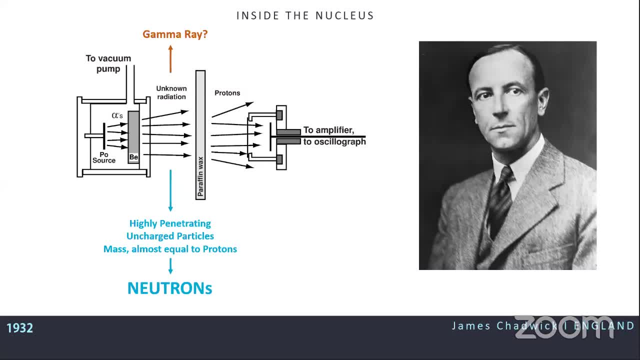 bombard with alpha particles like heavy heavy particles, They found the unknown radiation is being formed and these are neutral in nature. So, unlike alpha particle or proton or electron, which were previously charged, this radiation is uncharged. That means it cannot be deflected by electromagnetic field. So they initially found whether it is a gamma ray, but they 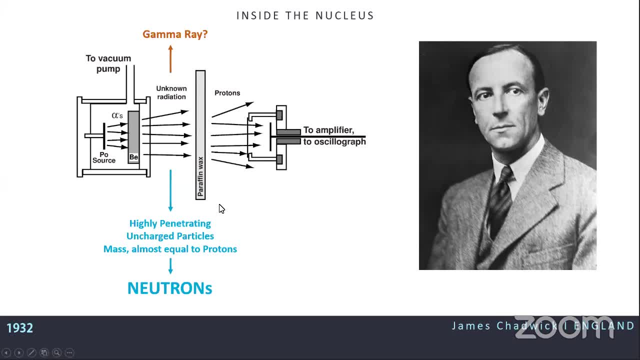 observed that the among these scientists were the Irene Curie and who established in Paris. They found that when the paraffin wax is used to this unknown radiation, this paraffin wax which is highly concentrated with hydrogen atom, they produce atom. That means these: 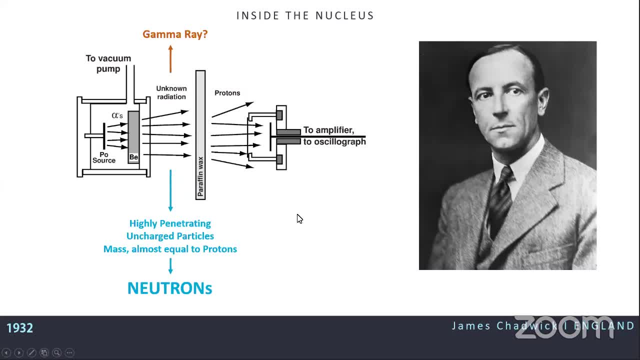 radiation must have a very high energy or mass so that they can explain protons from the paraffin wax molecule. So James Shadwick was a student of Rutherford. He established that this highly penetrating uncharged particle as particles rather than gamma rays. So he 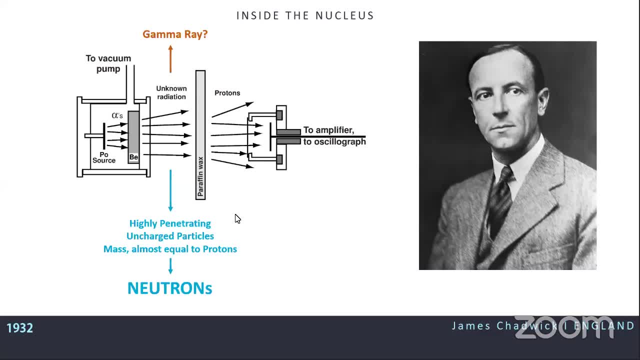 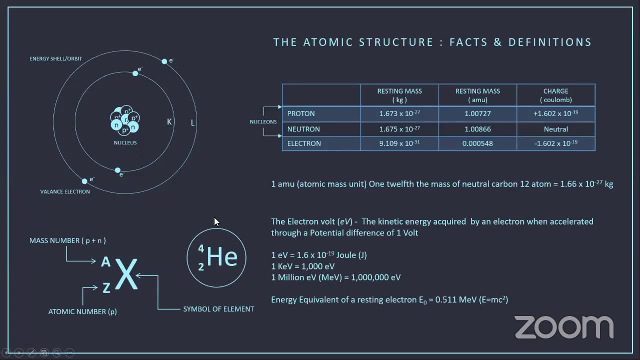 named them as neutrons according to their neutral charge. So with that we will come to a break with our current structure of the atomic structure. That is the nucleus inside, with proton and neutron- Proton being positively charged, Electrons are moving around it in. 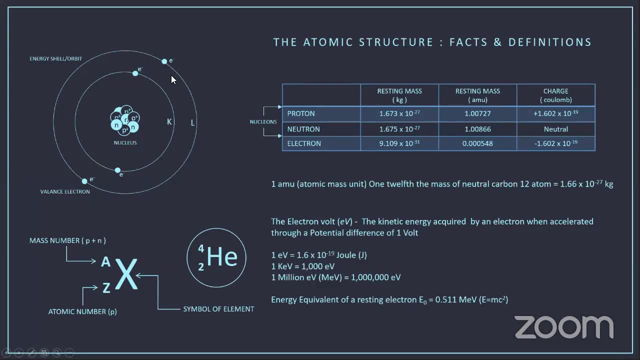 the K shell, L shell according to the Bohr's definition, And the number of electron is same with the proton, to keep the atom neutral. Now, with that we know how to describe an element That is. the X is the symbol of element like this, helium. Z is the atomic number or the proton number. that is true for helium. 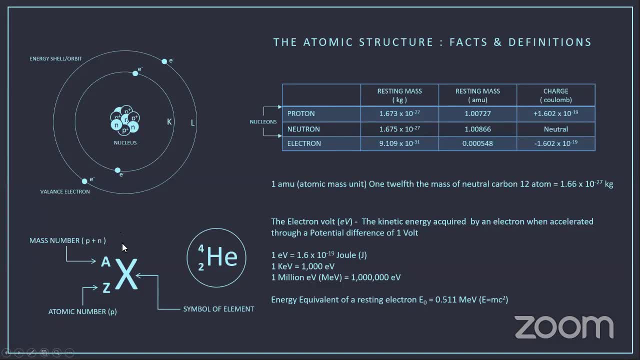 and A is the mass number, which is basically the number of proton plus neutron in the nucleus. This proton and nucleus is also known as proton and neutron is also known as nucleons, which constitute the nucleus. Now, with that, I have given some information. 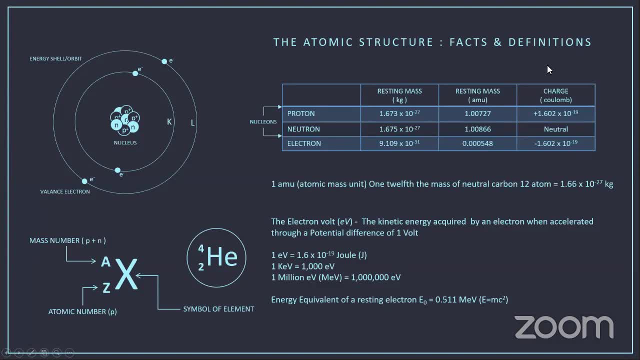 about these important charges and masses of these, all these particles. And you can see, the proton and neutron has almost similar mass and while electron is much lighter than them, And the electron and proton share the same charges, but in a different opposite, and they are opposite to each other. Now coming to some definitions. one atomic mass unit: 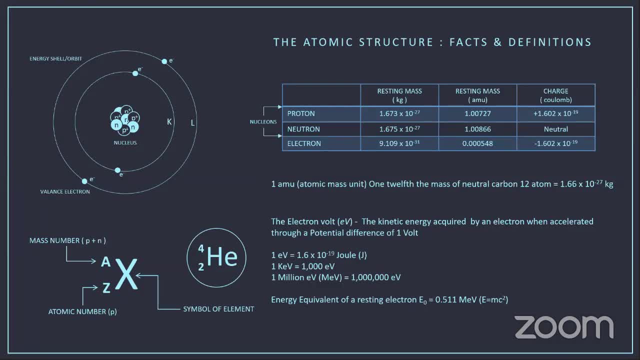 which is a unit to represent the mass, is basically one twelfth of the mass of a neutral particle. So the mass of a neutral particle is one twelfth of the mass of a neutral particle. So this mass is one ton of carbon 12 atom, which equals to 1.66 into 10, to the 1 minus 27 kg. And 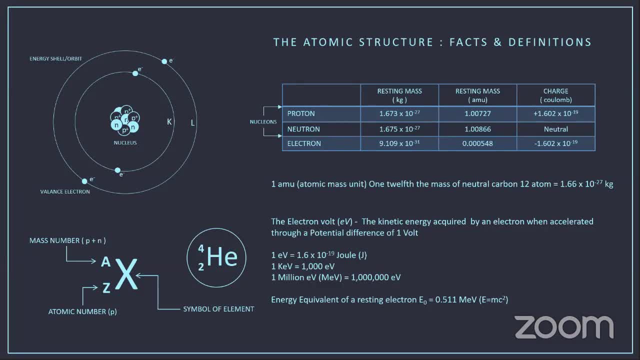 the electron volt is often used in the our radiation oncology subject, which can be defined as it is the kinetic energy acquired by an electron when it is accelerated in a potential difference of one volt. So, basically, electron volt is a measure of energy and it it can. 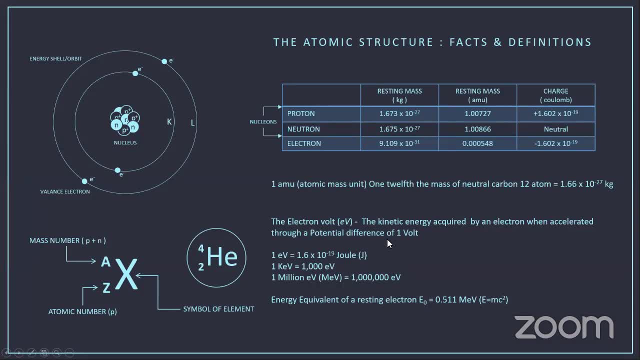 be explained, explained by the joule also. And one keV is equal to 1000 kV And this is actually the energy value of electron volt, equal to 1000 electron volt. and 1 million electron volt is equal to 10 to the 6 electron. 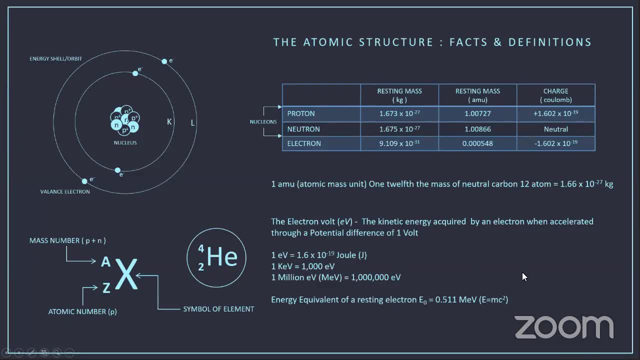 volt And this one MEB is very frequently used in our radiation oncology. This MEB unit is very frequently used in our radiation oncology system for describing the energy of radioactive isotopes And also, according to Einstein's formula of E equal to MC square, the resting. 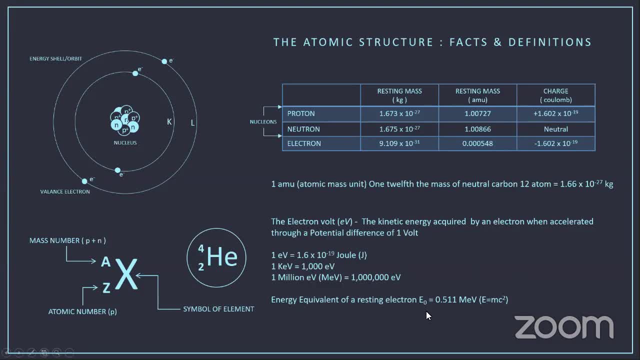 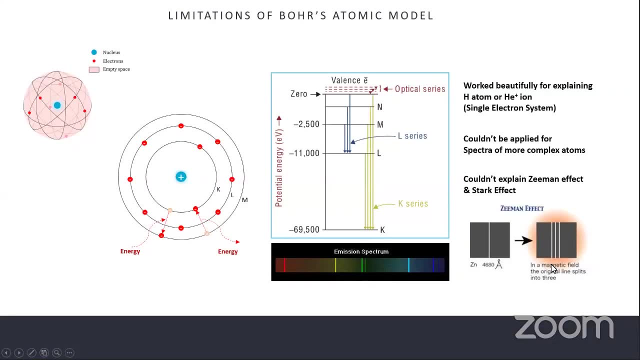 electrons. electron energy can be converted to. it can be equal to 0.511 MEB. Now coming to continuation of the atomic structure. So the limitation of Bohr model was that the Bohr model was worked beautifully when it was applied to hydrogen atom or helium ion. 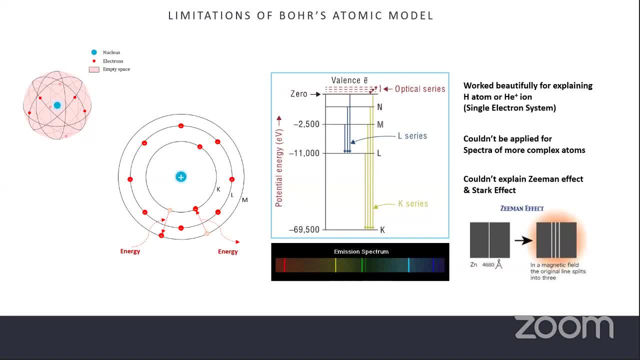 where there is only one electron is there, But when there is more complex atom and more electron are we producing complex electrons. So with spectrum Bohr model could not explain it properly And it also could not explain some other effect which are known as Zeeman effect of start effect, where it showed that 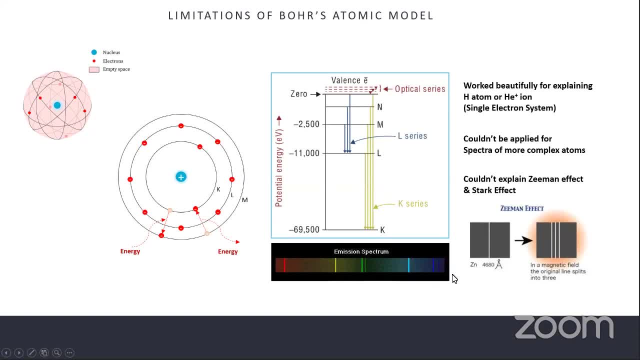 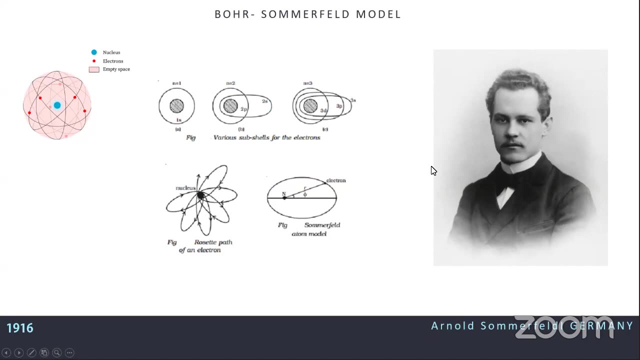 the spectrums are actually having fine lines rather than one line when they are exposed to magnetic or electric field. I will not go into detail of the electron distribution further but with this limitation of Bohr model, further models were developed by Sommerfeld. 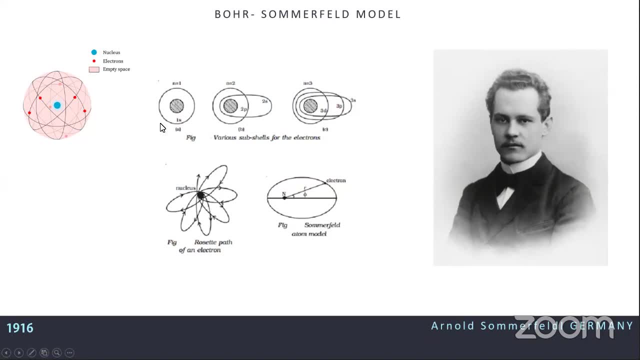 Bohr model, who said that the electrons are are not going to be able to be distributed in a circular way. The electron orbits are not always circular, but also elliptical, And the path is. it follows a rosette pattern, But till date, the pattern of electron distribution. 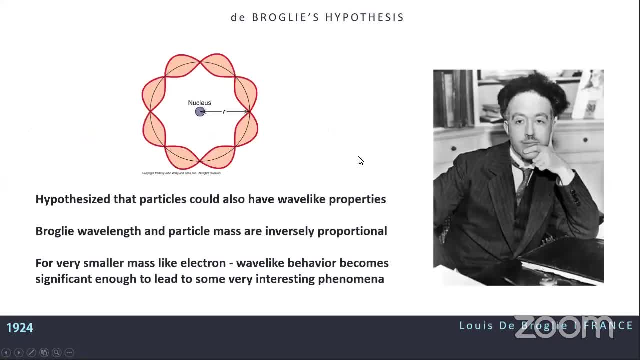 was 2D. The next hypothesis came from D Broglie, who is a faint scientist, who said that not only the wave can behave like particle, as said by Maxwell, said by Max Planck and Einstein. he said that the particles can also behave like particles, but they can also behave like 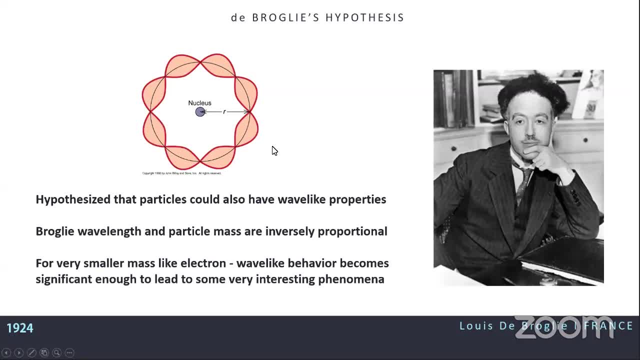 particles, And he said that the particles can also behave like particles, but they can also behave like waves. So the electrons at the smaller mass, like electron, the particles may also behave like waves, by which you can actually justify the nature of electron. And 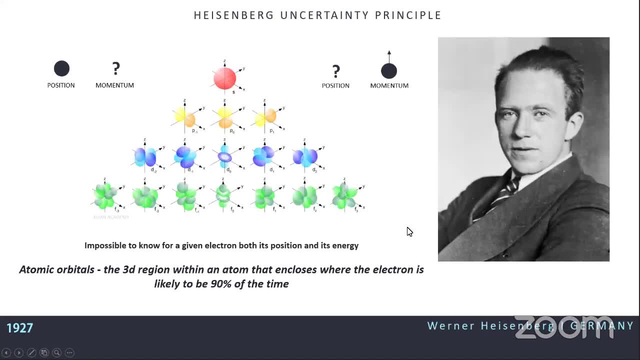 further. this concept was further added by Heisenberg's uncertainty principle to show that you cannot determine the position or momentum, that is, the energy of the electron simultaneously. So either you have to go for the momentum or position. So in the atom 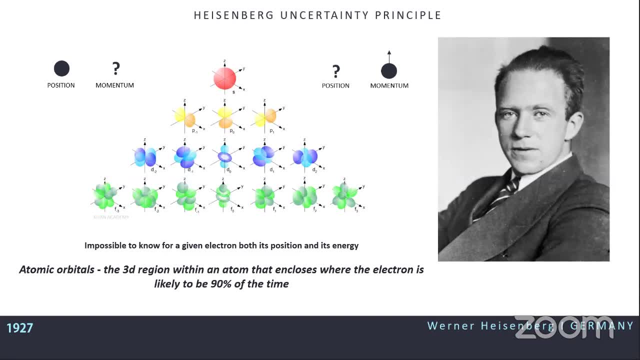 in the atom, the position of electron and all the momentum of electron is uncertain and he said that he the concept came like the basically electrons remain as a cloud is, or 3d region where nine, where it can be found in 90 percent time, and this equation was: these were mathematically 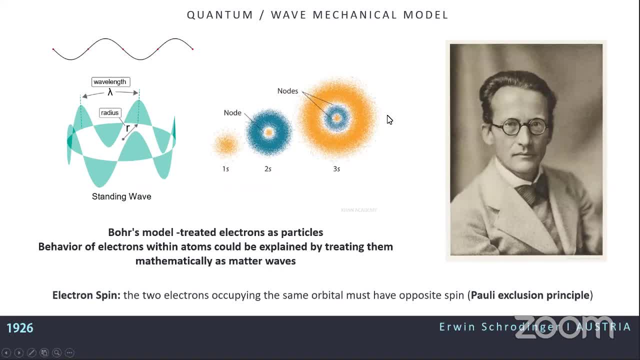 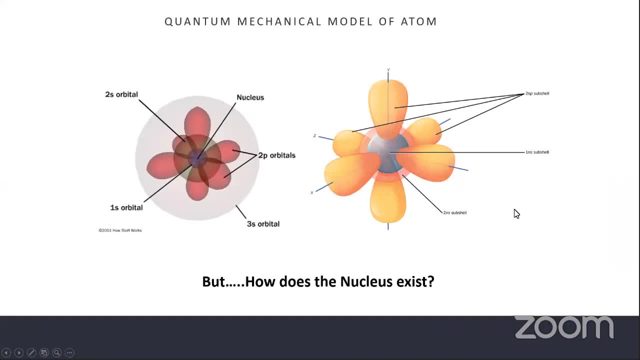 represented by schrodinger in 1926 by his model of quantum wave, mechanical model of standing wave. so we now we have come to the quantum mechanical model of atom. so we will not discuss about electron anymore, but we'll discuss about the nucleus. so the new, as we know, the nucleus is: 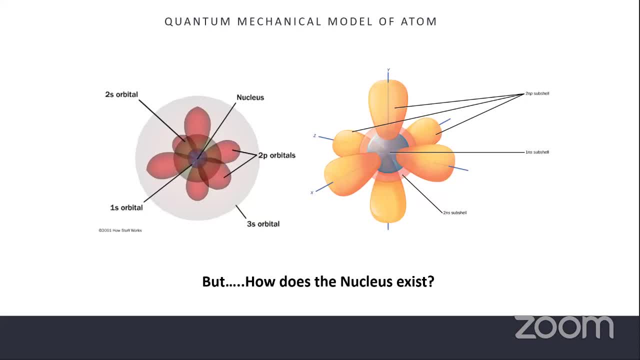 having positive charges. that means multiple protons which are positively, positively charged, now the as the electrostatic force. we know, the positive charges ripple each other, but how the nucleus exists then, because the positive charge, the proton, should ripple each other, but how they come together and exist simultaneously. So for that we come to the forces of nature. 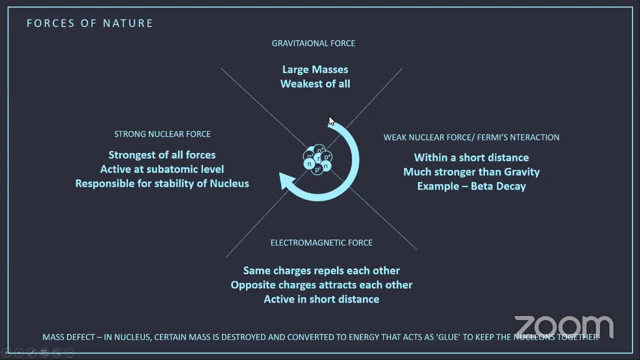 So we have four forces of nature and they are distributed according to their, from weak to strongest, weakest to strongest. So the first one, which is the gravitational force, is found to be the weakest of all forces, and it is applicable for large masses. We all know about gravitational 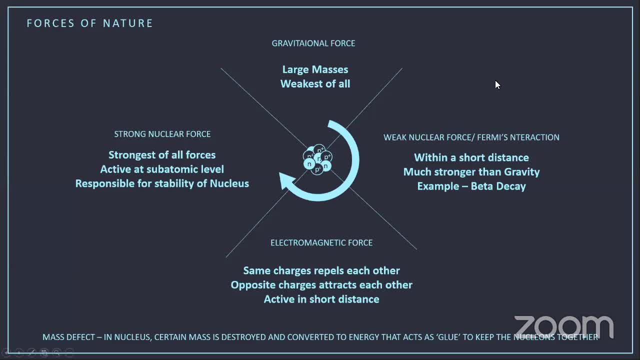 force. The next force is known as the weak nuclear force, or rather it is known as the Fermi's interaction force, which acts in a very short distance, in a subatomic level or maybe a distance of proton, but it is much stronger than gravity and it is usually associated with different types of 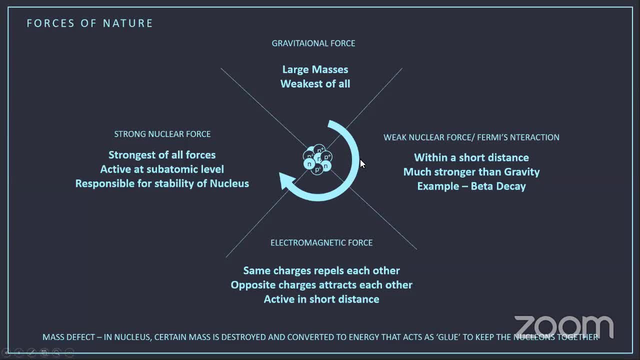 radioactive decay like beta decay. The next one is the electromagnetic force. We all know about electromagnetic force that the opposite charges attract each other. The next one is the electromagnetic force. We all know about electromagnetic force that the opposite charges attract each other and the same charges repel each other. Now this is also active in for short distance only. 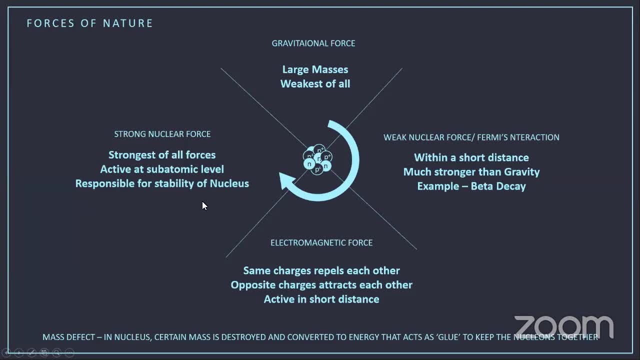 Now we come to the strongest of all, that is, the strong nuclear force, which can explain how the protons are held in the nucleus. These are active in subatomic level only and they are responsible for the stability of nucleus. Now how the strong nuclear force is. 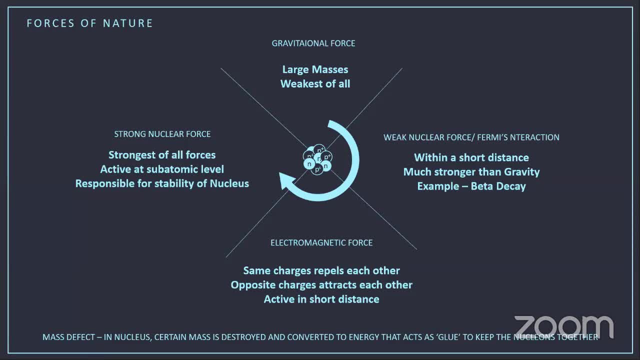 generated. The theory is that, as we have, we know, the nucleus is consisting of neutrons and protons. Now, the neutrons and protons, if we join their masses, so the mass of nucleus should be equal to the neutron and proton. but in practical it founds that the nucleus is having a mass. 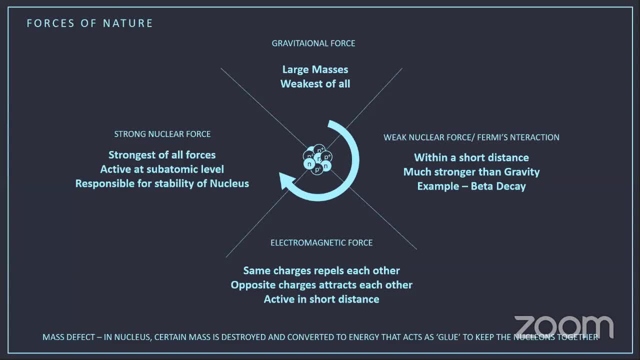 lesser than the summation of the mass of neutron and proton, So some of the mass is destroyed, which is known as the mass defect, and the concept is that this mass is converted to energy and this mass acts as a glue to keep the nucleons together. 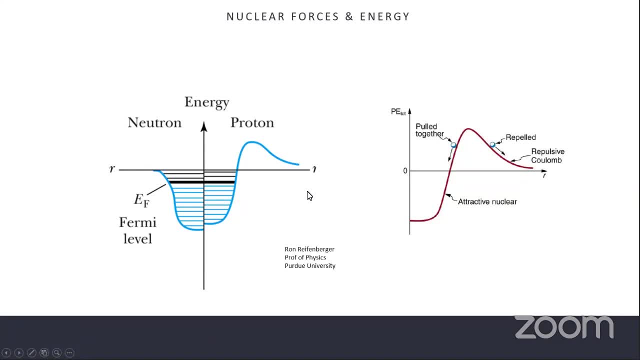 Coming to the further description of this particular strong nuclear force. So if, if you know, this strong nuclear force is acting in a very small area, or the radius, or radius of the nucleus, where, once, if a proton approaches the atom from outside, from an infinity range, the first he will it will face is a repulsion force due to the electrostatic force, because 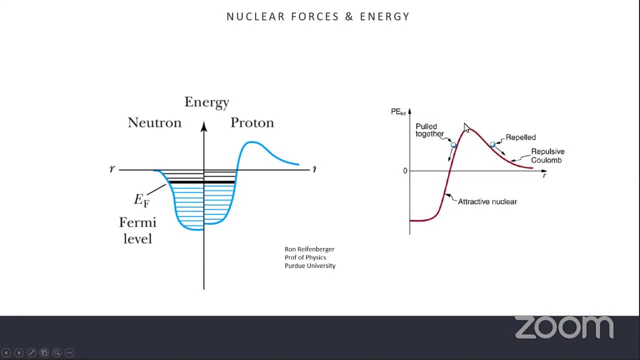 it is positively charged. So there will be a barrier to the. it will require more energy to cross the barrier. but once it crosses the barrier of this electrostatic force or the coulomb force, it will suddenly lack this barrier and it will be attracted within the nucleus by the. 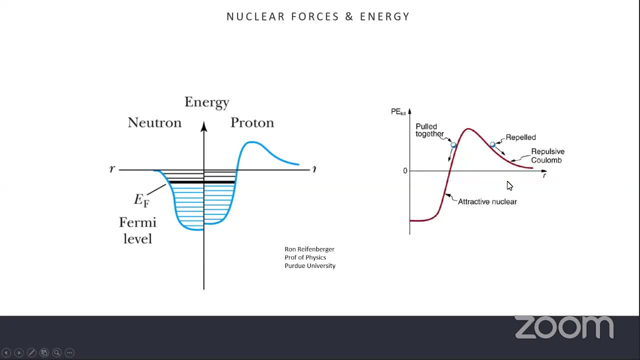 strong nuclear force. So you have to take the proton to a certain extent, to a very short distance towards the nucleus to have the strong nuclear force, and this is known as a potential one. So we have a very important point here and it is a very important point to note as well. 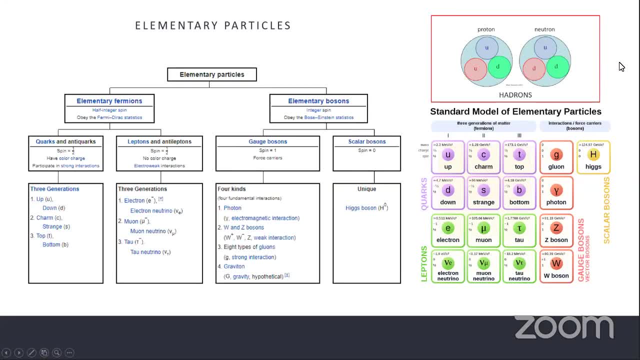 where the protons are attracted. So very few words about the elementary particles. which time it was discovered that the proton neutrons are not is not something which cannot be further divided? It was found that the protons and neutrons are basically made of some quarks, which are also known as fermions, and this glue thing. 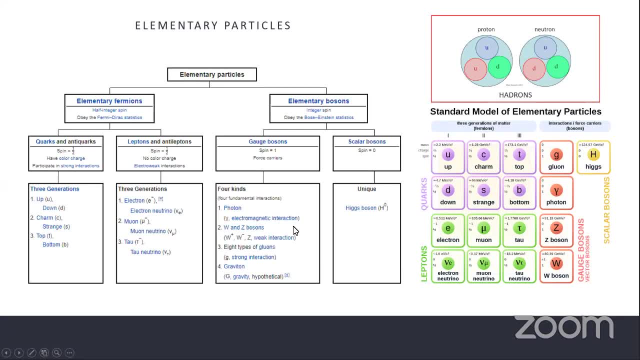 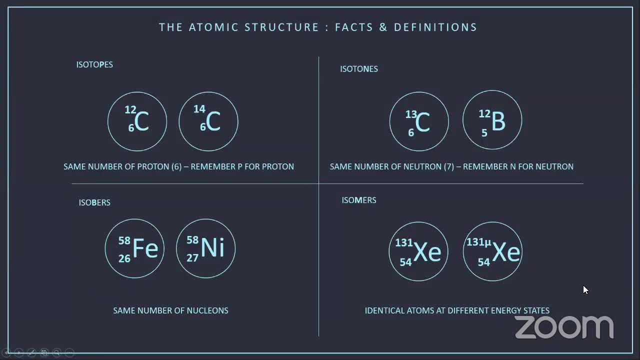 which is basically keeping them together is of which are also type of elementary bosons. We will not go into further detail for the elementary particles. So with that we come to some other important definition, which are known as isotope, isotones, isobars, isomers. So what are isotopes? Isotopes are basically two atoms with similar 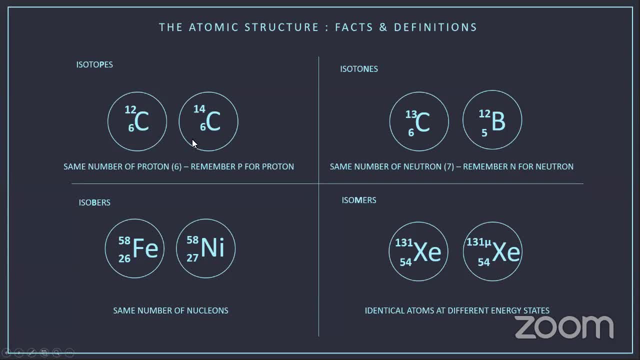 proton number. How to remember p for p? So the proton number will be similar for the two atoms, but the atomic weights are different. Isotones are similarly n for n. That is, the neutron numbers are equal for both the atoms, but the proton numbers are different. So in here you see both in both. 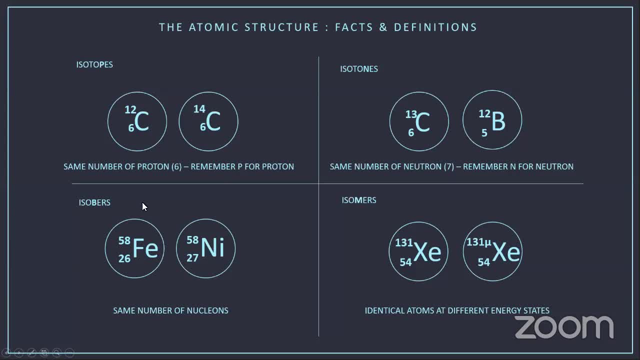 cases, the neutron number is 7.. Now come to isobars. They are basically with same number of nucleons, that is 58. They are called isobars And lastly, isomers. The isomers are basically similar atom, but at a different energy states. We will 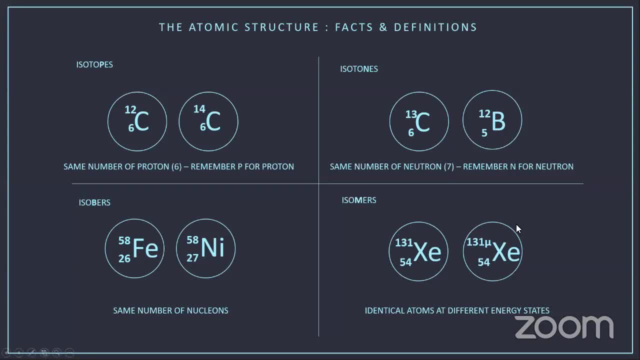 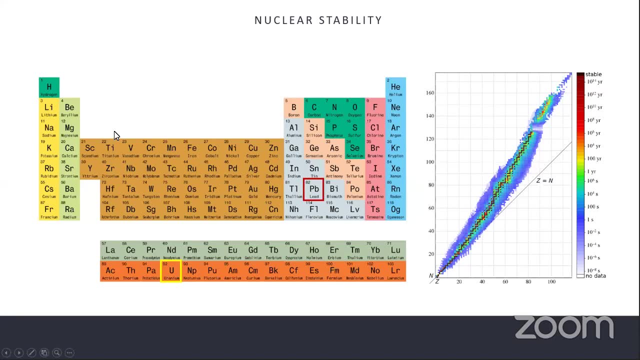 talk more about the isomers when we will talk about radioactivity. Now coming to the nuclear stability. So, as we are saying, if you see the periodic table, that as we increase the number of protons, that the z number, the neutron number, also increases. And if you plot the z number and 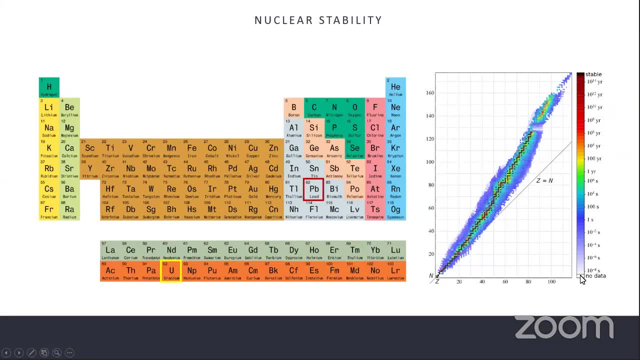 the neutron number in the x and y axis respectively. you see that this is the ratio, The ratio of n by p, or known as n by p. where z equal to n, You can see up to 20 atomic number, the actual, the elements follow more or less n by p of 1. And then this starts moving towards. 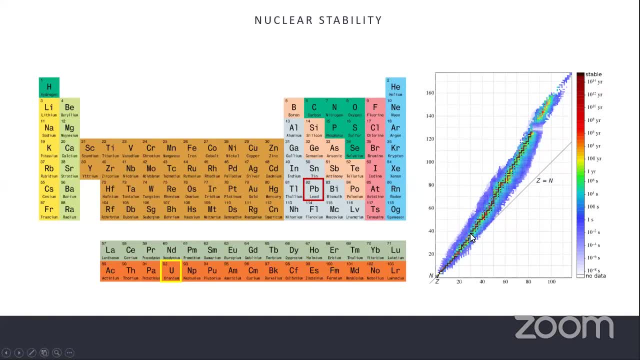 the neutron side And if you see this black line, which is basically this line of stable nucleus who maintain more or less a stable neutron to proton ratio, But as they go towards either towards this blue side, either towards the neutron side or towards the proton side, 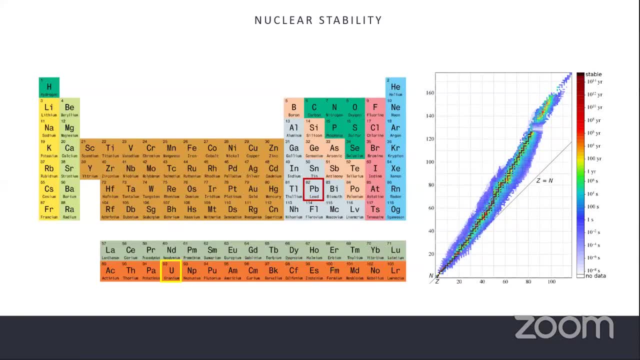 they became unstable because of either more number of neutron or more number of proton, or if it goes beyond 82, that is the blade, which is the most stable compound. It becomes unstable due to heavy weight, So they try to become stable by emitting some particles or some energy to become stable. So over 300 isotopes are. 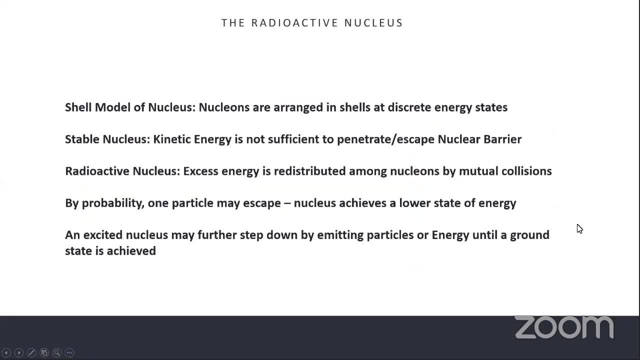 distributed in such way, So by the way they emit. this is all known as the radioactivity. So if you see the radioactive nucleus, what happens in normal nuclear? the kinetic energy of the particles are not sufficient to penetrate or escape the nuclear barrier. But in radioactive nucleus- this- they have some excess energy which is redistributed. 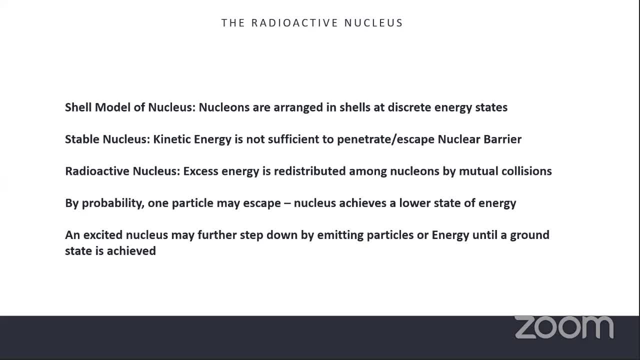 in the nucleons, By probability they may escape and the nuclear achieves a lower state of the of energy and they can further go to step down to a lower, a further lower step when emitting, by emitting particles or by emitting some energy to the ground state. Now this phenomena, which is 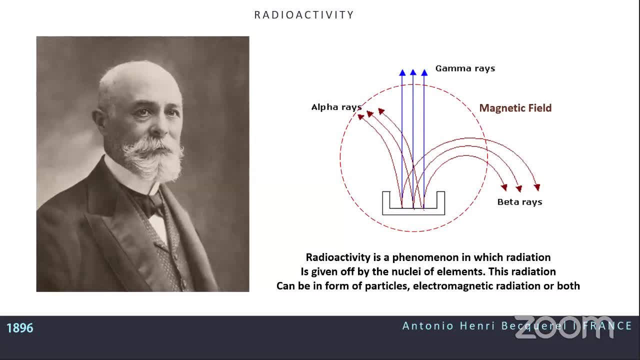 known as, by which the radiation is given off from the nuclear element is known as radioactivity, which was discovered by Henry Becquerel, who was a French scientist, in 1896, and this can be either particle or can be electromagnetic radiation, or can be both. So what he did, he got interested in 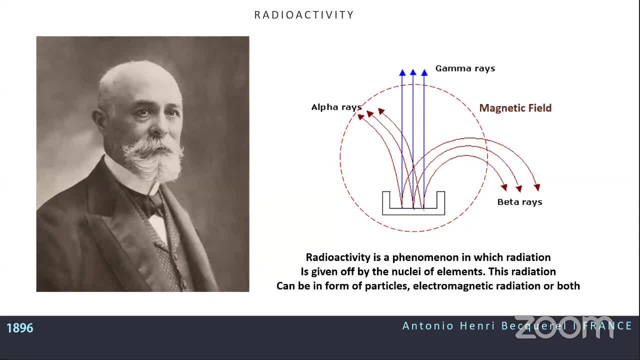 phosphorescence study and when sir Rondion developed x-ray, he thought that there must be some similarity with the phosphorescence, with the x-ray, and he started experimenting with uranium salt and he found that uranium salt can give three types of radiation. One is a light. 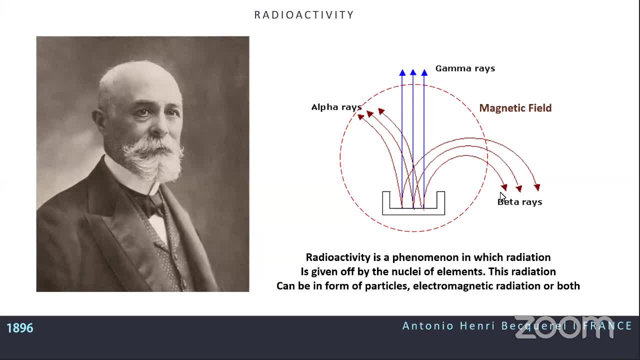 particulate radiation which is negatively charged and deflected in the magnetic field. One is heavier particulate radiation which is deflect, which is positively charged and deflected in a opposite field. and there are some other radiation, which is basically energy, which is not influenced by any magnetic field. So actually these were alpha ray, beta ray. 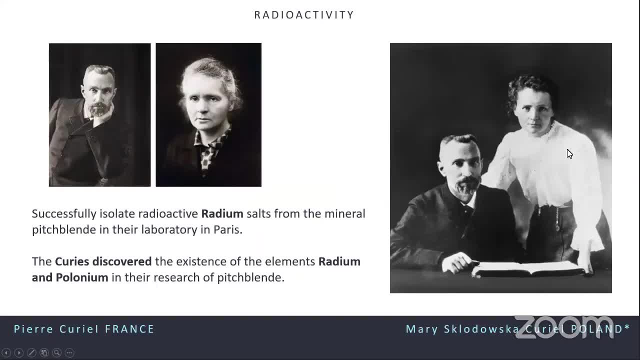 and gamma rays and for this discovery with Pierre Curie and the famous Curie couples. Pierre Curie and the three of them received Nobel Prize for the discovery of radioactivity and the Madam Curie named the term radioactivity, Who later discovered radium and polonium in their research on fish plane. Now coming to the types of 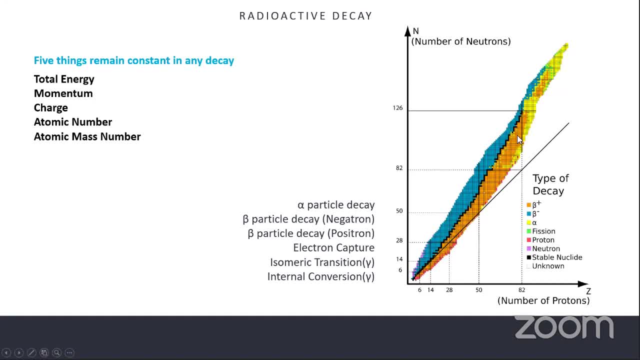 decay. so, as we've already said, the elements want to become stable by decaying some particles. so to see how to decay, if you see these elements which are orange in the, they are having more protons right, because they are having more z number. So they will try to. 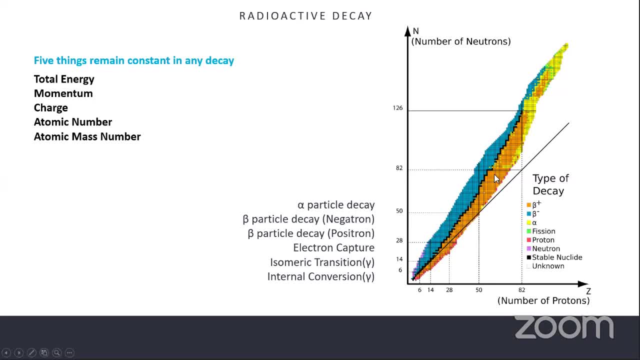 decay by some positive particles or in more, so that they are get rid of protons and they go towards more neutron. Why So this is? and why the opposite is observed for the other other, for the blue particles. I will come to that. So with that we come to the types of radioactive decay. 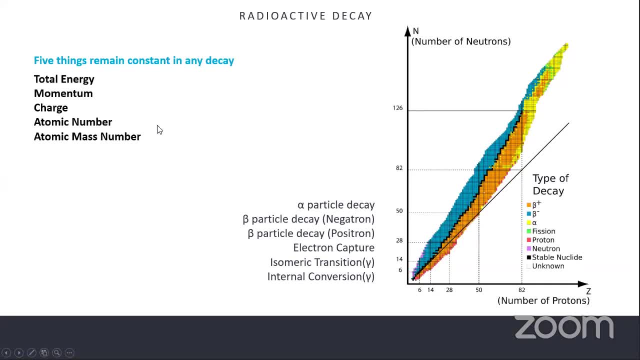 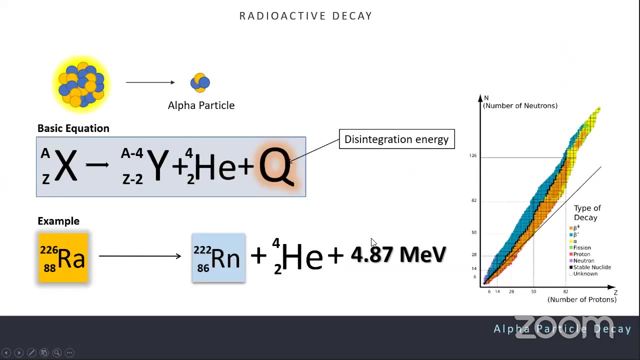 So, in any decay, these five things remains always constant, That is, the total energy of the of the system, the momentum, which is equivalent to energy, the charge, the atomic number and the atomic mass number. There is no destruction. So coming to the first type of decay- alpha decay, The alpha decay. 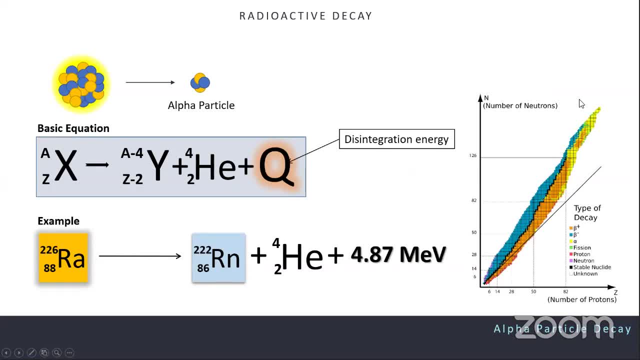 happens when the atom becomes very heavy. That is the 82 is the number of lead, proton number of lead. So lead is the more stable component, As I have already said, most stable element, beyond which the elements become unstable because of their weight, So decay by. they decay by mass, which is the helium nucleus. 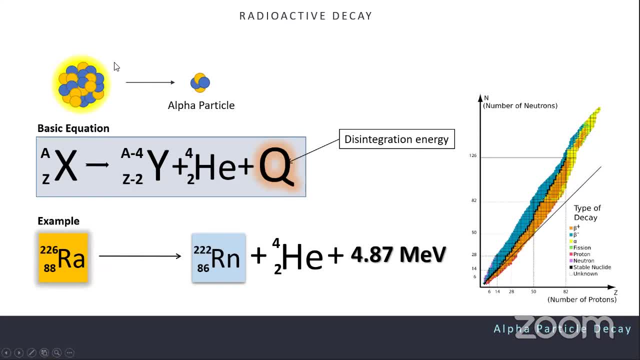 or a combination of one, two neutrons and two protons. So they give give rise to alpha particles and along with that they also give some disintegrating energy. The alpha particle takes this energy and comes out of the atom with kinetic energy and as the 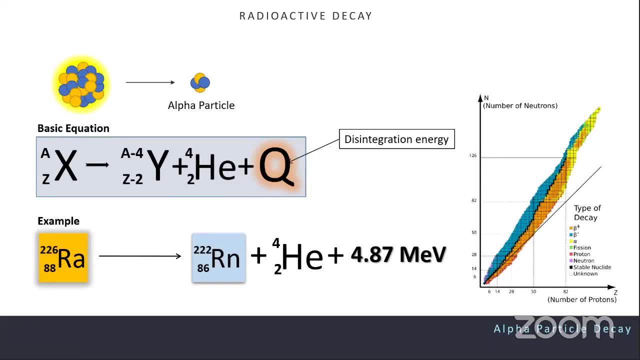 atom has much heavier weight than the alpha particle. the energy and the kinetic energy received by the atom is much less. Now the classical example- alpha of alpha decay, is radium. The radium decays by alpha decay to form the radons. So this region is the decay of alpha. 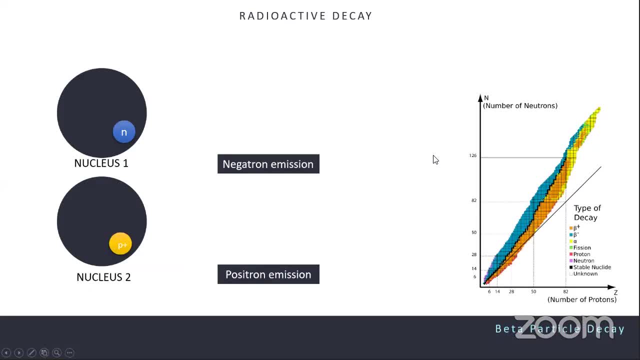 Now coming to the next type of decay, which is known as beta particle decay. So beta particle decay, as we said, that for this area, who has more neutron, what they will do? one neutron will be converted to one proton, one negatron or which is equivalent to electron, but because it is coming from nuclear, 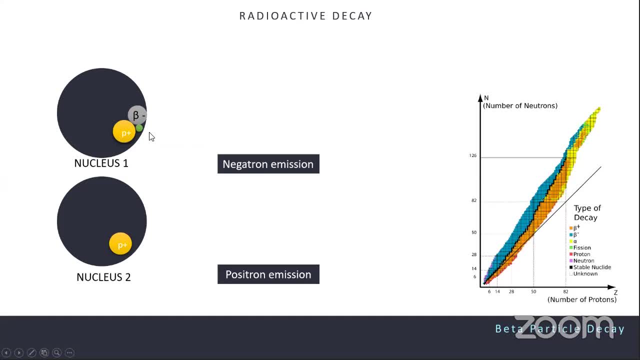 it is caused as beta minus or negatron and one antineutrino. So this is possible because we now know that proton, neutron are all made of quarks and they are interchangeable. So now, this way, the atom will decay by beta negative or negatron emission. So this is the area of negatron emission. 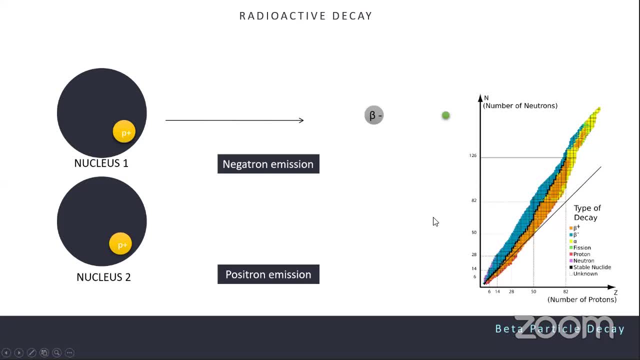 because they need to get rid of the high neutron count and they want to go towards the proton side. Now, oppositely, the proton side will start, will divide into one neutron, one neutrino and one beta positive particle, or which is known as the positron And this positron. 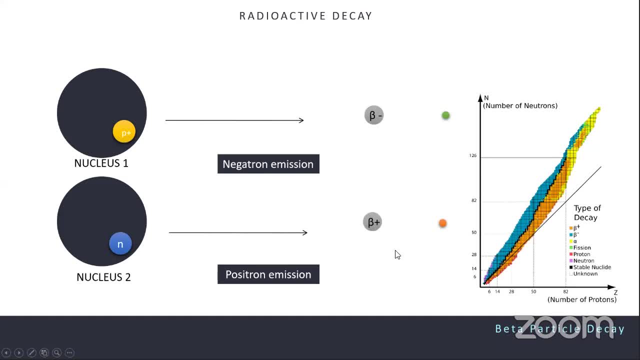 by this they will want to get any stability. So this is a quark. Now these wysotron aurait is known as positron emission. Eventually the positron cannot stay and it will react with another electron in the system and will develop annihilation reaction. So these are the example. 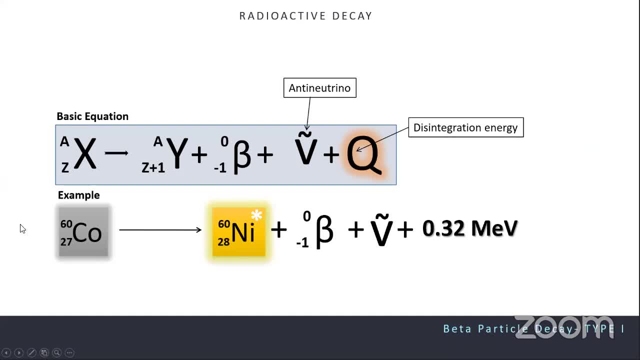 of beta particle decay or negatron emission. Cobalt-60 source decays by beta particle decay, which is the classical example of beta particle decay, and it forms a nickel source which is radioactive, which is in a metastable form of isomer of nickel. We'll come to know what happens. 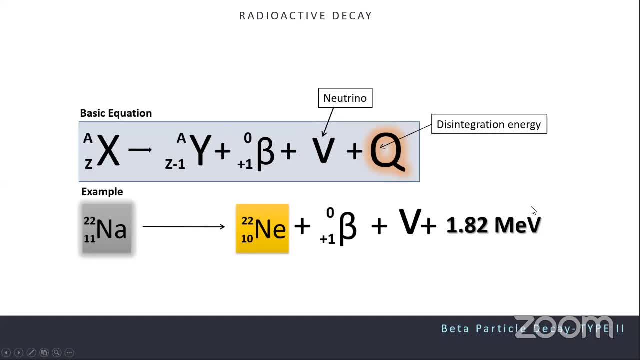 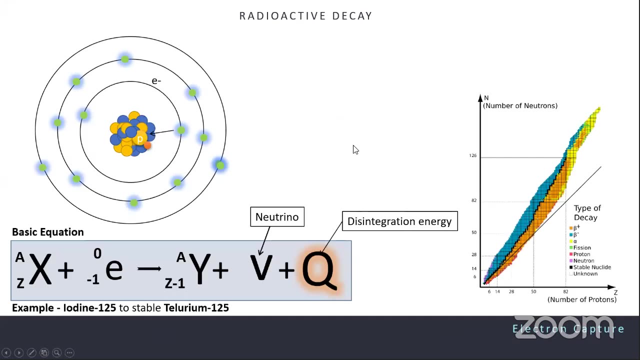 next to the nickel in later part. Now coming to the positron emission. sodium 22 typically decays by positron emission and the forms a neutrino and beta particle, with this disintegration energy. Now coming to the another mode, which is known as electron capture, Often seen in iodine. 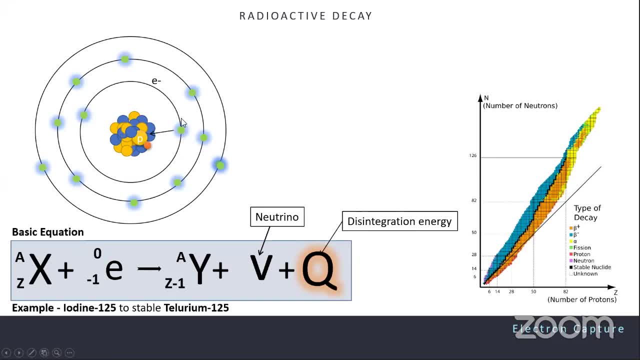 and tellurium. when an electron which is close to the, in the closest orbit, is captured within the nucleus Due to strongest force of attraction, and what will happen? the electron is a negative one, so it will react with the proton to form a neutron and a neutrino. Thus the neutron, the electron is. 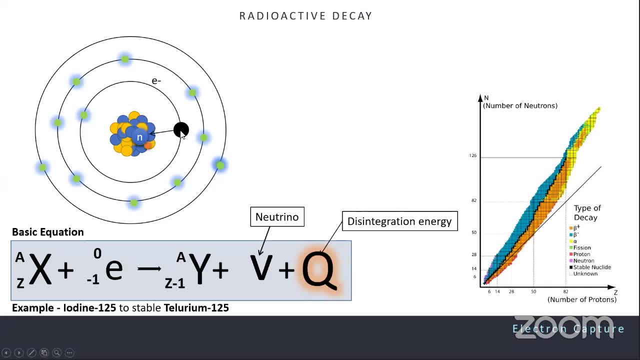 captured in the nucleus will create a hole or vacancy in the orbit. So this vacancy will be immediately filled out from one electron from the outer orbit. So, as per the Bohr's theory for jumping of electron from this part to that part, it will emit some. 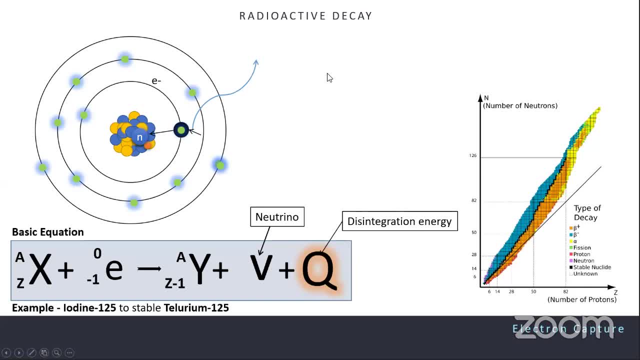 radiation. So either it will emit the energy as form of radiation, which is known as characteristic x-ray or phosphorescence x-ray. Why characteristic x-ray? because it is characteristic of this particular jump from this orbit to this orbit, And otherwise, if the characteristic x-ray is 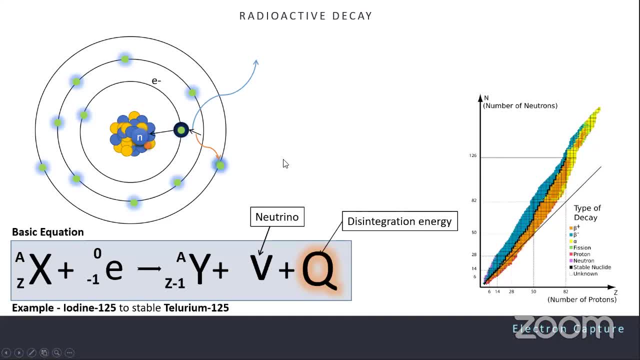 absorbed by this one outer shell. electron or free electron, absorb the energy and it will have the energy to move out of the binding energy and this will go out of the electron. So it will move out of the binding energy and this will go out of the electron. 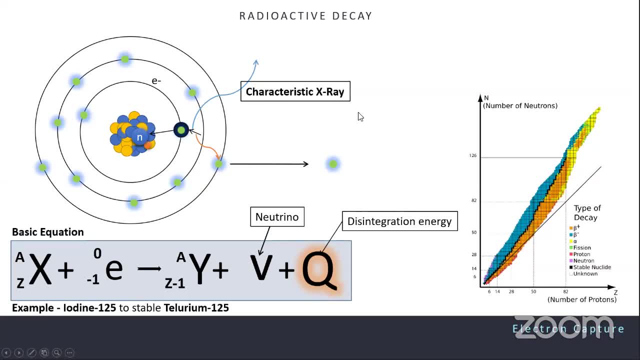 Which is known as Auger electron. So this is known as characteristic x-ray and this is known as Auger electron. So this is the Auger electron phenomena is mostly seen in low atomic number masses, while characteristic x-ray is characteristic of high atomic number masses. So this is electron. 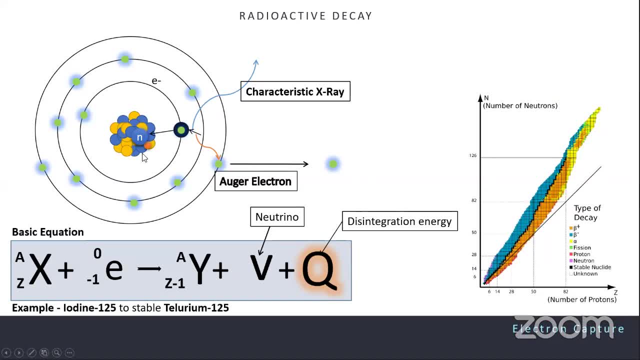 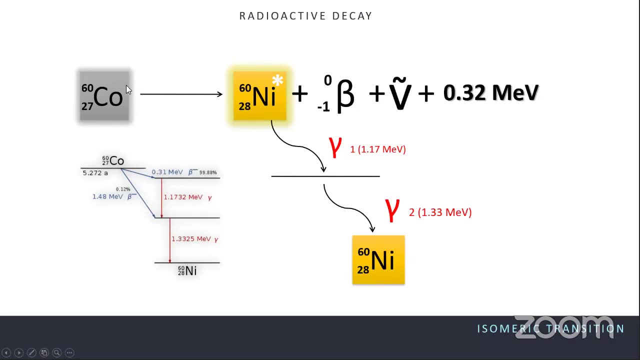 capture phenomena, where also the atom is getting rid of proton. So electron capture also occurs in this side of the NP ratio curve. Now coming to the isomeric transition of gamma decay. So here, as we know, the cobalt 60 is decayed by beta, but which forms a nickel of nickel. 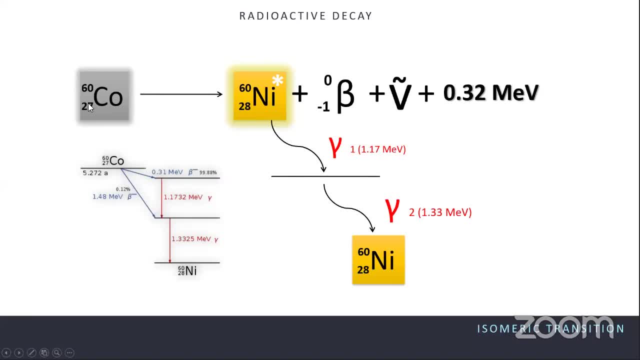 60, which is basically, you can see, the proton number has changed, So the element is changed, but it becomes, with the energy, in a high energy, non-metastable state. So it will emit, in two steps, two gamma rays of two different energies. See, this is the MeV. This is why I was talking about the MeV. 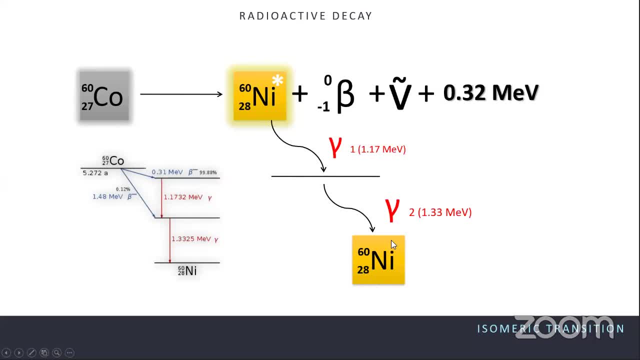 This is the energy of gamma rays and will become stable by emitting this energy And this is the classical cobalt decay, cobalt 60 decay scheme which is often asked in exams. So the decay of initially by beta and they will decay by two separate gamma rays. 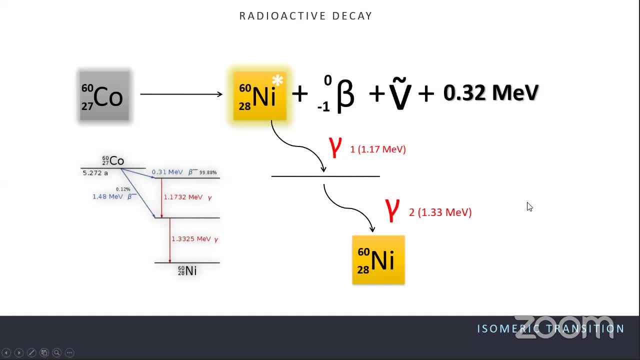 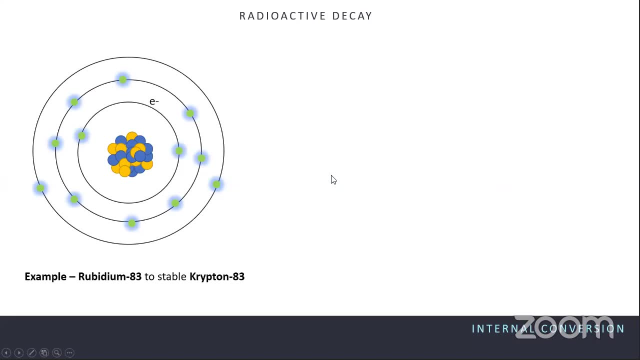 And, if you see, the average energy will be around 1.25 MeV by averaging these two energies. So another form of radioactive decay is internal conversion, Where a radioactive nucleus will emit some energy and will give it to the electron which is close to the nucleus And this electron by absorbing this huge energy. 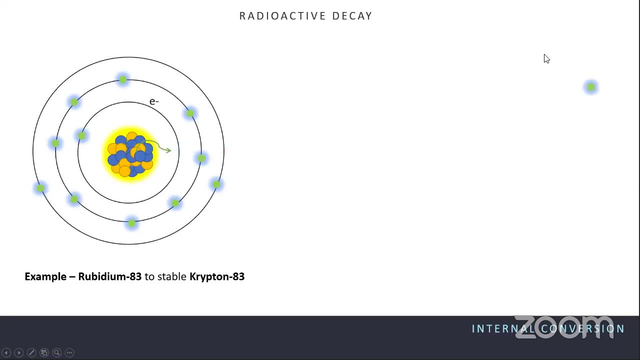 will release the binding energy and go out of the atom. So again a shell will be created. vacant shell will be created where the electron will jump from outer surface and again it will give rise to characteristics of x-ray. So this is the cobalt decay. So this is the cobalt decay. 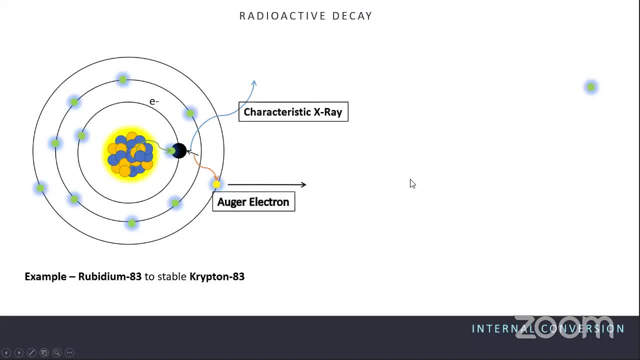 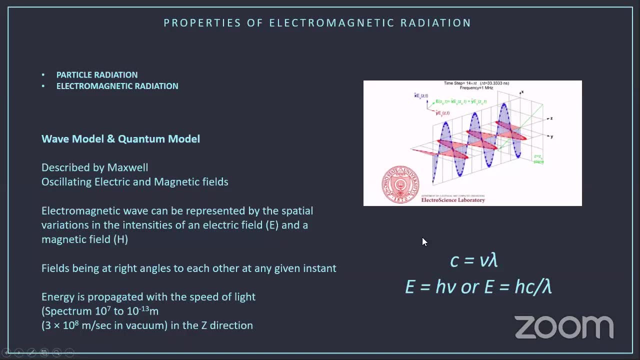 And in the� Producent Toxin or Auriga bagām or as electron similar to the electron capture phenomena. So with that we complete the radioactive decay type. Now let's come to the properties of electromagnetic radiation, which was given by Max Nicole. 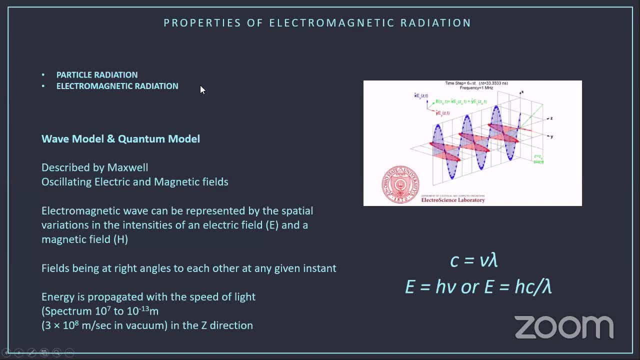 So by this time we know that there are two types of radiation: Either in form of particle, that is, alpha particle or bit of particle, or in form of electromagnetic radiation, like gamma rays, which are basically energy. And, as we know, this energy, this electromagnetic radiation, 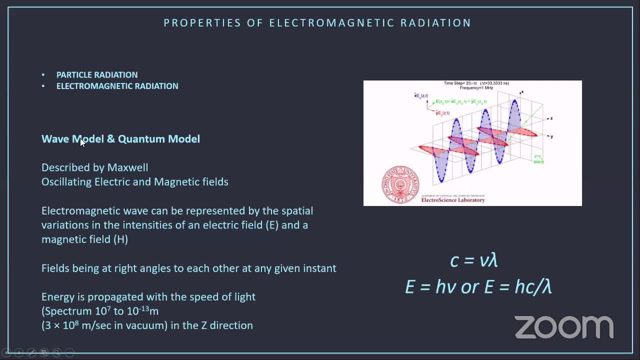 be explained by two types. One is the wave model of energy or the quantum model. The wave model is where it looks like a wave, or the quantum model where they can be explained by packets of energy. So the wave model was described by Maxwell. They say that the electromagnetic wave basically 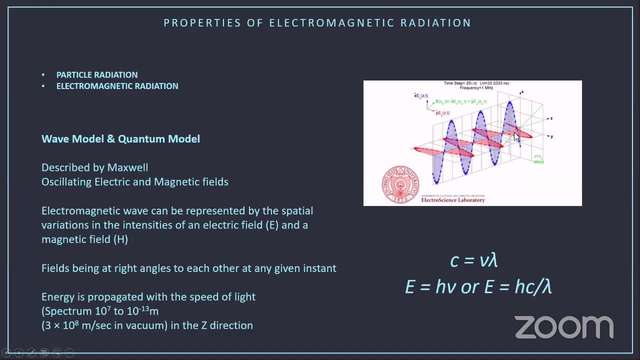 oscillates in two fields, the electric field and the magnetic field. And this electric field and magnetic fields are perpendicular to each other at a given instant. And also the direction of the electromagnetic wave is in z-axis. So if the electric force is in x-axis and the 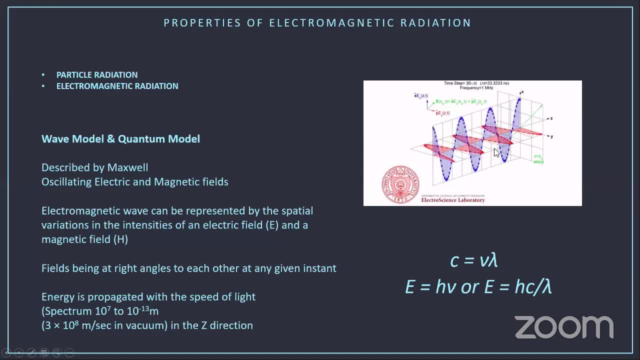 electric force is in x-axis and the magnetic force is in y-axis, the electromagnetic wave will go in the z-axis, So the three axes can be defined. The energy of the electro electromagnetic wave is that it can propagate to the speed of light And it has got a spectrum of 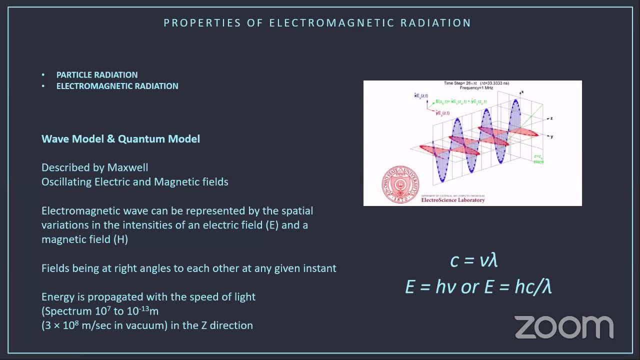 10 to the power, 7 to 10 to the power minus 13 meter. So it is. it ranges from the radio wave to very high energy x-ray waves. This is the electromagnetic radiation. In contrast, if you see the particulate radiation, they cannot attain the speed of light. Rather, according to 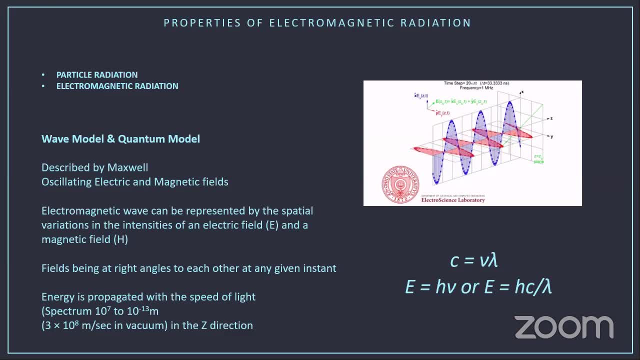 the theory of Einstein, if they want to attain the speed of light, they will gain mass according to the theory of real energy. So that is the energy of the electromagnetic wave. So the energy of the electromagnetic wave is that it can propagate to the speed of light And it has got a spectrum of 10 to. 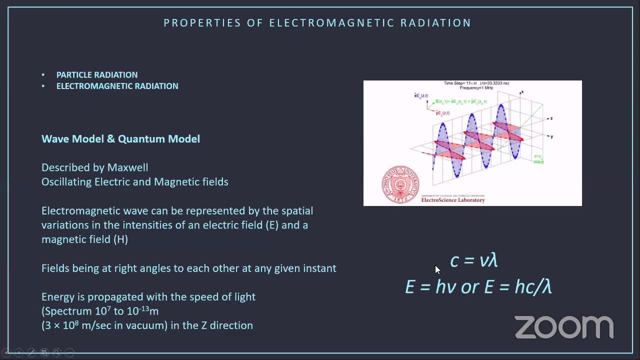 the power minus 13 meter. So the energy of the electromagnetic, that's this spectrum of 10 to the power minus 13 meter, from 1 to 8.. And the onghle rubber is that it can apresent the strength of the electromagnetic wave. So the energy of the electromagnetic wave is chant. 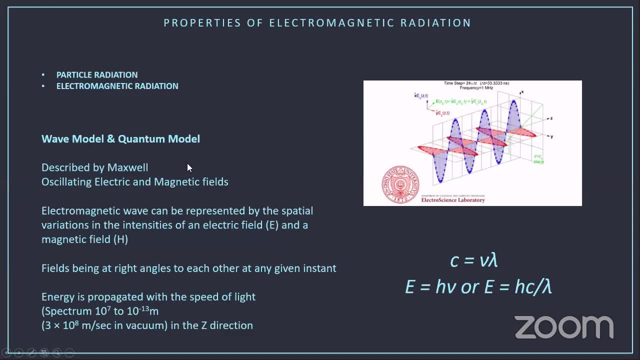 life is actually 1 to the power of one talk. I mean right. C is a constant right, So each wave is a constant momentum. So you know our def test: heightened magazines and extender posses the total energy of all the不要. 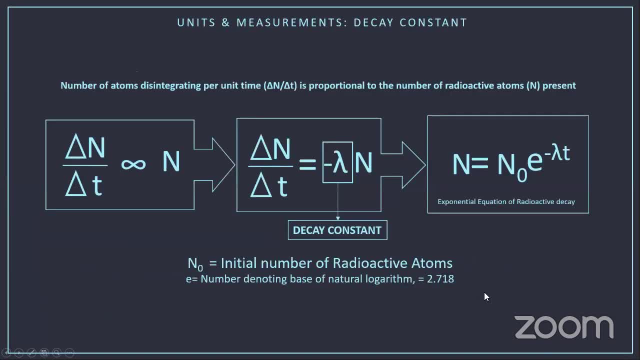 energy, or see is the velocity of light, Now coming to few other important units- and measurement for radioactivity. So what is Dicte constant? So it is seen that naturally the number of atoms that disintegrate per unit time, that is, the disintegration rate, is usually proportional to the 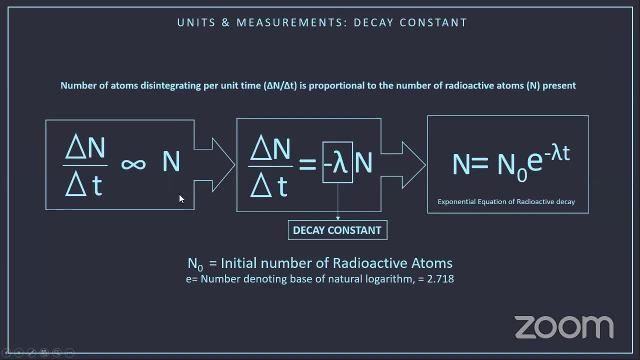 number of atom in which is present initially in the in a radioactive atom. So the disintegration rate is proportional to the initial number of atom present, So from which we can derive a constant, which is known as lambda or Dicte constant, which is denoted as negative because the number 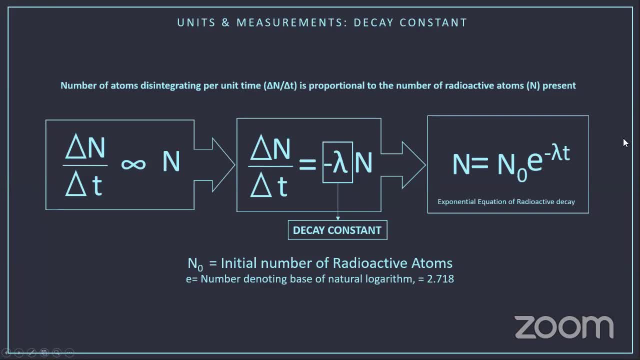 will decrease with time because of the decay. From here, by logarithmic expression, we can get this equation, where n is the number of atom present at a time of t and after a certain amount of decay, after the time of t and n0 being the initial number. 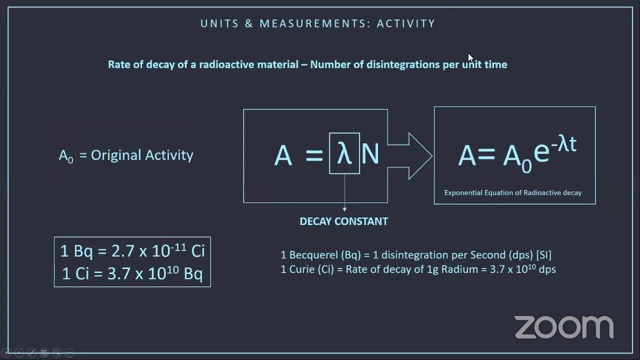 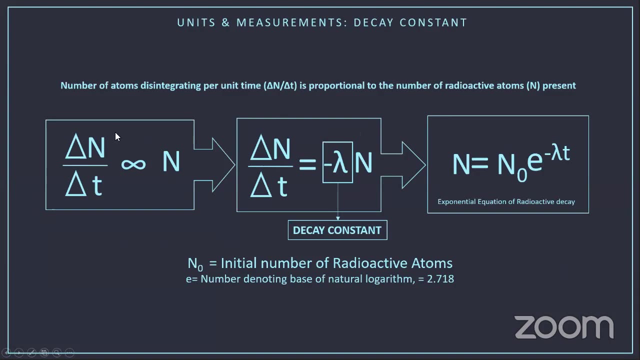 The same thing can be extrapolated in another equation of the activity. So activity is basically defined as it is: the rate of decay of a radioactive material, that is, the number of disintegrations per unit time or second. So if you see this model, the number of atom disintegrating per 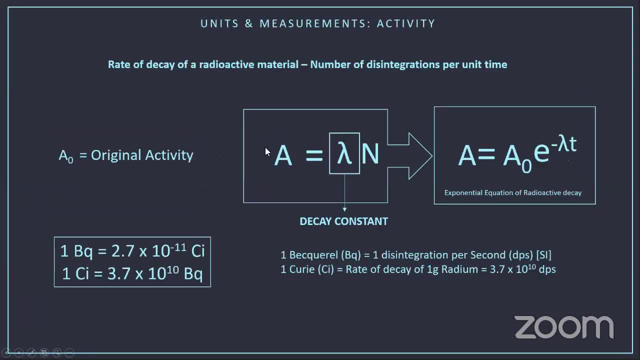 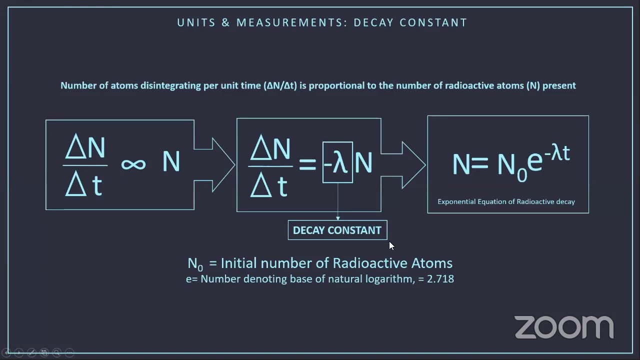 unit time is basically this dn by dt, which can be replaced by activity, and from here we can derive the similar equation for calculating activity also, where a0 is the primary activity. So the activity will decrease with time according to its decay constant, So the decay constant will vary. 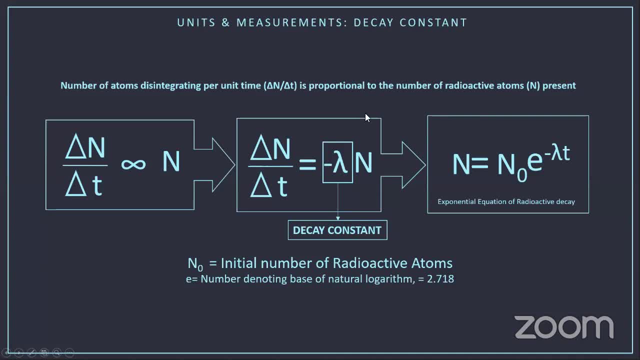 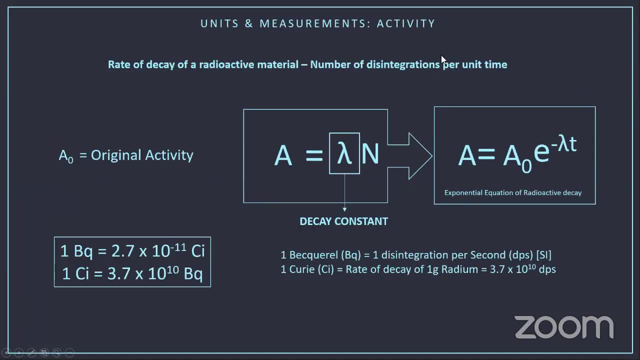 according to the element and for a particular radioactive atom, the decay constant will be specific. So according to that the half will be determined, which will be determined by the number of atom disintegration per unit time. So now we can get some totality. unit was given at that time. it was found that the radium's decay is 3.7 into 10 to the power, 10 dps. 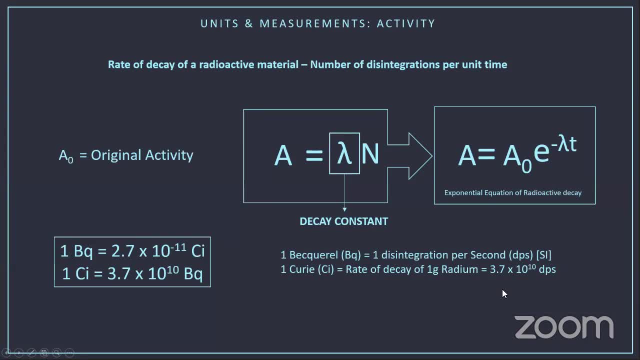 but later it was found that it is not actually 3.7 but it's around 3.66. but however, for the definition purpose, one curie is defined as 3.7 into 10, to the power, 10 dps and if you see the 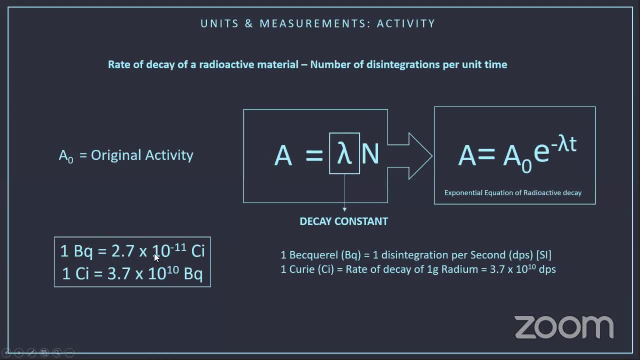 relation between becquerel and curie. the becquerel is usually 2.7 into 10 to the power minus 11 curie. one curie is equal to 3.7 into 10 to the power 10 becquerel, as it is equal to one disintegration per. 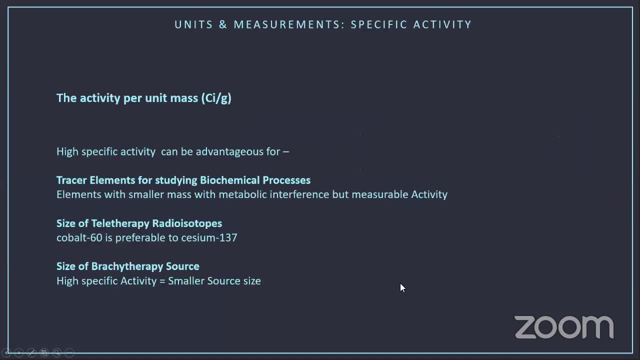 second now coming to some other properties of radioactive materials, that is specific activity. specific activity is basically the activity per unit mass. that means how much activity is there within a unit mass of a material. so you can see if the specific activity is high. that means a smaller amount of material can have more activity. 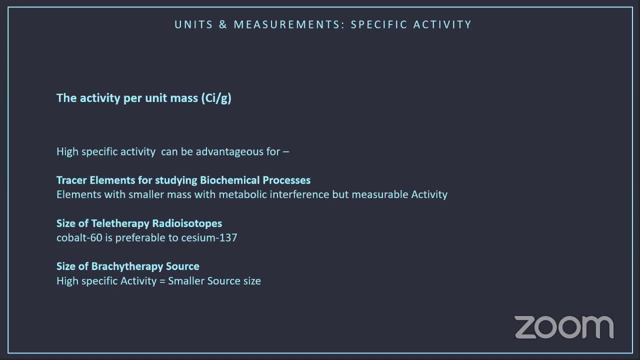 so this property is exploited in tracer elements for starting biochemical process, where a very small amount of radioactive material can be injected in the body which will not take care, take part in metabolic interference or cause metabolic interference because it is so small in amount, but will give some measurable activity, and for radiation oncology we use this specific 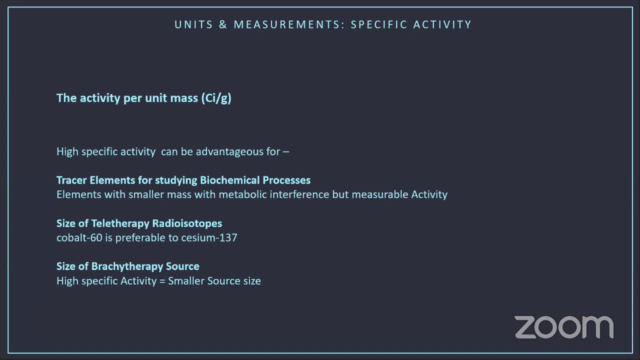 activity for to determine the size of teletherapy or brachytherapy sources. as you see, if you have a high specific activity, you can make smaller size of radioactive sources, which could be useful because the smaller size of radioactive teletherapy source can have smaller penumbra and 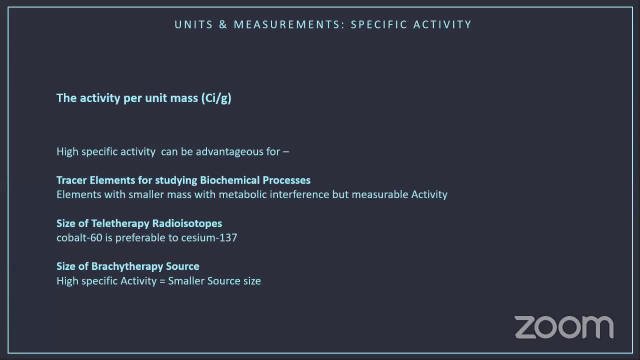 smaller size of brachytherapy source is easy to use and easy to be inserted in the body. so if you see the what are the ideal nature of a brachytherapy source, you will see high, specific, specific activity is one of the most important criteria. 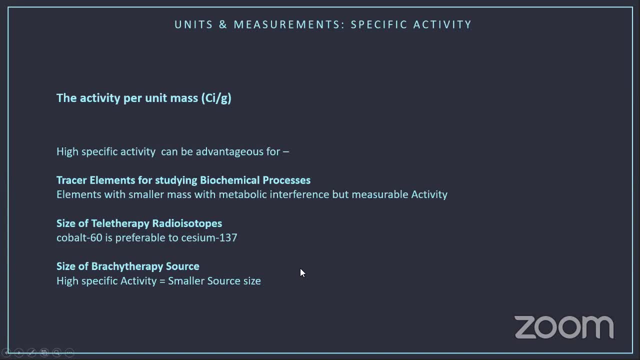 for an ideal brachytherapy source. so it can be explained that. why cobalt 60? despite having a half life of 5.26 years, in contrast to cesium with 130, 137 of 30 years of half life. why cobalt 60 is? 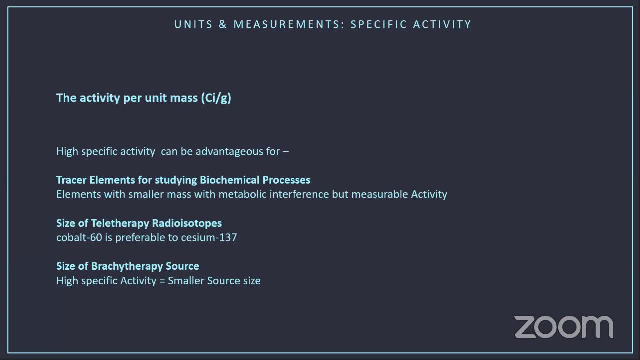 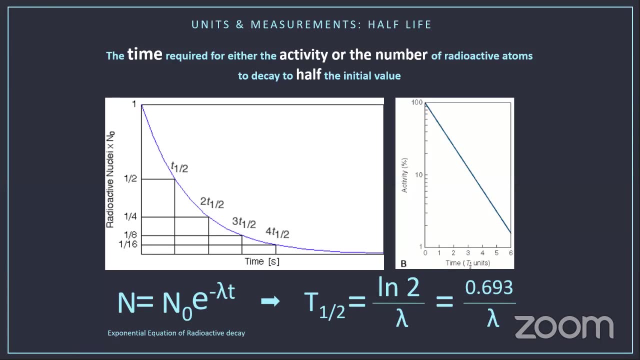 preferred over cesium, because the specific activity of cobalt is much more than the cesium. now coming to one of the most important phenomena, which is known as half life. so what is half life? so half life is basically a measurement of a time. it is a time required for something to become half. what to become half? it is the activity. 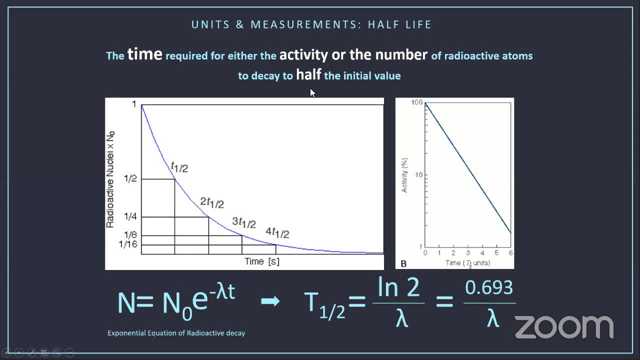 or the number of the radioactive atom to decay to its half of the initial value, so that it is the time required for either the activity or the number of radioactive atoms to decay to half of the initial value. this is known as half life. so let's see what is this. so if you see the 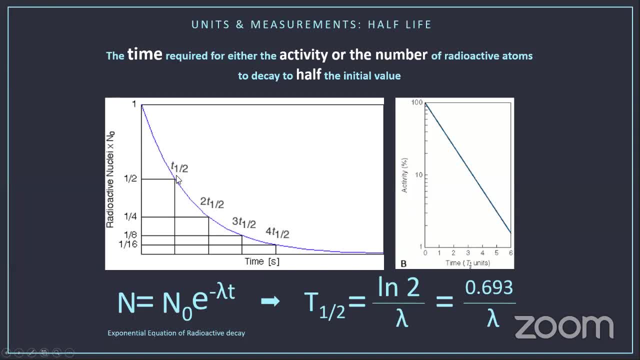 number of radioactive nuclei was one. so after certain time it will become 0.5 or half. then again, after certain time it will become 1, 4, then 1, 8, 1, 16. so it will decay in an exponential fashion. so it will never reach 0 because it is decaying in an exponential fashion. so that's, that is but. 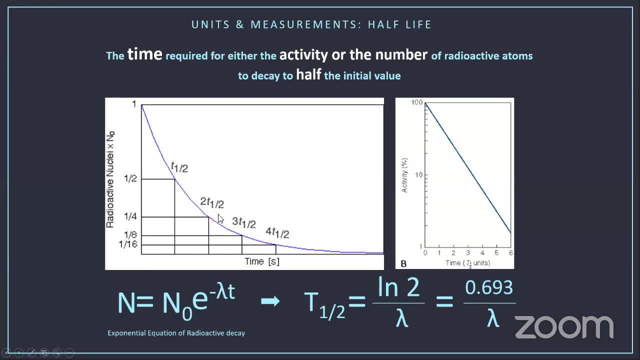 you can see the decay. this distance for each half is equal, so this is known as the half life, which is basically the time. so this curve for a mathematical expression can be represented in a semi-logarithmic curve with a straight line further calculation. so the calculation of half life is that. so we have this equation in mind. 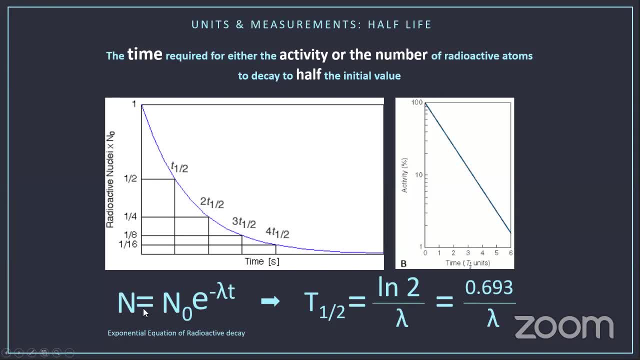 that n is the number of radioactive element at a certain time and which is equal to the initial elements, to the power. lambda is the decay constant and t is the at a given time. so if you see, if you want to make it half, so n by n? 0 will be half. so if the n by n? 0 is half, then you need to find. 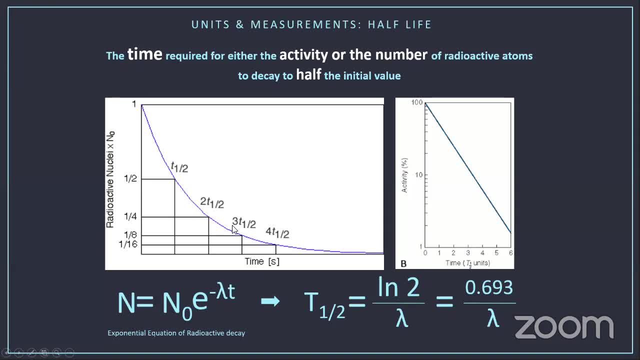 what is the time required to become n by n 0 to reach half life. so that's that's the calculation. half the value, so that is called as t half, is t is replaced by t half. then you see the it is basically 0.693 by lambda. so now i have already told you the lambda is the decay constant for a. 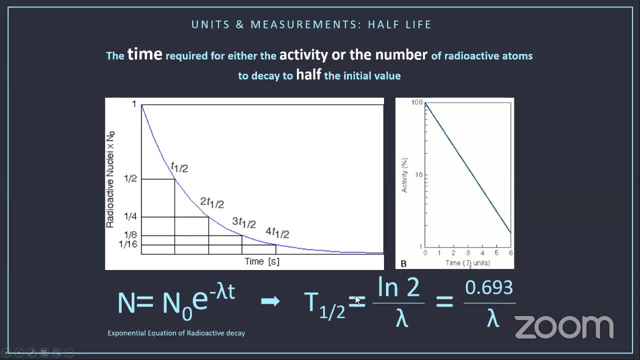 particular element. so for a particular element, t half will be fixed, as we have already told. for the cobalt 60 the t half is around 5.26 years and the for cesium it is around 30 years. so for a particular radioactive element, half life will be fixed. 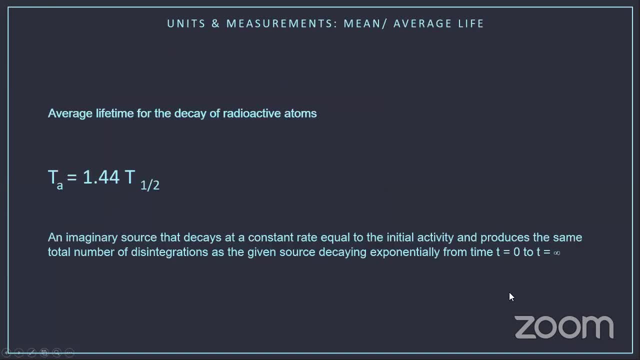 and that can be derived by this formula. so coming to one more thing which is known as mean or average life, it is particularly useful for some calculation. the average life means, suppose, the um source which is rather than decaying in the, rather than decaying in the like exponential pattern. so suppose it. 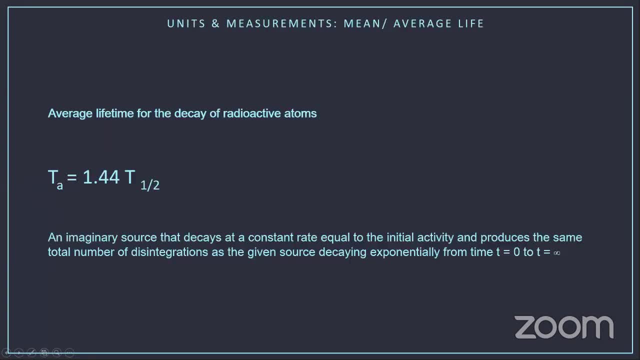 decays in a constant rate equal to the initial activity and use some, all the all, the lifespan or the decay. decay of the all radioactive elements, and you divide by the number of radioactive initial number of radioactive atoms present, So you get something which is known as the average lifetime. So it is. 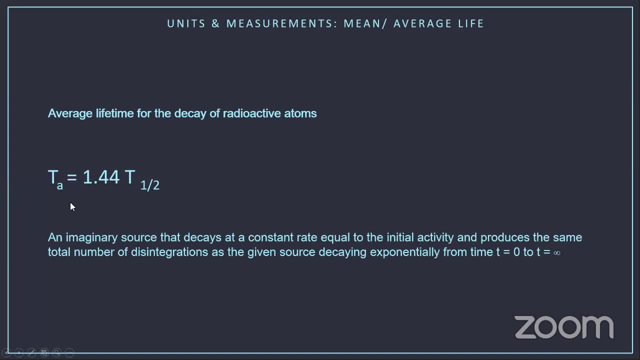 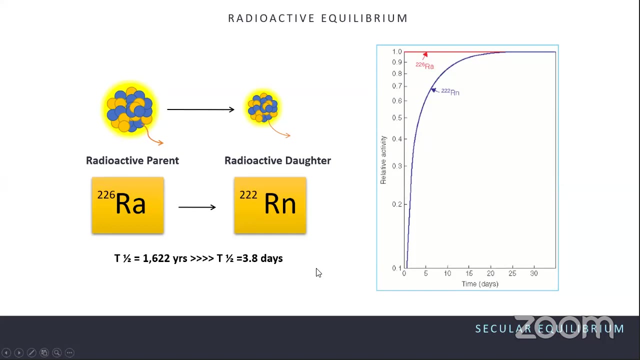 useful for some mathematical calculation and is also can be represented by the Greek letter tau. The t average is basically 1.44 of the into the half life, So by this you can calculate half life, the average life. Now coming to one more phenomenon, which is known as radioactive equilibrium. 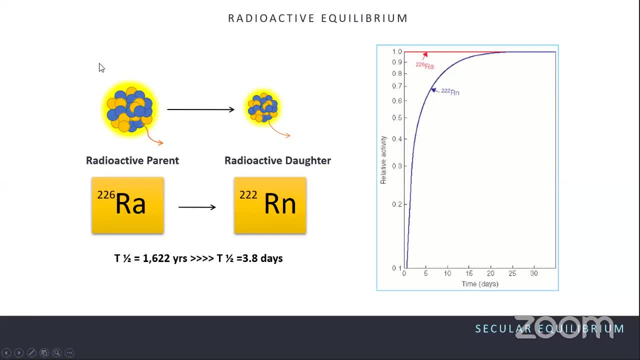 So this occurs when you have a radioactive material which disintegrates to form another material which is known as the daughter product, and the daughter product itself becomes a radioactive one. So suppose in here the radium gives rise to radon, and this radon is again a daughter product, but again radioactive. 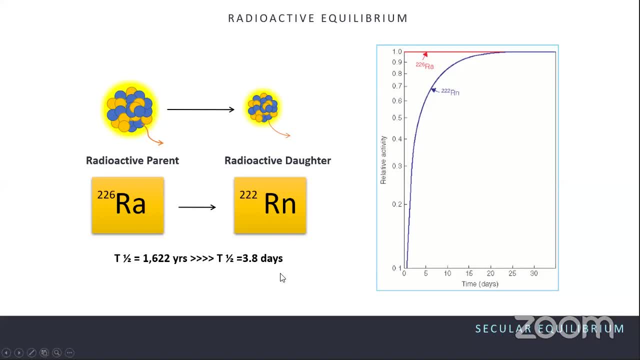 So when this kind of Raydon is again a daughter product, but again radioactive, So when this kind of RADON is again a daughter product, but again radioactive, situation occurs that the parent and daughter both are radioactive, the, both, the decay, both the decay or the activity of this, both isotopes becomes, the ratio of the activity becomes. 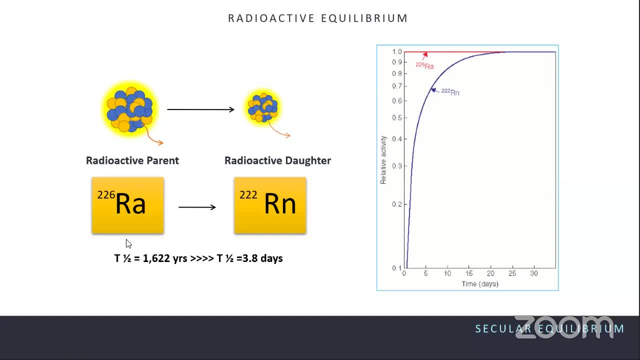 constant after a certain time. So like here, when- and that depends on the half-life of the parent and daughter molecule, daughter elements- If the half-life of the parent molecule is much, much more than the half-life of the radon, with the daughter molecule, as in the. 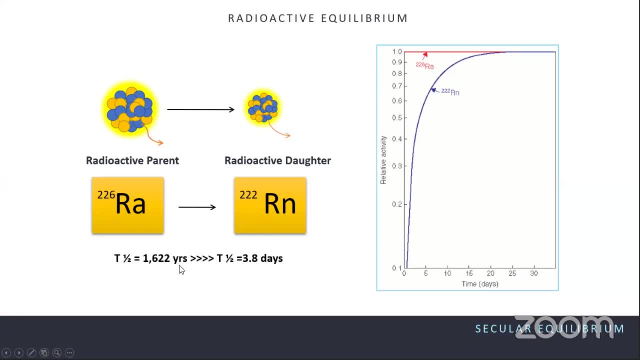 radon gas only 3.8, which is negligible to 1622 years of radium's half-life. it will reach an equilibrium with which is known as a secular equilibrium. That means the initially. initially, there will be no radon when the radium is there and the radio it will. 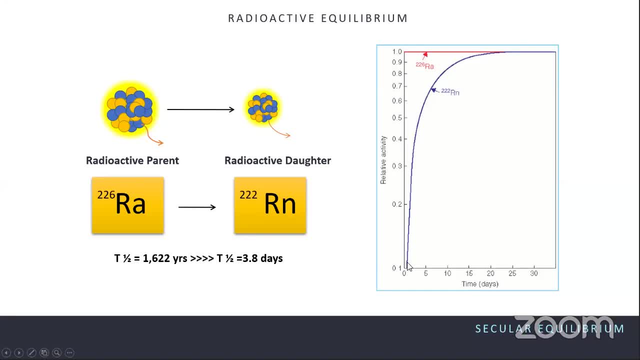 As the radium starts decaying to radon, the radon gets accumulated in the system and it will increase in number. But, as you see, the time to become a radon to radium is much better than to radium to radon is much longer because of the high half-life after starting around. 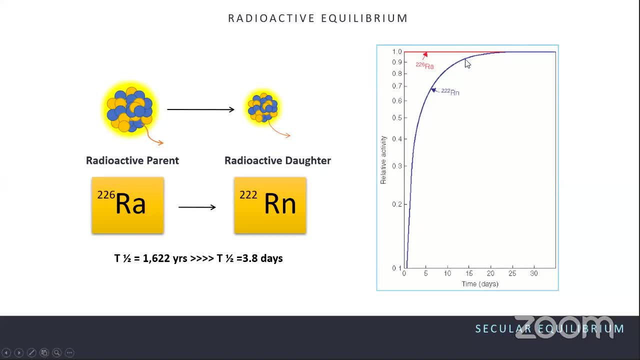 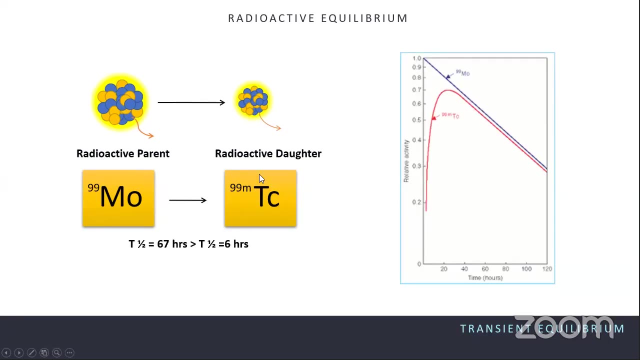 seven half-lives the radon, the amount of radon in the system, and the activity will become almost equal. equal, the activity will come into equal when, And they will reach an equilibrium. This is known as secular equilibrium. While, if the similar thing occurs, but with a smaller half-life, for the parent parent element, where the half-life 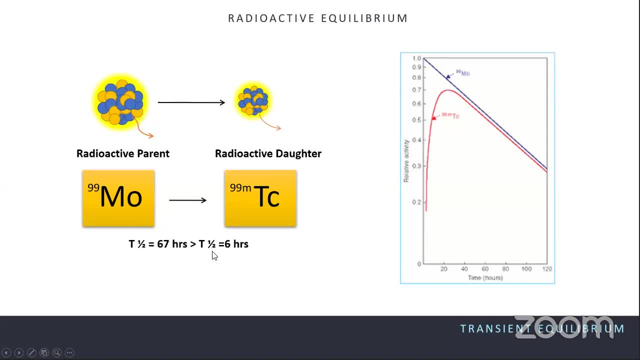 of the parent element is not that small, the more- not that long- than the daughter element, the equilibrium achieved is different. That is a classical example of this transient equilibrium where the molybdenum, Which is Used to create this metastable technetium which is used in different medical application. 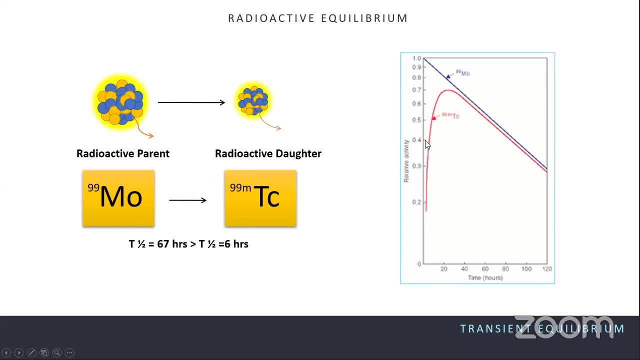 the. once the system starts generating molybdenum quickly, it reaches the equilibrium and they reach the ratio of a constant ratio of the parent and daughter activity, and these reaches by usually four half-lives. and this system is also known as the cow, like every time, 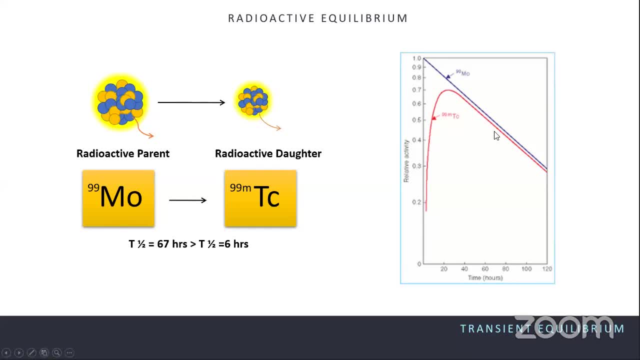 the technetium is generated from the molybdenum and some amount of My technician is always generated and can be taken out of the system or the purpose of medical As making of the call for the purpose of medical Experiments or interventions. 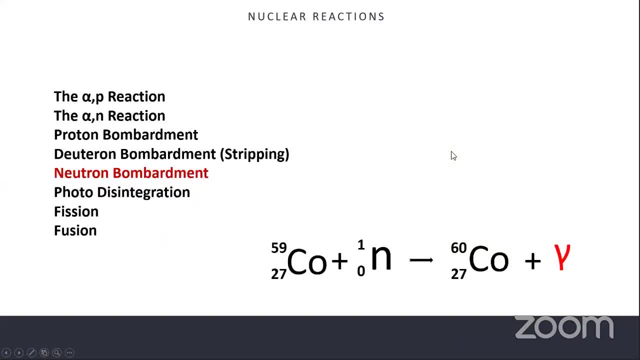 The last week come to the nuclear reactions will not go into any details on nuclear reaction. we are not different types of nuclear reaction and basically nuclear reactions or the reaction between the particles, protons or neutrons, with the nucleus and they form different types of change in the elements. 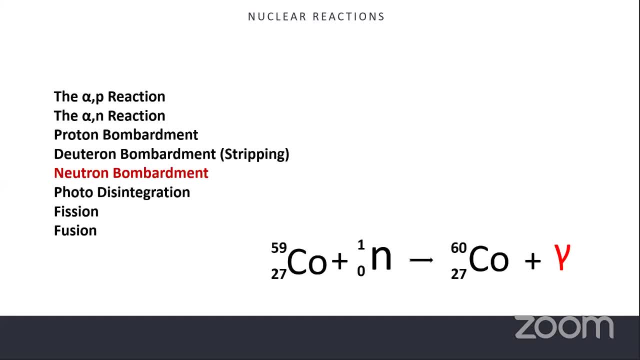 and different types of energy emission. I will come to one or two of them, specifically the neutron bombardment, which is very commonly used for generation of radioactive nuclides or isotopes, which we commonly use in our radiation oncology practice. Most of the artificial isotopes are prepared by neutron bombardment, which does not change. 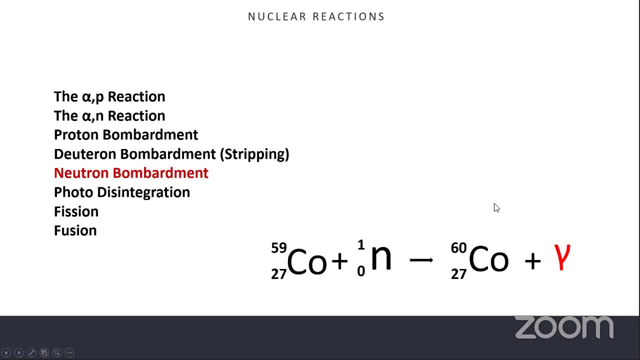 the element, but changes the atomic number and makes them radioactive in a reactor which will later cause decay by radioactive decay of beta particle decay and gamma ray emission. Now another thing is the fission reaction, Which is basically sometimes called a spontaneous fission or fission by neutron, or especially 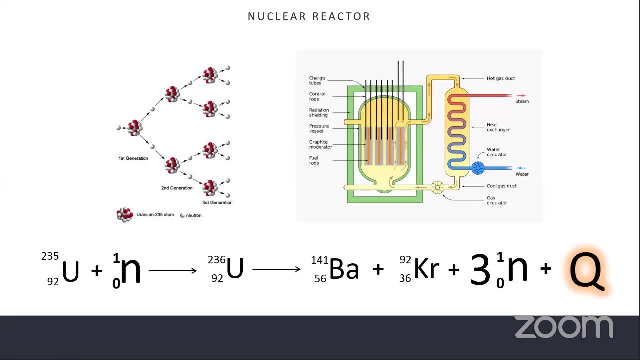 the thermal or the slow neutrons, which are very efficient for this fission reaction. when a particular element like uranium is bombarded with thermal or slow neutron, it will generate, or initially generate, an element which will spontaneously break into few other elements and will give rise to few more fast neutrons also. 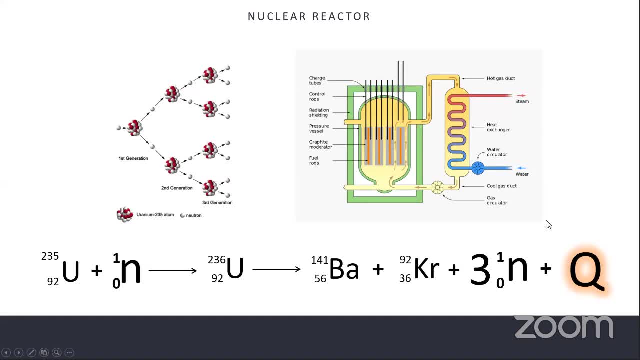 And this fission reaction will release massive amount of energy. And this fission reaction is also a form of decay. it is somewhere it is also classified as a type of decay- where a particular element is spontaneously broken into some smaller elements and gives rise to enormous amount of energy. 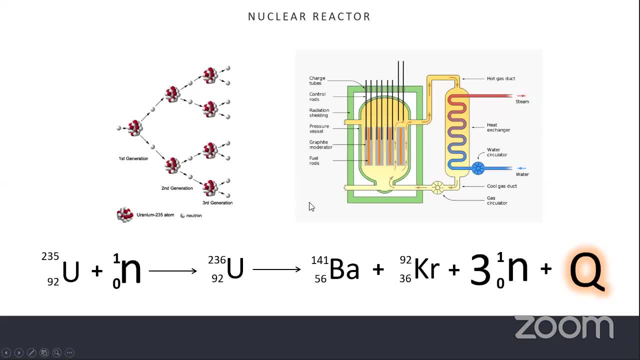 And this particular idea is exploited in the nuclear reactors to produce huge amount of energy for use of nuclear reactors. So what happens in the nuclear reactor? the- basically the neutron- first bombards one uranium molecule, which is basically the fuel which is inside the nuclear reactor and which gives 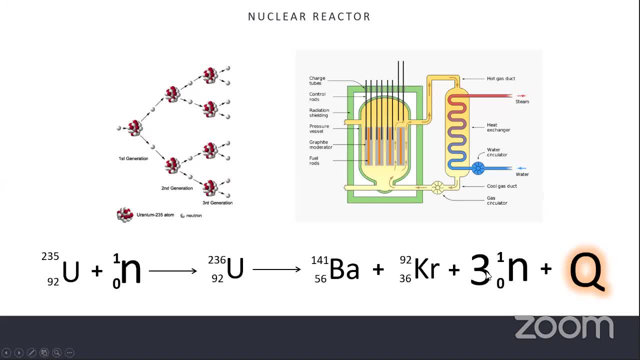 rise to subsequent energy release and some other fast neutrons which will again bombard some other uranium and thus initiate a chain reaction when a sufficient amount of uranium is present in the nuclear reactor. So in this particular case, if we look at the nuclear reactor and we have the source, 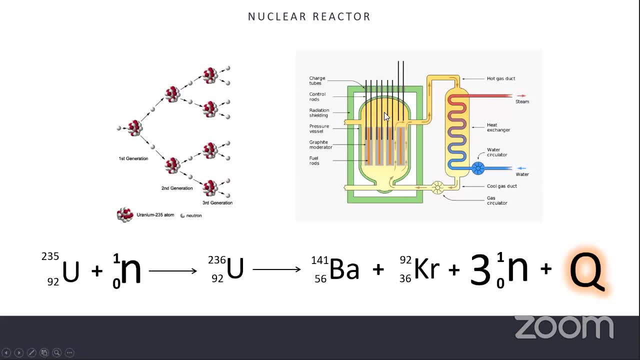 in the system, and these neutrons are sometimes very fast, and they are converted into slow neutrons by some moderators, like graphite heavy water, so that they become slow and they can again interact with the uranium, and thus the power generated can be used for some other. 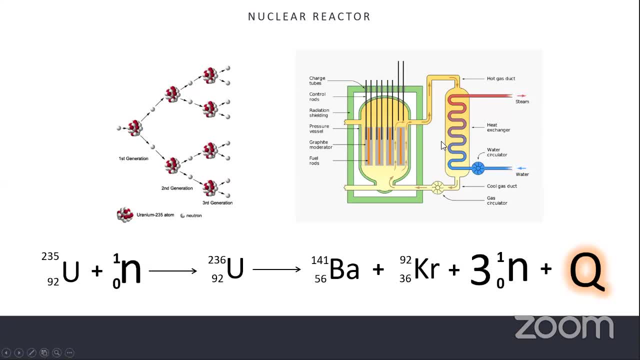 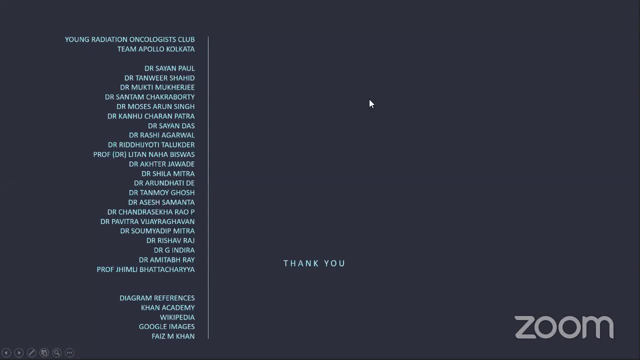 purposes. So with that I would like to conclude our first class on atomic structure and nuclear activity. I would like to conclude our first class on atomic structure and nuclear activity. like to thank the Young Radiation Oncologist Club for giving the opportunity and my team. 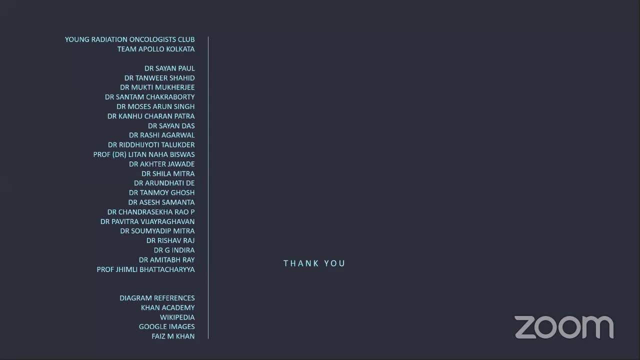 Apollo Kolkata, Dr Sayan Pal, Dr Tanvi Shahi, Dr Mukti Mukherjee, Dr Shantam Chakraborty, Dr Moses Arun Singh, Dr Tanu Charan Patro, Dr Sayan Das, Dr Rashi Agarwal and Dr. 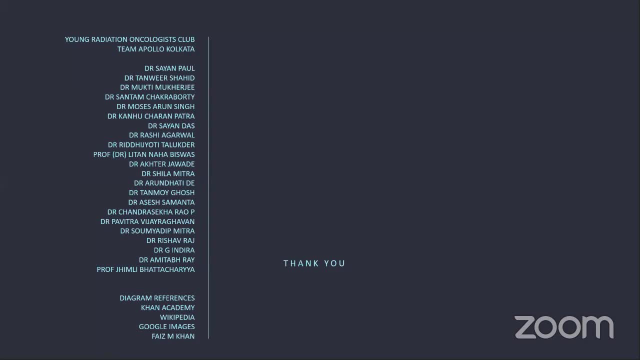 Hrithvi Jyoti Taluk there, who has given enormous time to create the Zoom platform as well as the YouTube platform so that we can simultaneously play in both the platforms over past two days, And I would also like to thank our departmental, my seniors and colleagues. 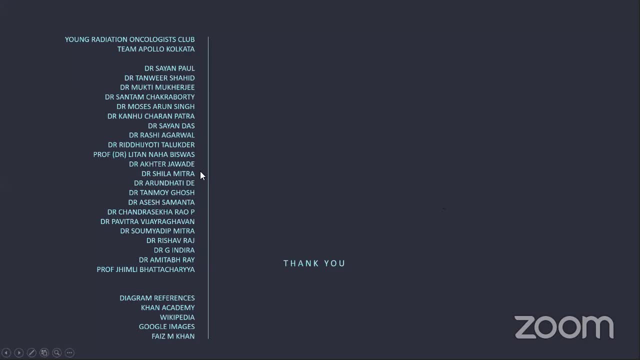 for giving their feedback during the presentation, my teacher and my cousin sister, who is a professor of chemistry, who also guided for this presentation, And thank you, Thank you very much. Thank you, Dr Givhar. It was an excellent class, I must say Very, very, very very. 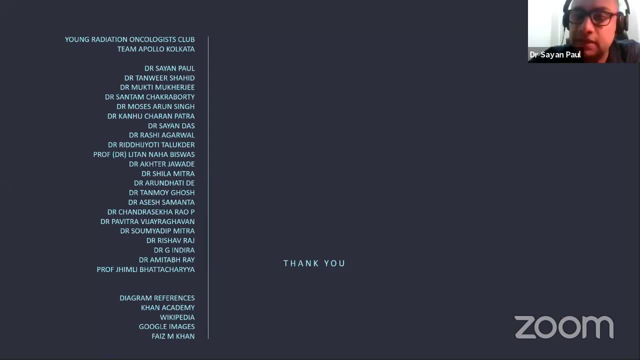 interesting And I hope the students will be benefited, Like this class. We have a few questions for each section, Okay, So if you want me to read it out, or if you can read this, you can answer these questions. Okay, Give me one minute. 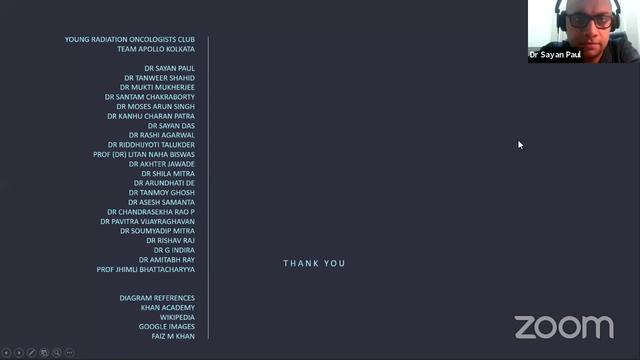 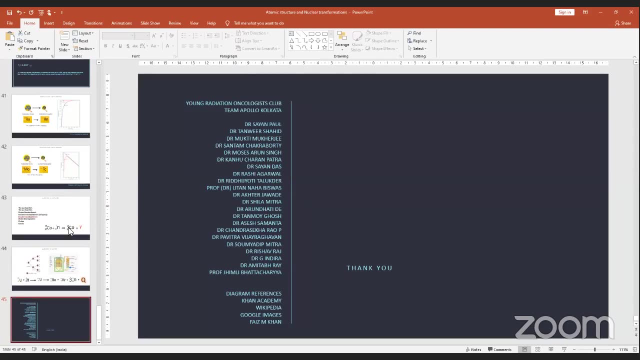 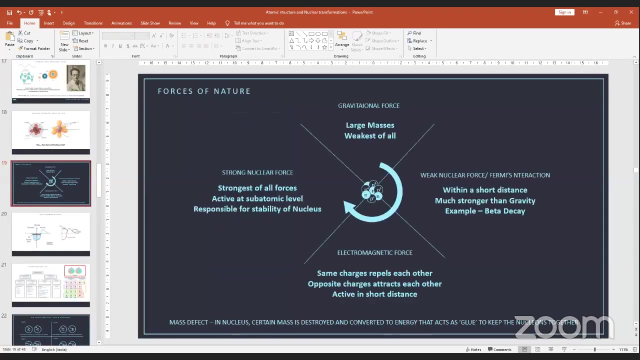 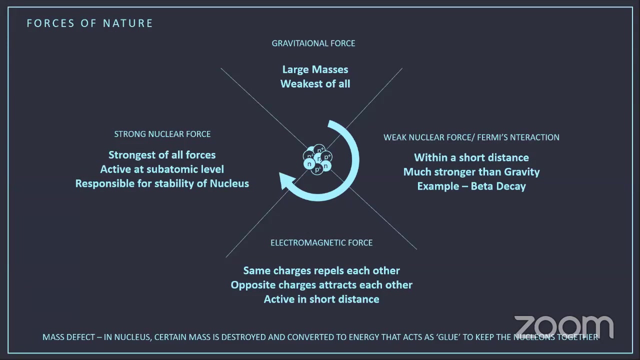 First one was: please explain nuclear forces and energy graph by Dr Tikla Curry. Okay So I'll go to the slide. Okay so, as we discussed that we have four forces in nature and I will not go into the gravitational force, so you wanted to know about the nuclear forces. 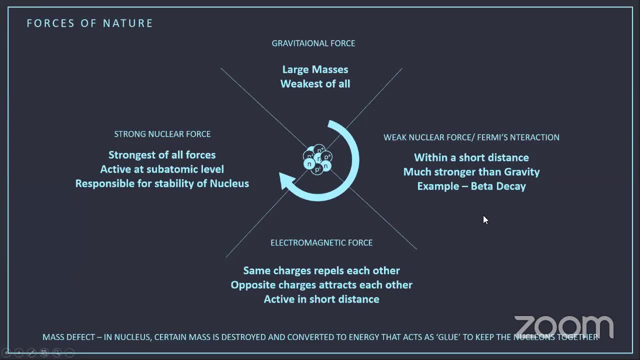 So in the nucleus, which is a very- I mean a very short subatomic which you can use a microscopic thing, rather in a very short distance, gravitational force does not work. So gravitational force is not some force which can work in the nucleus. So mainly these three forces act in the nucleus. 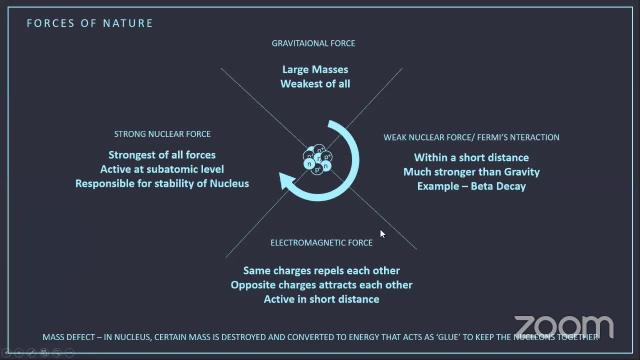 So, coming to the most easy one, this is the electromagnetic force, which we all know that the same charge- sorry for the grammatical mistake- the same charges repel each other. the negative charges will repel and the opposite charge will attract. So this is happening in the nucleus. it is easy to understand. 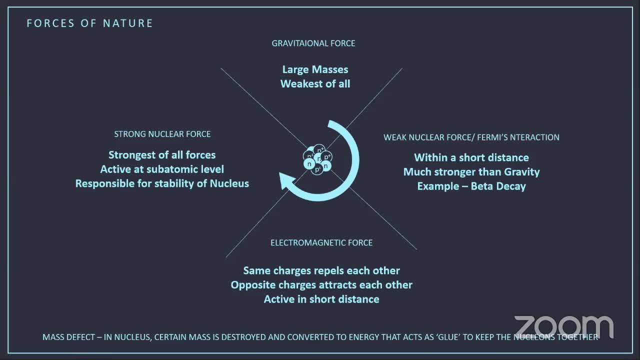 So when an electron comes towards a proton, it will attract, And if two protons come towards a proton, it will attract, And if two protons come towards each other it can repel. And it can be explained that when we are talking about the radioactivity, when the proton number, 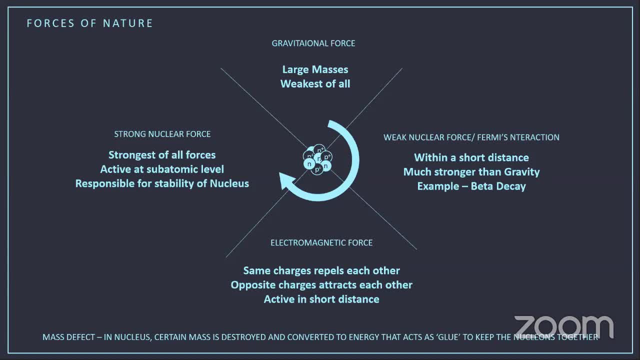 is very high in a particular system or a particular nucleus, you can think that the diameter of nucleus will increase And as the diameter of nuclear increases the distance between the two proton will increase. As the distance between the two proton increases it will go beyond the strong nuclear force. 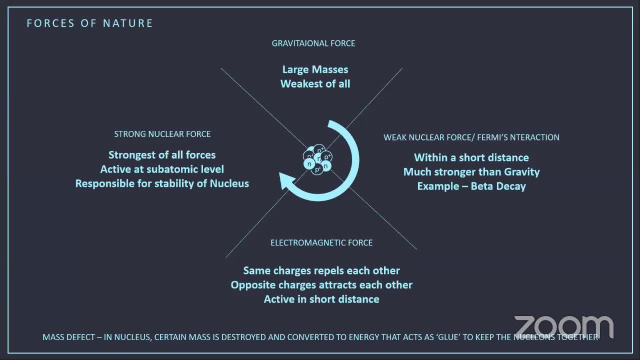 As soon as it goes beyond the strong nuclear force. it will go beyond the strong nuclear force, the electromagnetic force will act and they will repel each other, So they will try to go away from the nucleus. By that you can basically explain how the proton wants to go out or wants to decay by 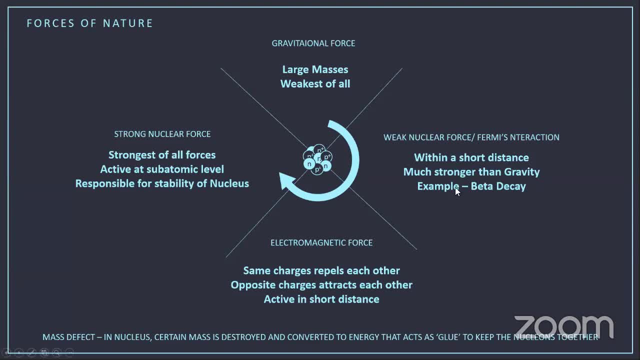 beta positive decay. That is one thing. Now, coming to weak nuclear force, the weak nuclear force is actually also known as the interaction. Basically, it is not said about force, rather it is described as an interaction. It is an interaction which was given by Enrico Fermi. 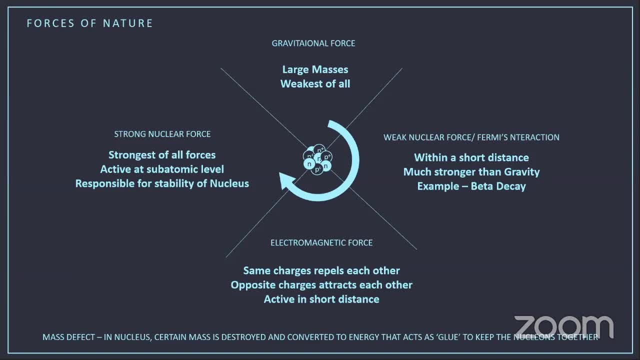 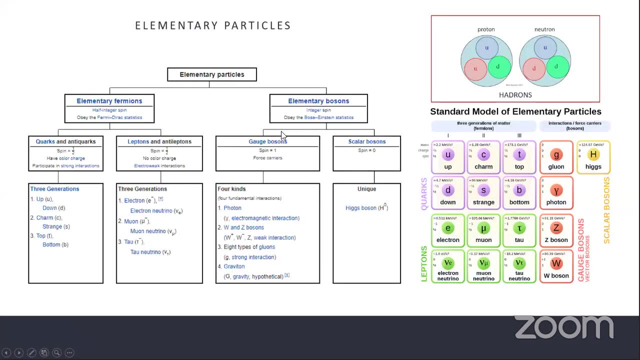 So it also acts in a very short distance, maybe at a distance of the size of a proton, and it is stronger than gravity. And if you see the elementary particle, you can see the bosons which are basically known as, which is a type of elementary particles, with this W, W and Z. these are the bosons. 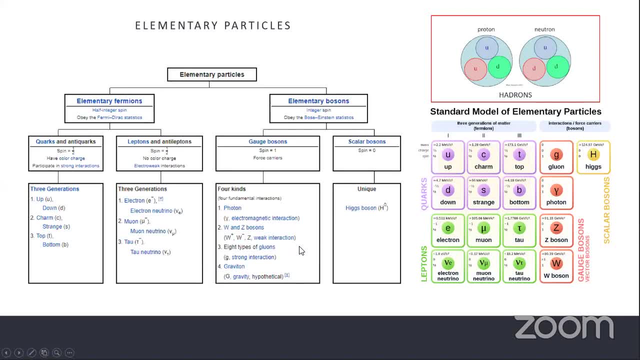 or the elementary particles which have some force fields And they basically act in a very short distance. So they basically are responsible for this kind of interaction. So by this interchange of these force field molecules, the proton and neutron can change with each other. 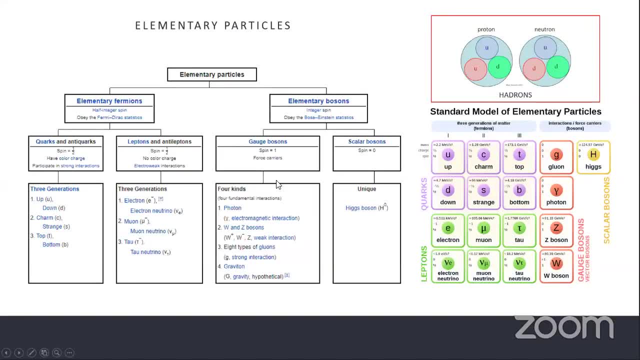 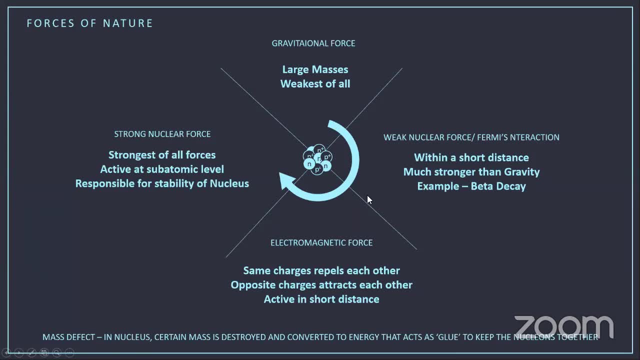 And so that, as we have seen in the beta particle decay. so these interactions are basically guided by the weak nuclear force or Fermi's interaction. Now, coming to the strong nuclear force which you were asking about, the strong nuclear force is something which binds the proton. 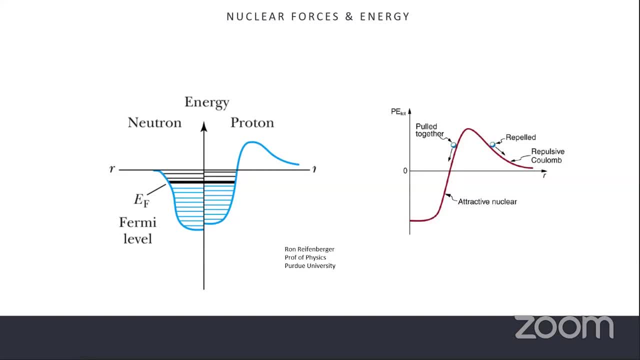 Even they are positively charged, the strong nuclear force can bind them. So there must be something unique. So that is in a very short radius. the strong nuclear is so active that the protons can actually ignore their repulsive force and they can become together. 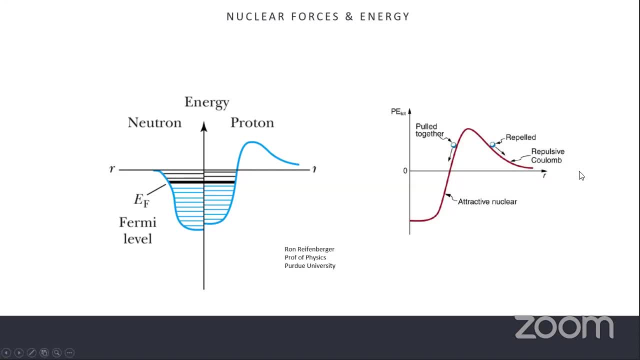 So if you take a proton, which is a positively charged, from an infinite distance towards the atom, So initially it will feel the repulsive force And then it will act in a very short distance. So the proton can be a repulsive force because of the positive charge of the nucleus. 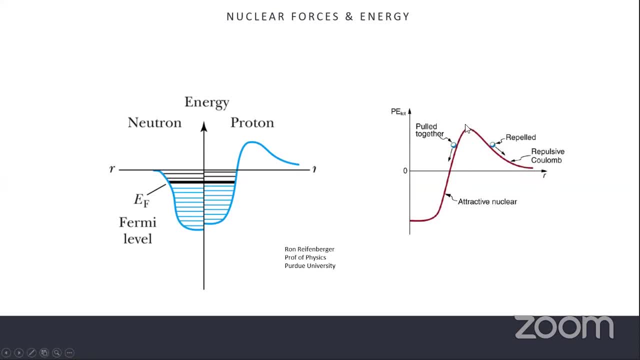 But somehow it has got enough energy to cross the maximum repulsive force, which is known as the potential barrier. Then it will come into the field of the strong nuclear force and it will be a part of nucleus. I hope I could explain that. 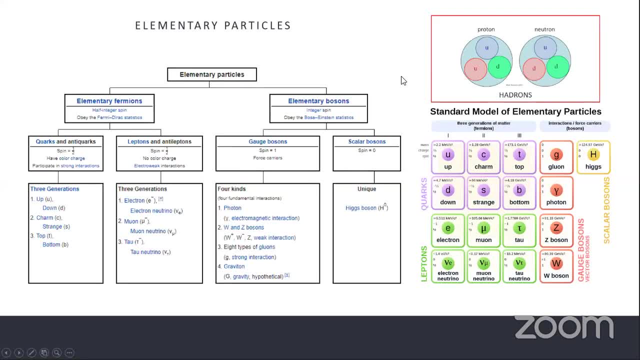 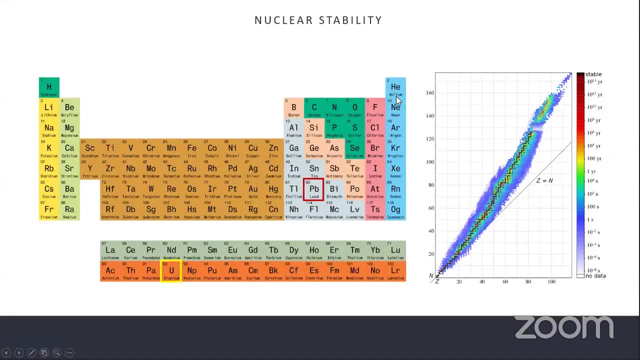 Dr Jeebar. So now the second question is: Kovalsky, Yes. So the first question is: why does the 60F2 energy, why it is called mono energetic? And third one is: what is the use of average half-life? 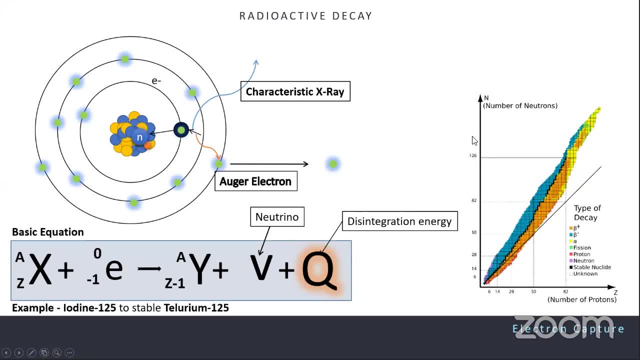 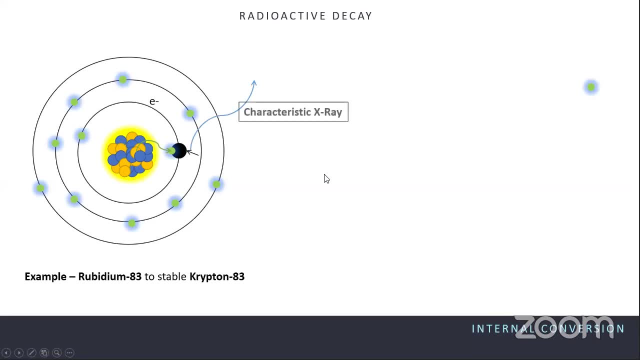 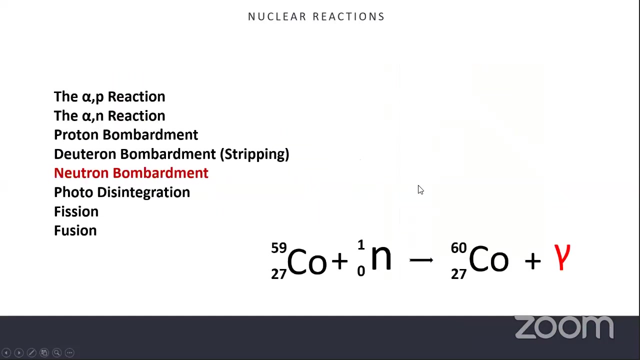 Okay. So first thing is that the average half-life is basically something used for calculation of quick calculation of some amount of radioactive material in some system. And now coming to the first question, that is why it is called mono energetic. Basically, the mono energetic and poly energetic beam concept comes from X-ray versus the nuclear. 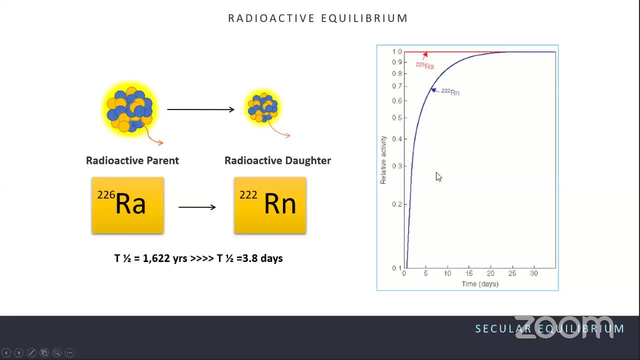 energy right. So in X-ray, if you see in when X-ray is generated, the X-ray ranges from zero to the maximum energy produces and that is producible And that is depending on the amount of potential difference you give for the generation of. 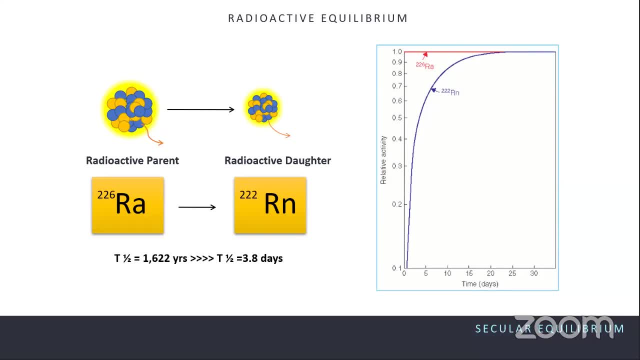 the X-ray in the cathode tube. So the more energy is generated, the more energy is produced. So the more the potential energy you give, the more the range of spectrum of energy will find for the X-ray. So it will range from it is. you cannot just count it. 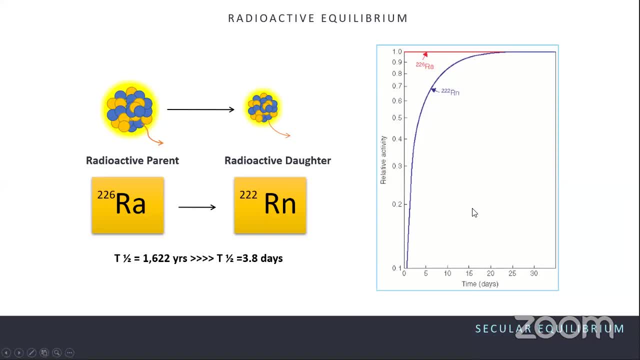 So that's why it is called a poly energetic While. so you cannot particularly identify one energy of the X-ray beam. So what you do, you take as a rule of thumb: you take one third of the maximum energy as an energy of the X-ray. 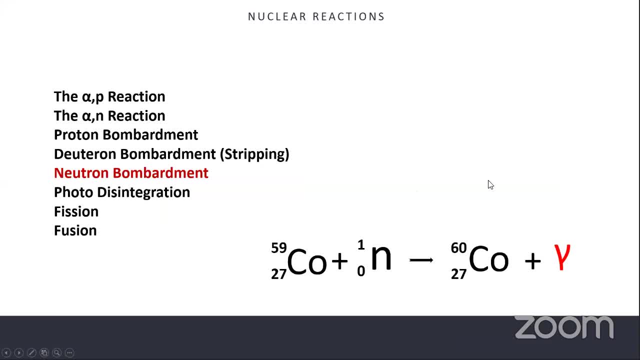 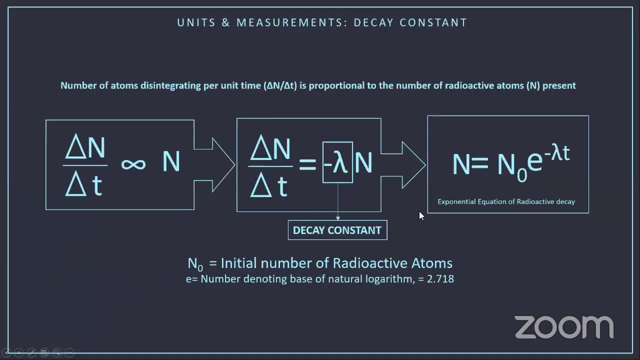 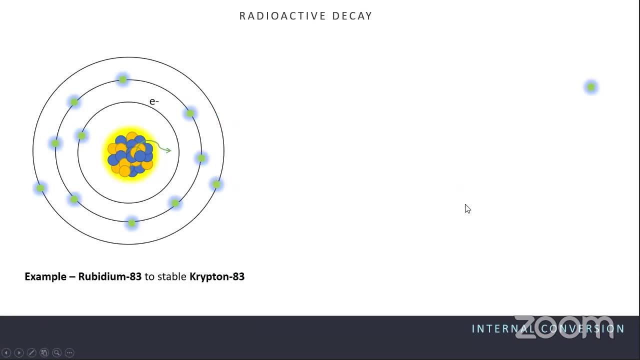 But for cobalt, though, it has got two energies liberating simultaneously, but you can actually identify the energies, the basically you can identify the energy, that is, it is finite. So that's why these are called mono energetic beams. But if you go to X-ray you cannot identify a one particular energy. 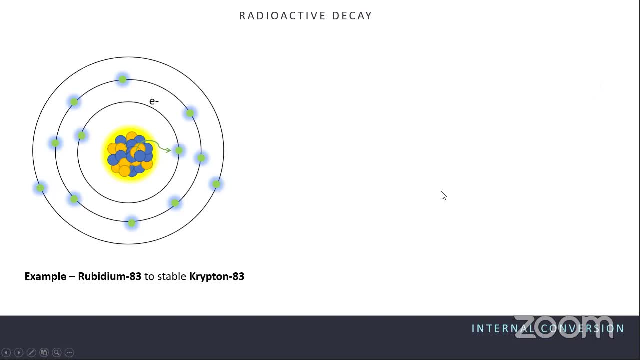 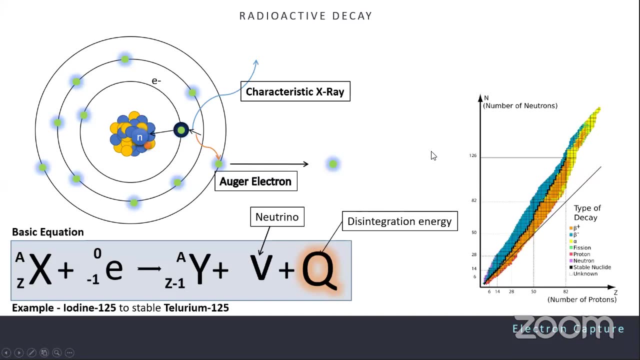 It is a spectrum, basically, Okay. The other question is: what is the difference between potential energy and binding energy? Okay, So potential energy and binding energy? the binding energy is nothing but the energy by which the electron is bound in the atom. So it is basically. it is usually the. if you go to the Bohr model, it is explained. 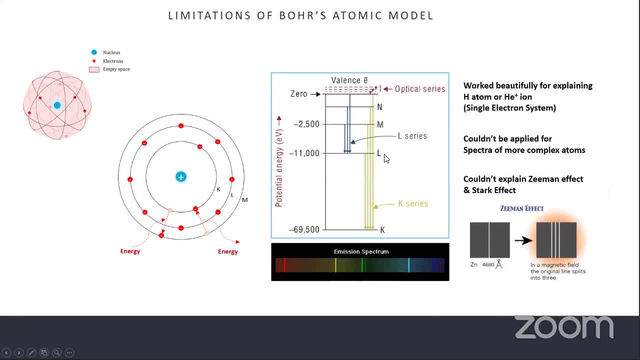 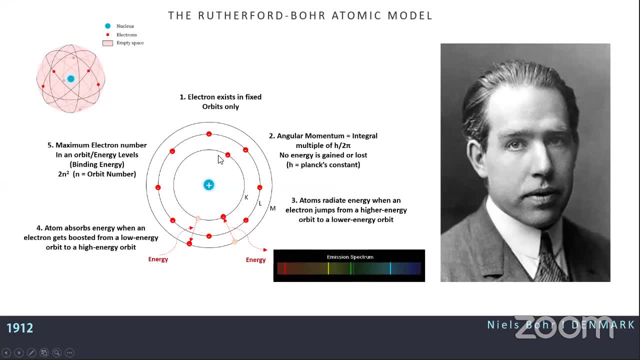 by. give me a time. okay, so it is. if I see the angular momentum, so if you see something that is rotating in a circular fashion, we know there will be something called a centrifugal force. So it will come, it will try to go out of the orbit because of the centrifugal force. 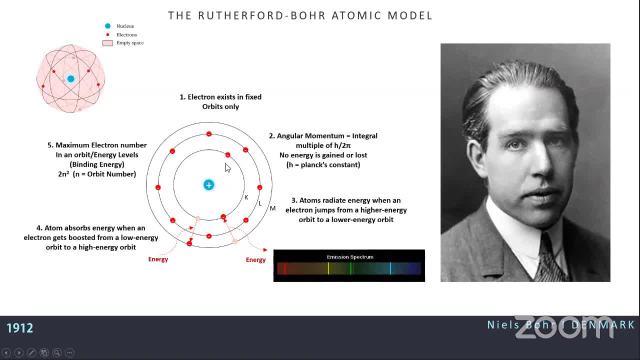 And on the other hand it has got something, the electrostatic force. So they will neutralize each other so that it can remain in the same orbit. And these forces can be explained by the angular momentum, which is the integral multiple of the h by 2 pi, which is basically given by the Planck's constant. 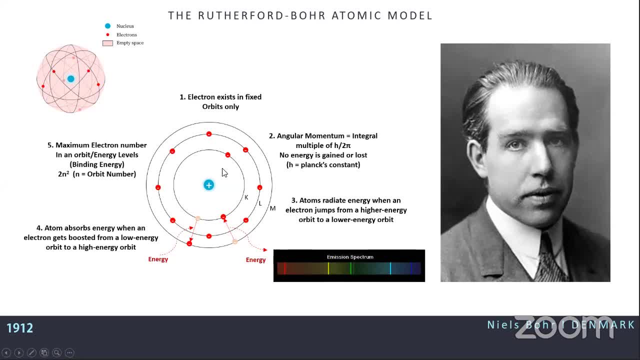 Okay, So this is the angular momentum. Okay, So this is called the binding energy. That means which is the energy specific to this particular shell of the orbit of the electron, And for each orbit it is different. So that's why, when one electron jumps from one orbit to another orbit, it will release. 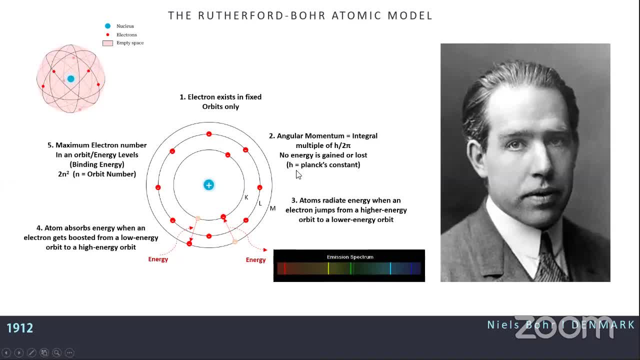 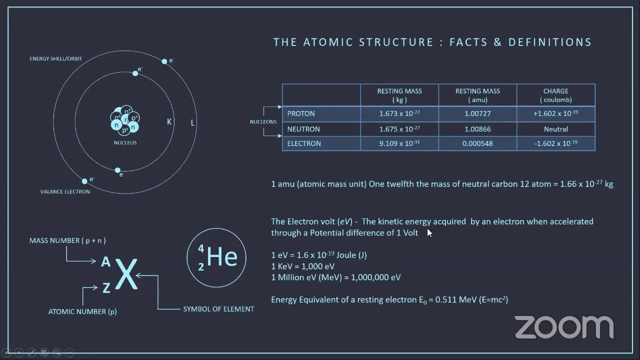 an exact amount of energy, which can be explained by the h nu 1 minus h nu 2, according to the orbit. Okay, So this is the potential energy. It is basically. if you go to the here you can see the. it is basically the when you. 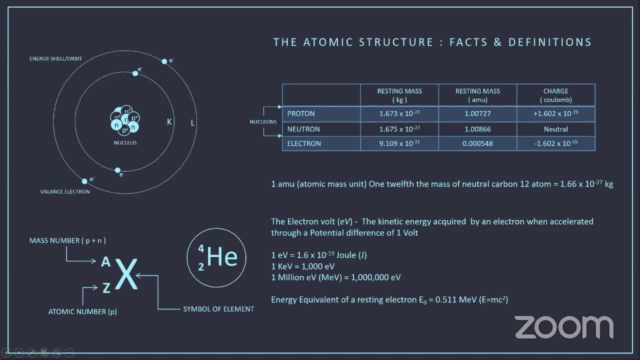 have an energy, which is, which is a kinetic energy. anywhere when the charge particle is within a field of electricity and given within the potential difference, it will gain some energy, And that is known as the. that is what is the electron volt, or the kinetic energy. 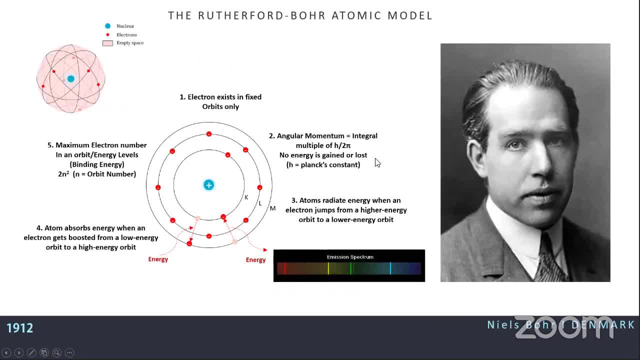 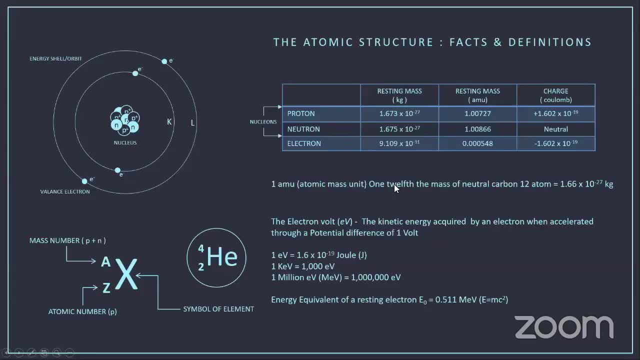 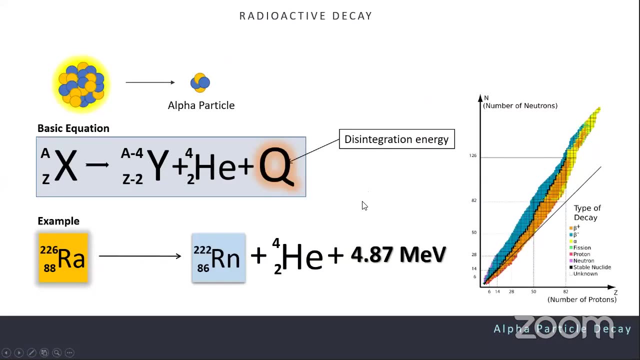 Okay. So the next question is, sir, can you please explain the potential? well again, I've just explained it. Yeah, Please explain megatron and positron emission again, Okay, Okay. So negatron and positron emission, So basically where the negatron will happen. 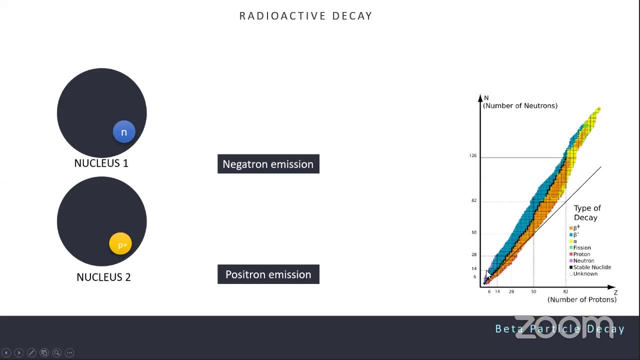 So basically, you know, this is this line of stability. So here you have more neutron, Here you have more Proton, So protons are positively charged, So they will want to expel positive charge and become neutral. So if you want to expel positive charge or emit positive charge, it must be something. 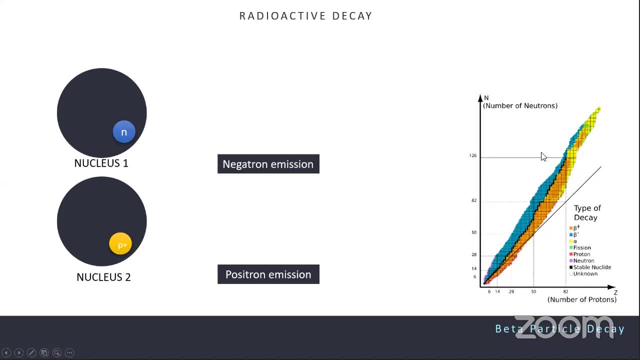 positive. So here you see positron emission, and for the upper part, the blue one, where the there is more neutral, they will want to have more proton, to get close to the NP ratio of one. So to get more proton they needs to get rid of the negative charges. 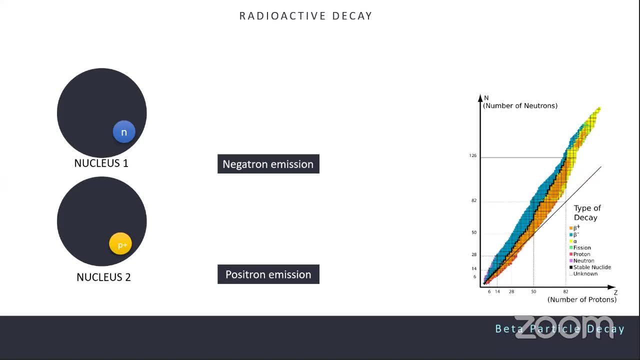 Right. So if you get rid of negative charges, you will get positive charge. So that is that is why this will. one neutron will be converted to one proton, plus one negatron and one anti neutrino, and these negatron will be expelled out of the nucleus. 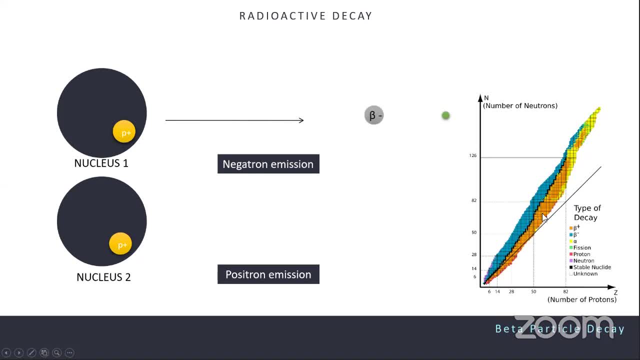 And so this is known as negatron decay, And in in here the positron decay. one proton will change into one neutron, Okay, Okay. So one neutron plus one beta positive or positron, and it will with a neutrino which has got. 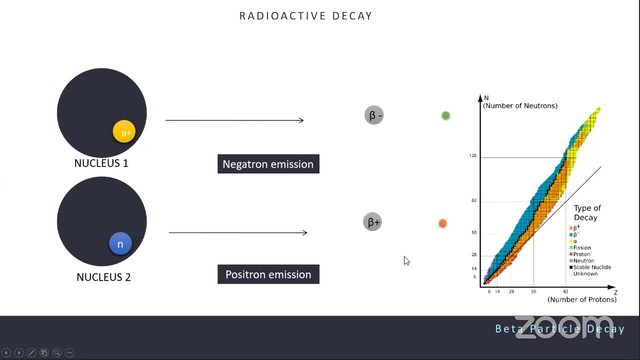 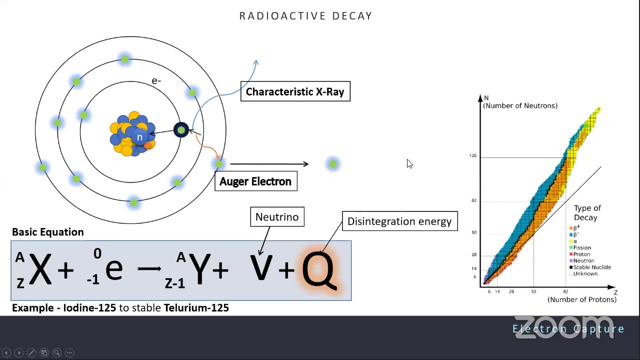 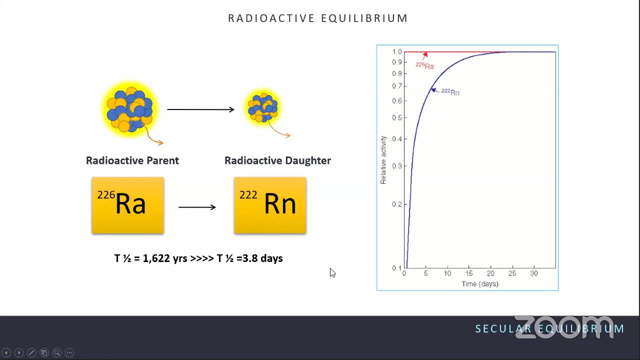 negligible mass and will come out as positron decay. Okay, So the other one is: can we explain the slide showing radium and radon, half-life and equilibrium? Okay, This one right. So the equilibrium is something. it is applicable only when the parent and daughter both are. 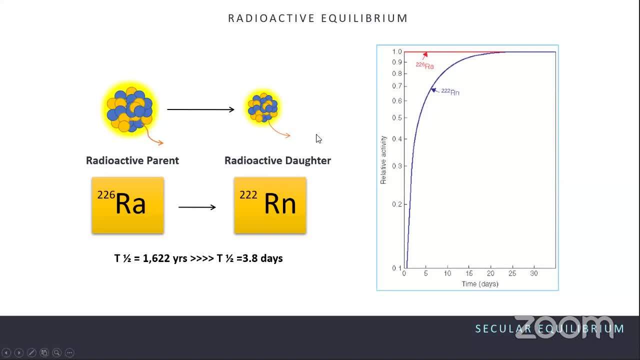 radioactive. Okay, It is not applicable when the daughter is not radioactive or the daughter is removed from the system. So both of them had to be radioactive and both of them have to be in the same system- rather I will say a closed system- to achieve a equilibrium. 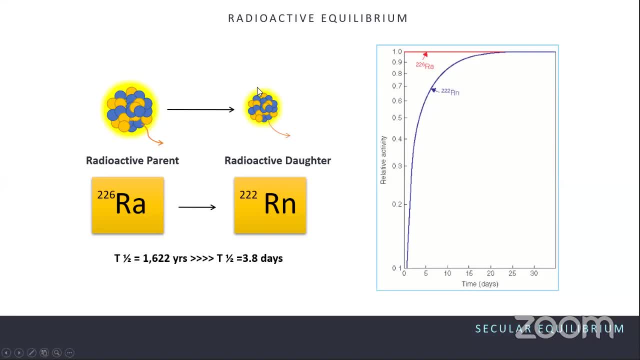 Equilibrium means the activity of the parent and activity of the daughter will become. the ratio of these two activity will become constant after a certain time. This is equilibrium. Equilibrium means the activity of the both parent and daughter will become constant after a certain time. 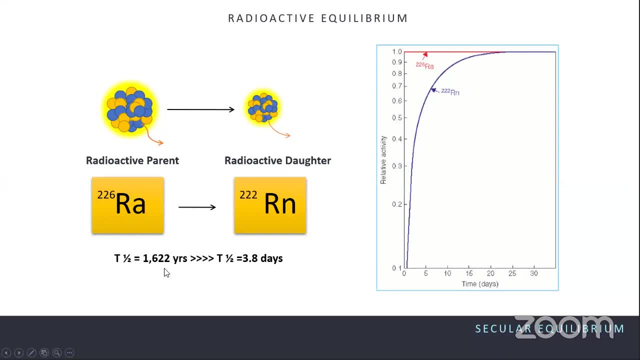 Now, if you see the half-life of radium, that is almost 600, 1600 years, and the radon is only 3.8 days. So that means the radon which is produced from the radium will be decaying again. 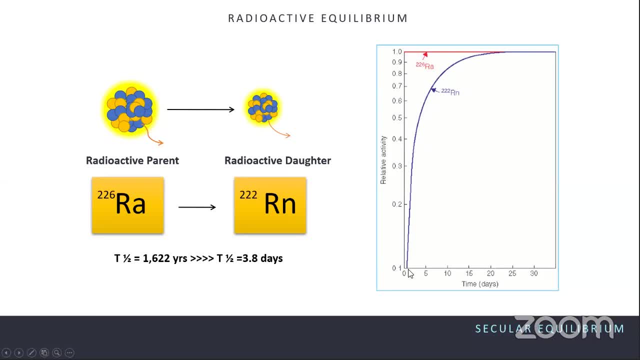 So we'll be decaying before the new radons are added. It will take more time. It will take more time to reach the equilibrium where the rate of decay and rate of decay of the radium and rate of decay of radon will become similar, the at least constant. 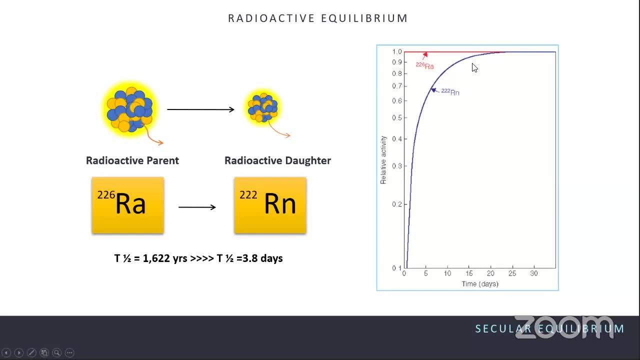 The ratio becomes to be constant, where you can see the both are merging in a, or it is known as asymptotic merging in a same line. So basically, it will take a huge time because the radon will be decaying in a higher rate. 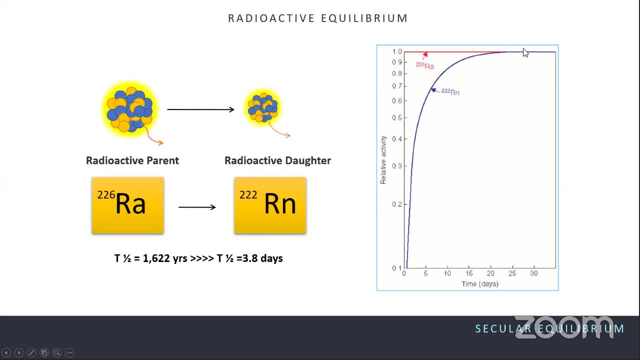 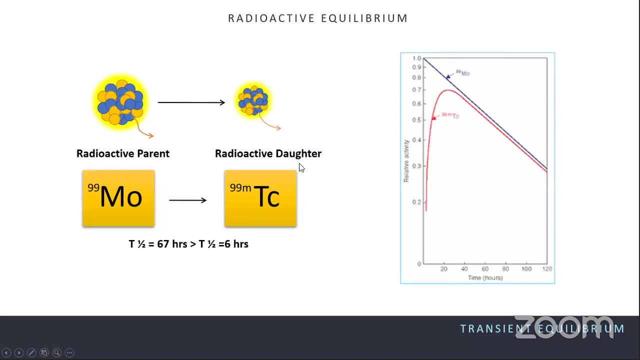 That is the equilibrium, But as the radon accumulates more, for the theory of activity, it will achieve the equilibrium, but, which is different for the transient equilibrium, where the difference between the half-lives are not much, So it will achieve the equilibrium quickly, within a few hours. 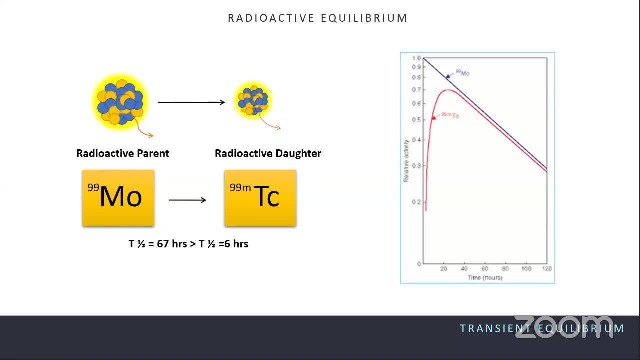 Yes. So the other question is: please explain beta decay and the particles, Beta decay, Beta decay. I have explained, Yes, Yes, Just your question: Is rate of disintegration for radium constant? Yes, Because the rate of disintegration is something you can see. it is the rate of decay of one. 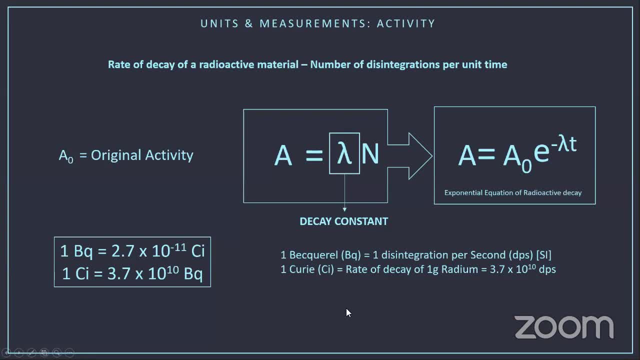 gram radium. If you want to see the unit that is curie, it is the rate of decay of one gram radium And this is basically activity. Activity is constant for any given material at a given time. So the other questions for radioactive equilibrium: 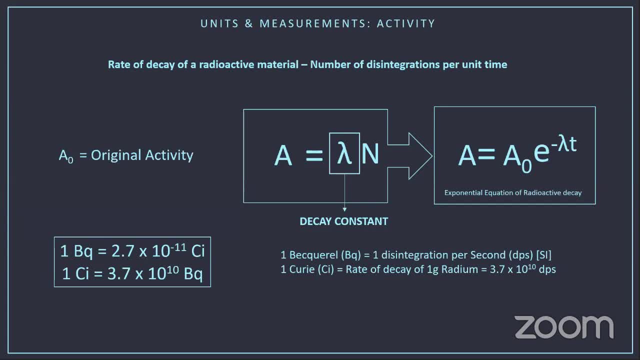 Two, three questions. I am just Wonderful presentation. What specific activity and how it related to disintegration, constant for the initial number of atoms And how these terms are different. Okay, Yeah, What specific activity and how it Decay, constant is something different. 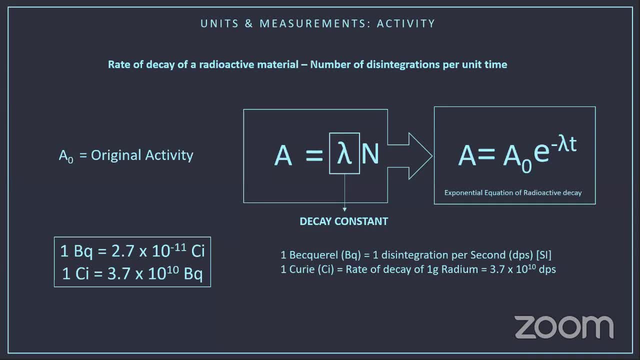 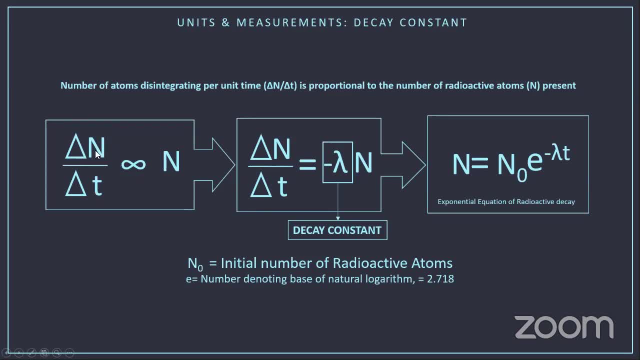 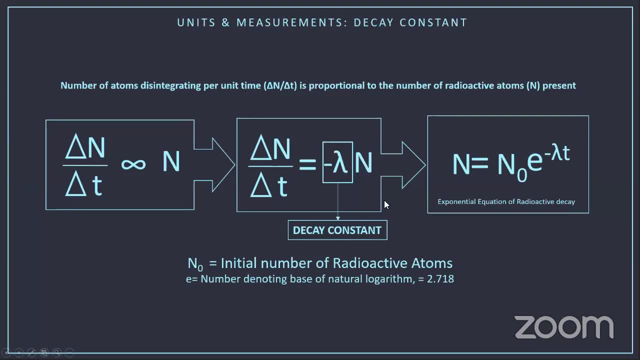 First of all, most of you know it. So if there's Tomorrow before you graduate, I can just- uh, I'll just tell you right now When you graduate, You as a professor, and a somewhere or once in the future. 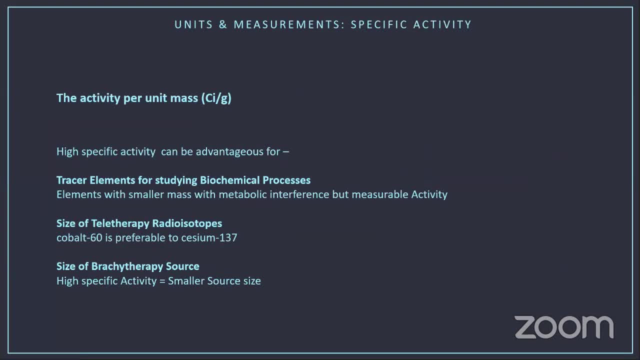 You have many practices And then, during the course of study, you have killed what happened, what had been affected by your materials, or what we have said. That was very, very important. So this is basically the amount of activity per mass. it is like at something like a density. 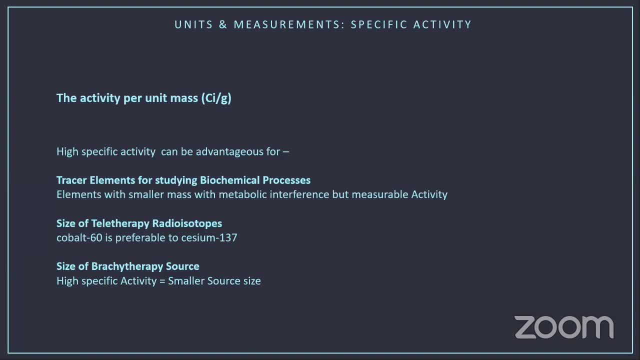 you know, the different types of element have different types of density, which is the amount of electron per unit mass or amount of material per unit mass. to similarly, the. it depends on the density. So the more atoms on within a unit mass, there will be more activity. 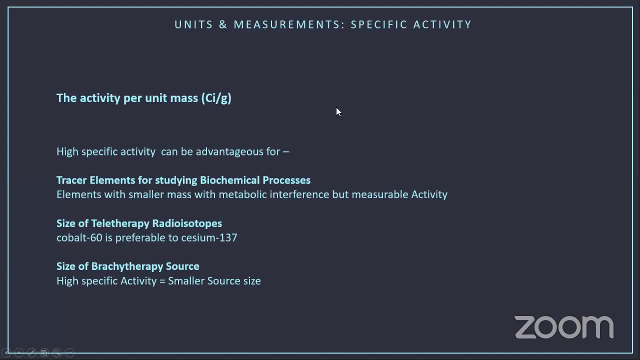 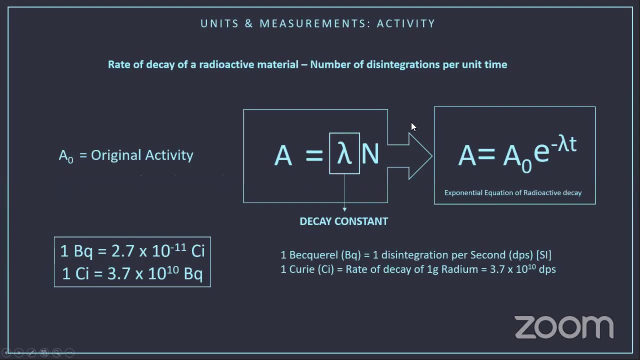 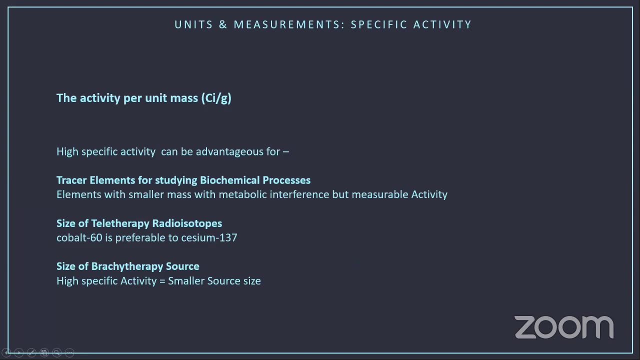 So basically, that can be explained, that that can explain their that they are different. These are two different properties of a radioactive element. So basically, the decay concept defines the what will be the half life, while the specific activity will define what will be the size of the isotope required to produce a similar. 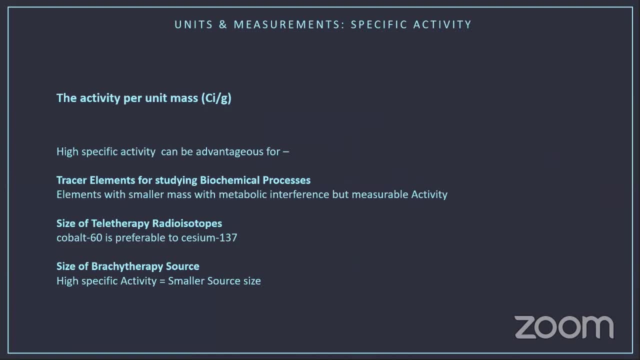 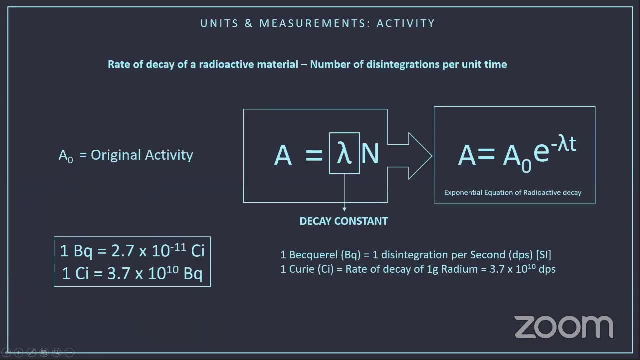 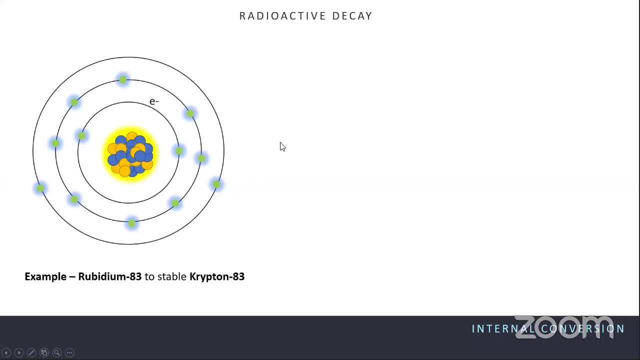 amount of activity. Then another question is: what is the Auger electron? and the other one is binding and potential energy. Okay, fine, You have already explained binding energy. I need to talk about Auger electron, Yes, Okay, Okay. so Auger electron is nothing specific for this internal conversion only. 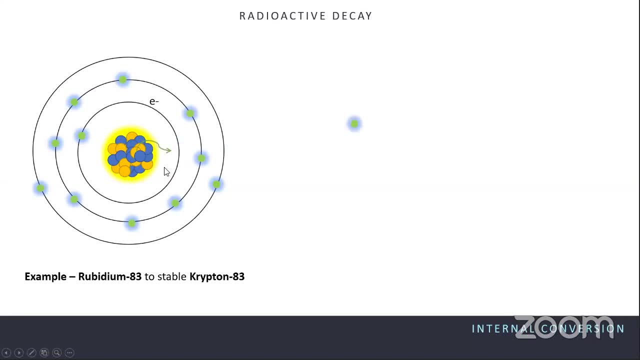 So whenever you see a particular valence, shell is empty, so some it cannot be kept empty. Okay, so some electron will jump from the outer orbit to fill the hole. So once the electron jumps to fill the hole, as per the law of atomic energy, it will release. 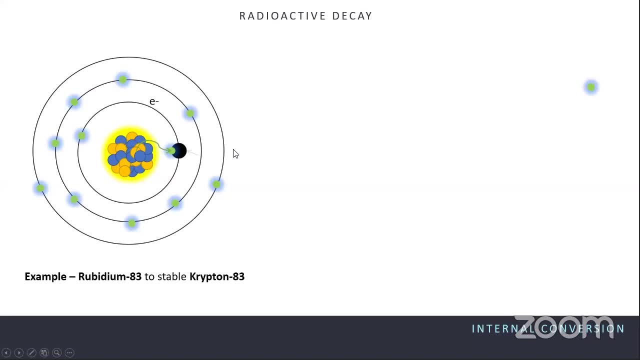 some energy And this energy, as we know the energy- will be released as a photon. So suppose there is an atom and the photon is coming from the inner shell. So photon has to traverse through the atom to come out of the atom. 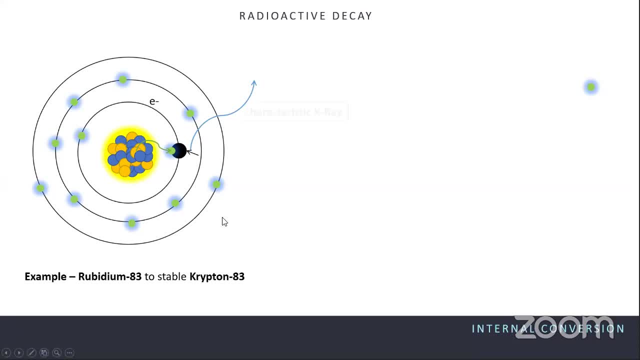 Now in the pathway of the photon, it interacts with another electron which is in some shell, And as soon as the electron absorbs the energy of the photon And if the energy of the now the new energy of the electron is more than the binding energy, 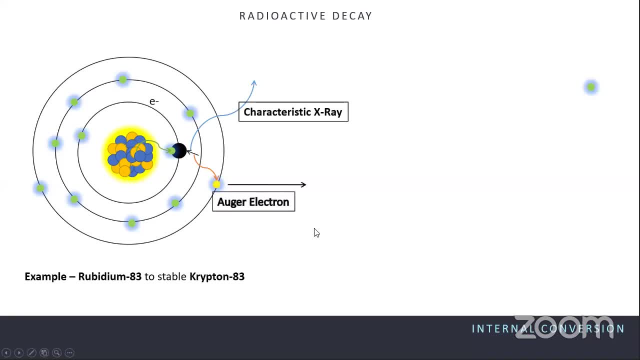 this electron will escape of the nucleus, So this is known as Auger electron, because it is produced by absorption of the characteristics or phosphorescence x-ray. Okay, so then, binding energy: you have explained MeB and MeB. I think this will be explained in later classes, right? 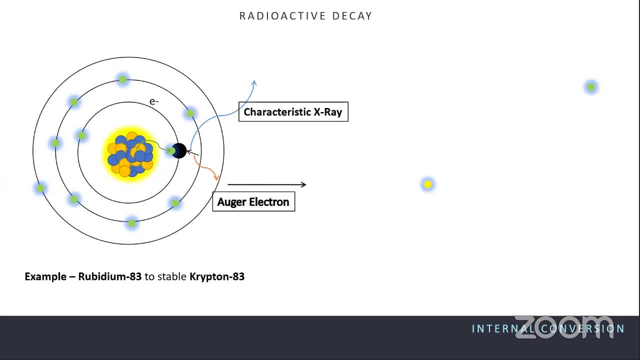 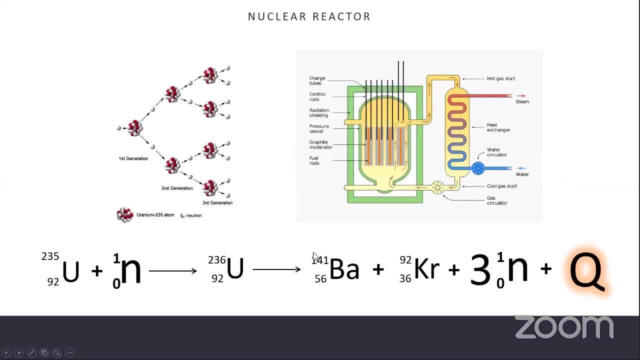 Mm-hmm And the fission Mm-hmm. And the fission comes from where? In fission, first neutron comes from where? That is the question. Okay, So when the first thing is that when this uranium is bombarded with a slow neutron, 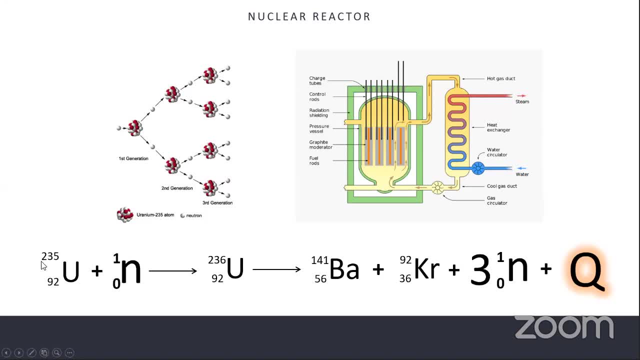 so which is done is with a slow neutron, the uranium is bombarded. Now this uranium element will spontaneously break into this elements, or it will change into barium, it will change into krypton And it will give rise to neutrons. Now, this entire process will generate an enormous amount of energy. 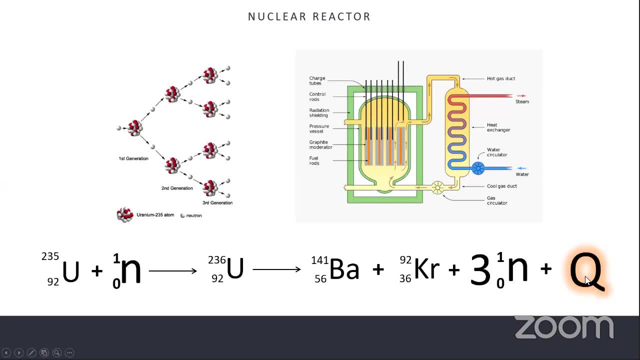 And out of all this product the energy will be distributed equally so that there are no energies lost. So, apart from the energy which is radiated as heat, the other energy will be absorbed into this particular elements and they will be acting as the kinetic energy of the elements. 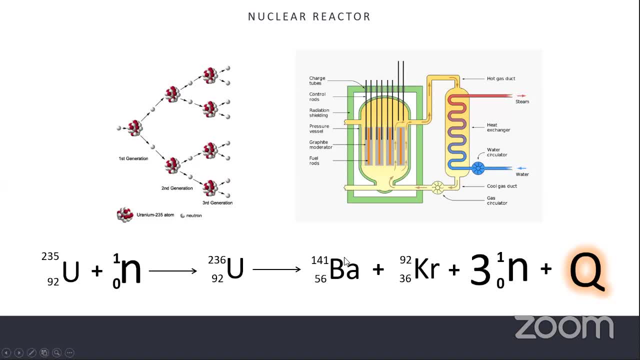 Now, if you compare these elements, you will see the amount of energy. Okay, Okay, Okay. These are all heavy particles compared to neutrons, heavy nucleuses in compared to neutrons, And even the energy will be going. these will have the recoil kinetic energy because of 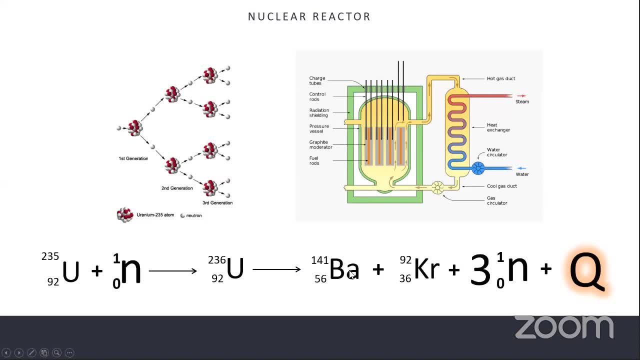 the high atomic weight they will not move much, But because of the light weight of the neutron they will absorb the energy and will have enormous kinetic energy. So these neutrons will be fast neutron. Now you need to understand this, Okay. 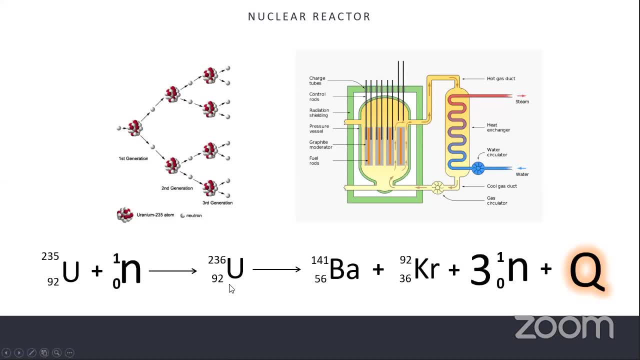 Now you need to make them again slow to further initiate the chain reaction, because the slow neutrons are capable of generally causing the fission reaction. Okay, So could you please explain that if an electron moves from outer shell to inner shell, then how the energy is emitted? is it related to winding energy? 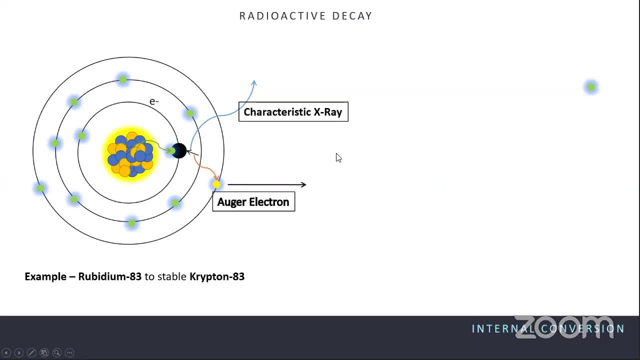 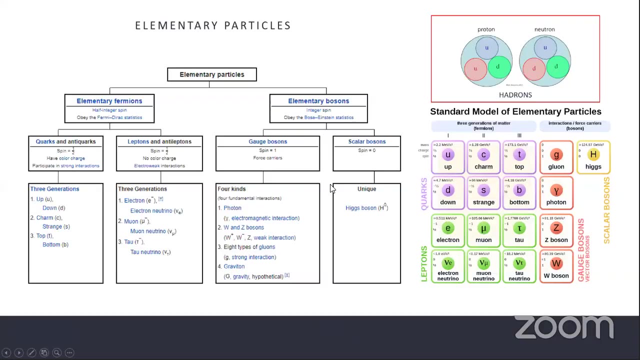 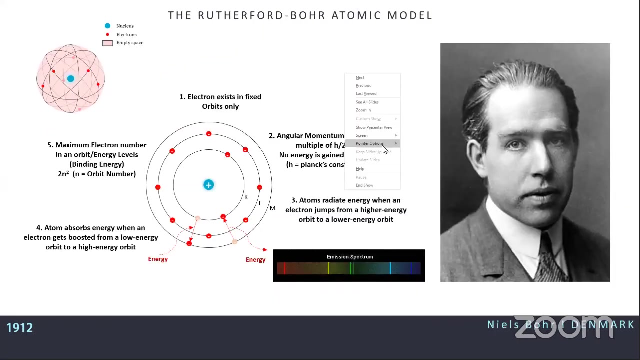 Yes, So Can you give me one minute, Just a minute, Okay, Okay, Okay, If you go to the Bohr model, you see, Okay, Okay, So You can see that you can see the energy of your system of-or by orbit is fixed. 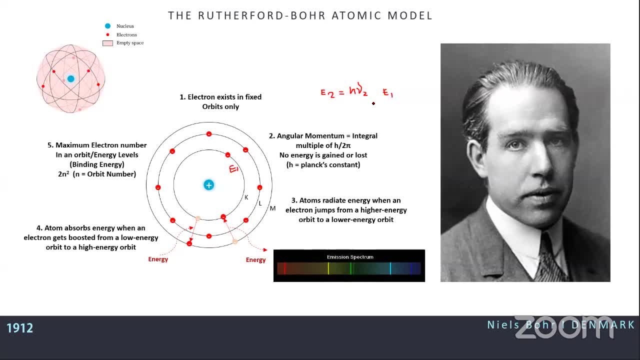 Right. So we can write this energy as suppose E2, equal to H, is a constant and the frequency Right Now for this particular, the lower one, also, there is some energy. So the energy will be the E2 minus P1, which can be described with the cos theta. 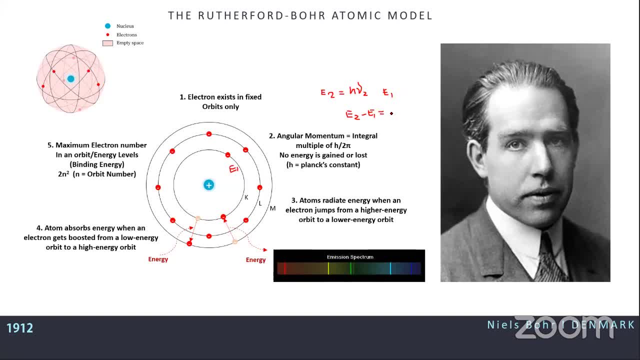 So let us just see if it is true. Yes, Described by the h nu 2 minus h nu 1.. And if you want to see what is the nu nu is basically c. by lambda That means c is the speed of light and lambda is the wavelength. 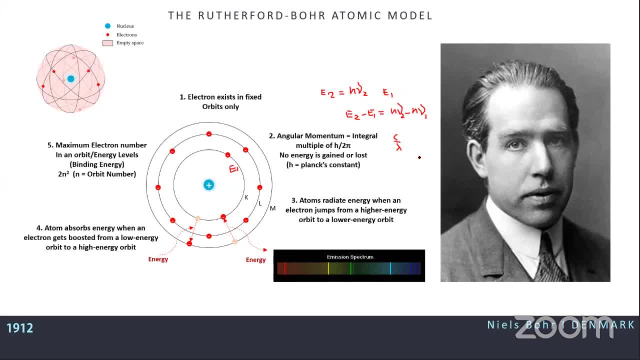 So it depends on the wavelength of the energy. Okay, so other questions are: explain biological half-light, That is. I think that is not related to this topic. Do you want to explain that? I don't think so. Yeah, and difference between activity-specific activity already explained. 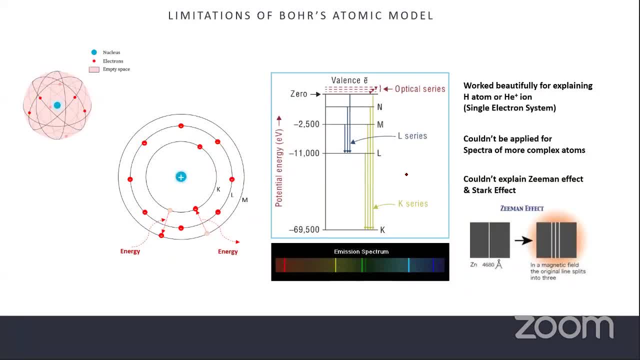 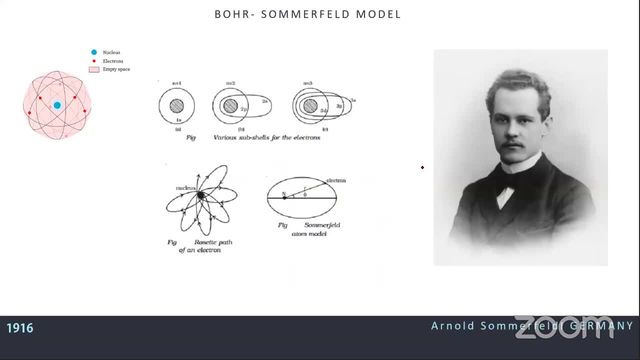 And characteristic X-ray. Dr Baivar, this will be taken in next class. We will cover everything. So is the average life is related to time to retire the source, like global 60?? No, usually it is calculated with half-light. 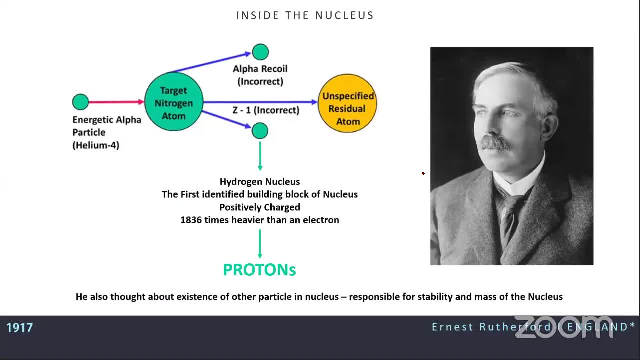 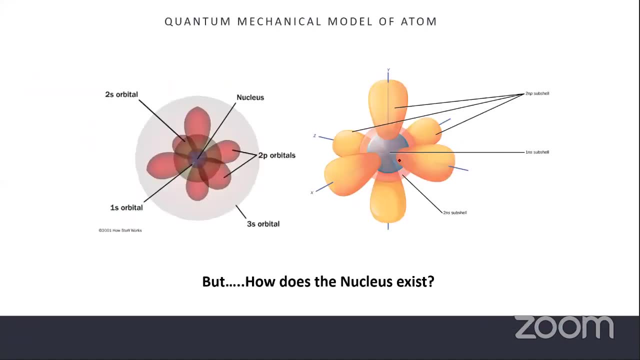 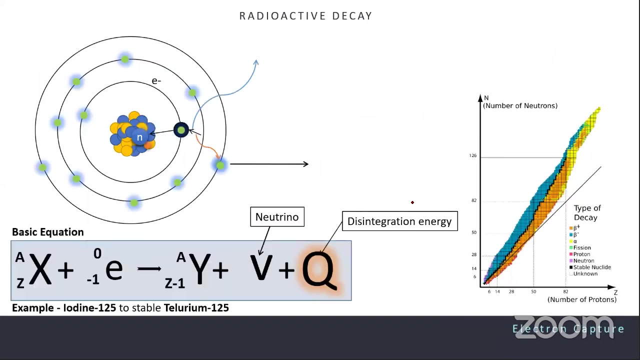 Yeah. clinical implication of it: Okay. And radiation oncology? I don't think there is any. for radiation oncology There is some application of clinical equilibrium, But in usually the secular equilibrium is important, for as it is in the nature And the transition equilibrium is important for this generation of the technician sources. 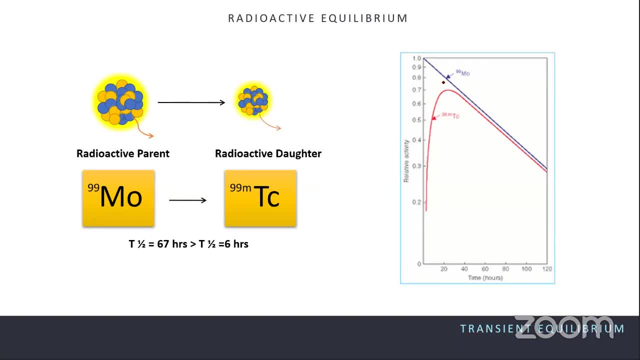 Because you can as the technician, as the rate Of decay is achieved quite fast And from the system it can be constantly taken out so that the production is very expensive. So because of this equilibrium, it is, the availability of technician in a metastable state is easier. 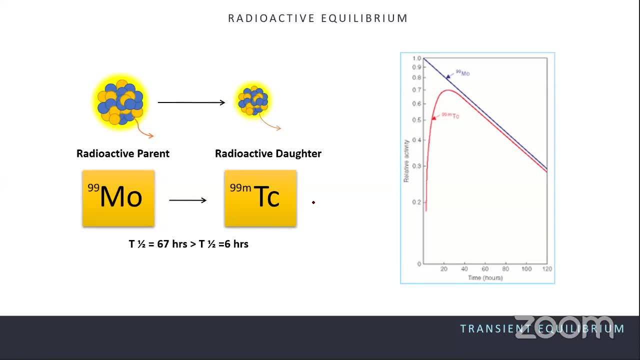 So you can quickly collect the metastable technician and can be inserted into the body for intervention. Okay, Dr S Chaitanya has asked: please explain a little about periodic table. I don't think we need to explain periodic table. We are essentially radiation oncologist and medical physicist. 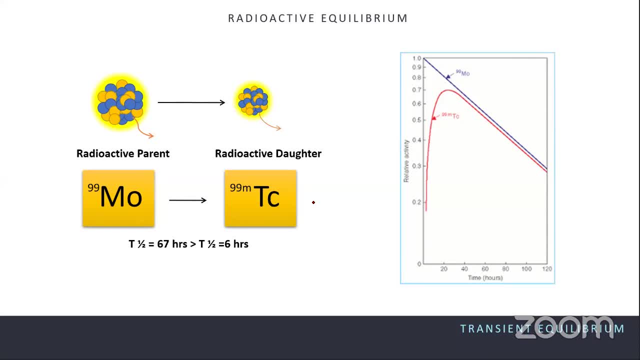 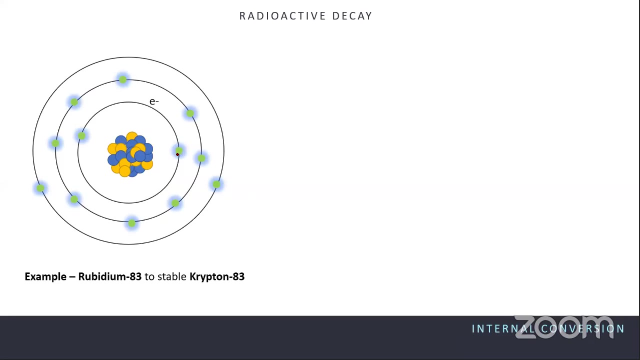 So that is another domain. Please explain about excited electron. Does it remain in their original orbit or it leaves the orbit? Okay, So if there are multiple way for the electron, So if one electron is excited, depending on the energy it is absorbing, so it can go to the outer orbit? 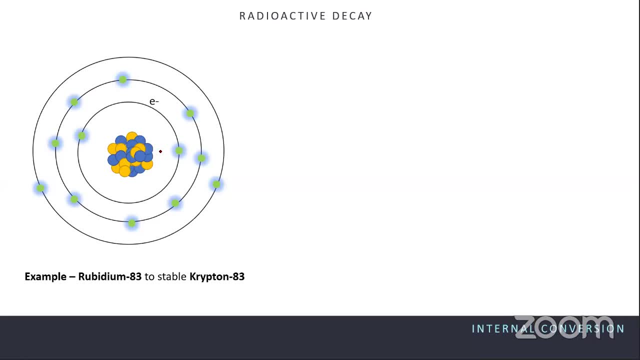 It has got so much of energy that it can be, It can go out. Okay, So if there is so much of the system that is more than the binding energy, it can go out of the system also. So we can have more about this excitement and reaction of electron to energy in the, I think, when we will read about interaction of photon with matter. 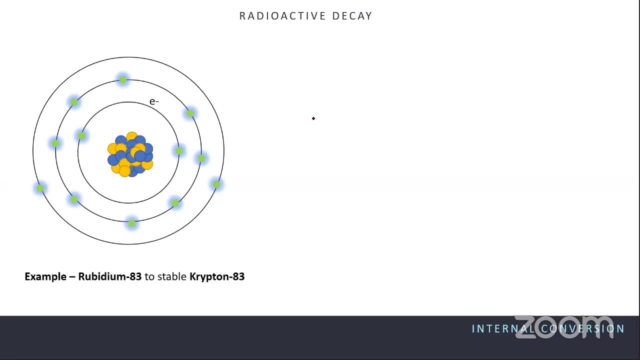 Yes, yes, We have in next classes will be explained, And cobalt decay and electron capture you have explained. I don't think you need to repeat it again. So another thing is yes, So any more questions? No, cobalt decay and electron capture. 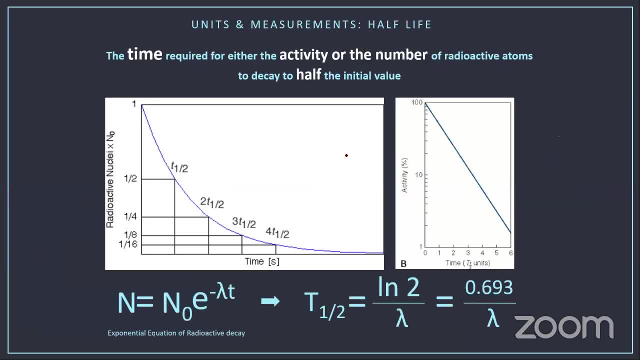 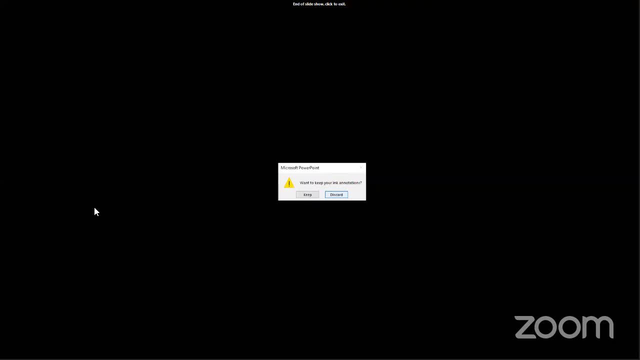 I think you have already explained, right? Yes, electron capture. I have explained. I can explain the cobalt decay once more. Yes, And then, if Dr Sayan does, if there is any question from YouTube, you can put it here. 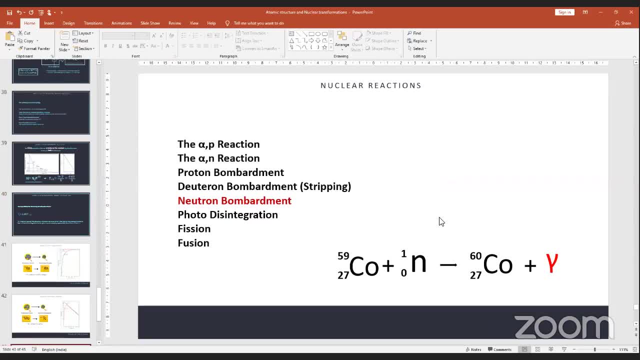 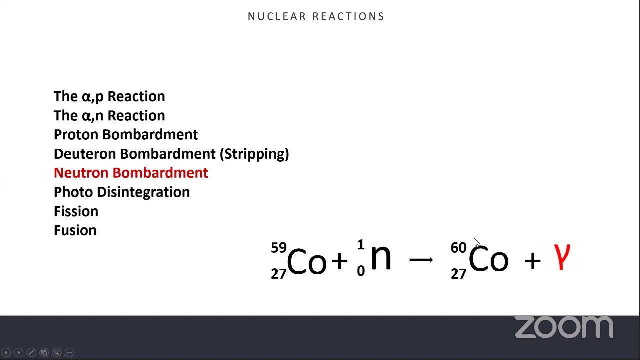 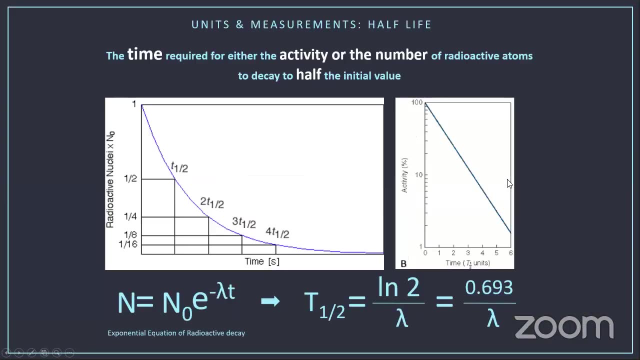 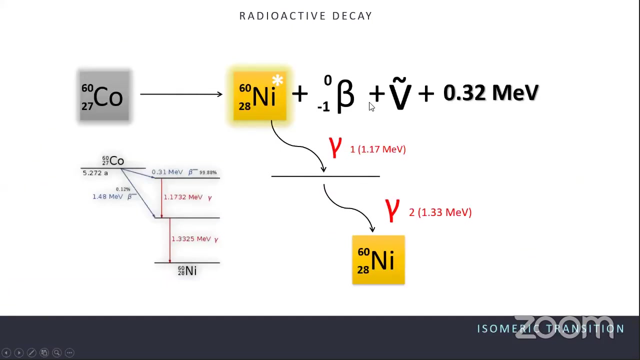 So how the cobalt is formed: One neutron go by Neutron, go by Neutron bombardment, We find the. we make the cobalt radioactive, which is an artificial isotope, And this cobalt decay by beta decay, And I'm not going to explain beta decay again, but the cobalt decays by beta decay, right. 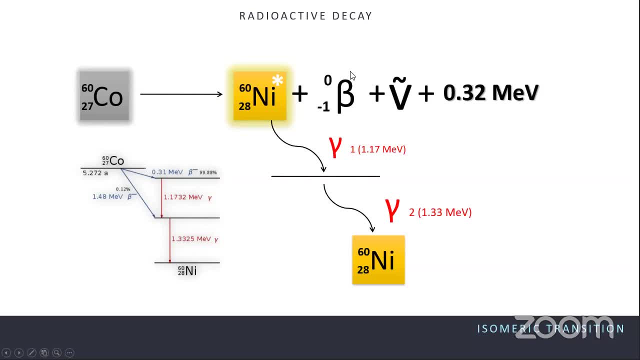 So it will emit one beta negatron. Now, as you see, there is one emission of the negatron. That means there will be increase in the proton number. Right, Because the positive, the negative charge is explained. So the positive charge will increase. 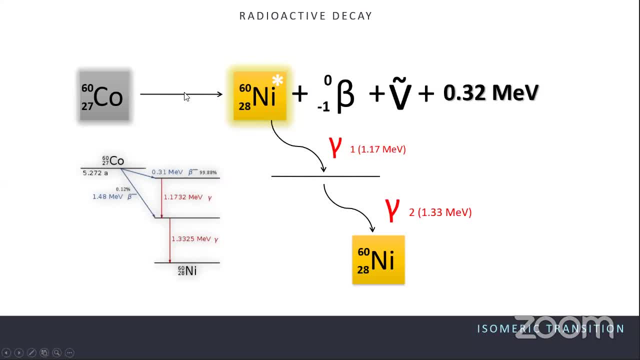 So as the proton number changes, the element will change to nickel. Now this product from the cobalt-60, the nickel-60 will remain metastable or unstable for some time because of the reaction, And this will emit the energy in two steps by two gamma rays of 1.17 and 1.33 MeV and will become stable. 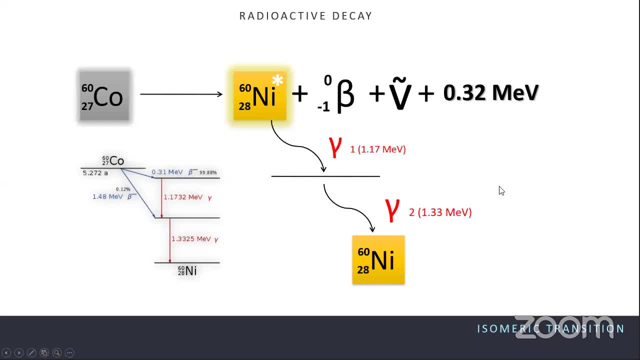 So this is the gamma ray which we use, Which we use for the treatment purpose, And if you know the cobalt source we have, it also decays by beta And this beta is actually captured within the shielding material. Dr Sayan, is there any other questions from YouTube? 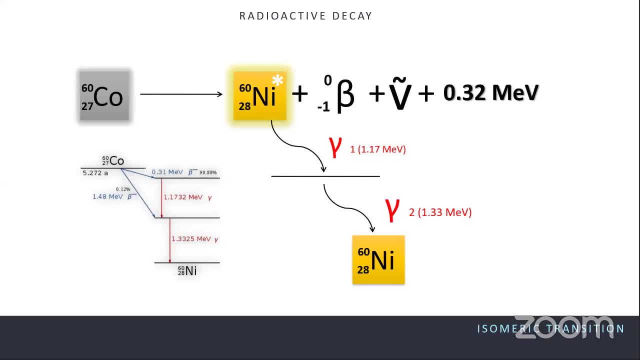 No relevant questions, And some of them have already been answered in the comment section. Okay Then, thank you, Dr Jeevak, And thank you all the participants. It was an excellent class And we had almost 800 people attending this class. 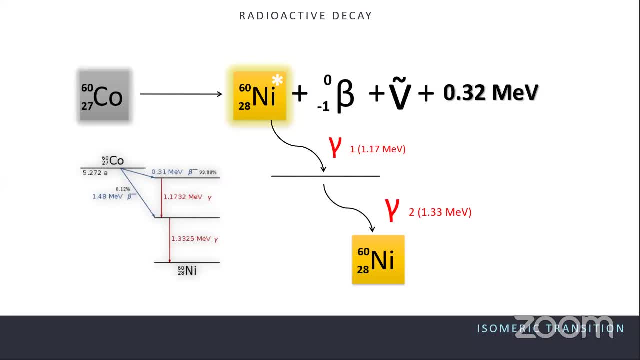 I think one of the biggest medical-physicist class ever happened in the world. Thank you, Yes, So maybe we have created some record. So thank you all. The next class will be by Dr Hrithika Hinduja on the Thursday. 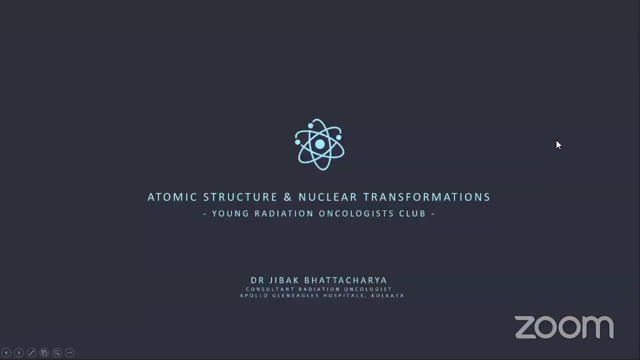 That is, on 3rd of September, On production of X-ray and clinical radiation generator. So we expect everybody will again join on Thursday for the next class. Thank you, Thank you all. Thank you. Now, I am just closing this session.